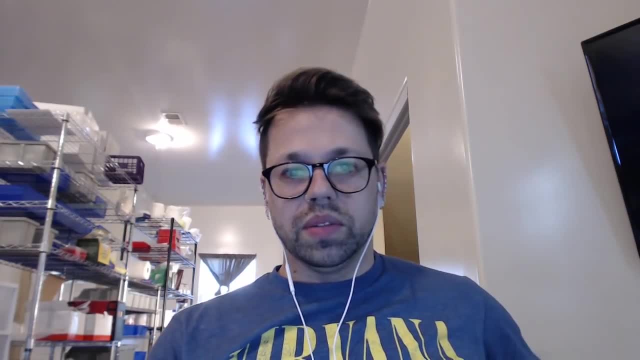 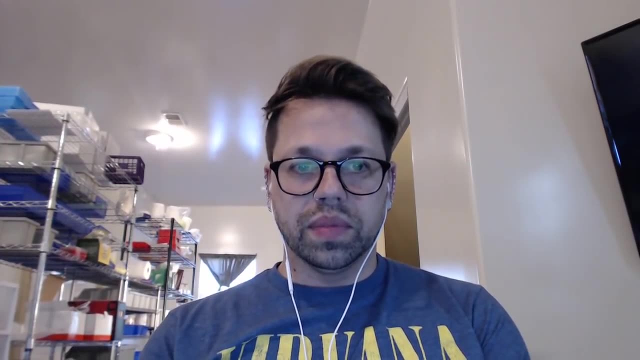 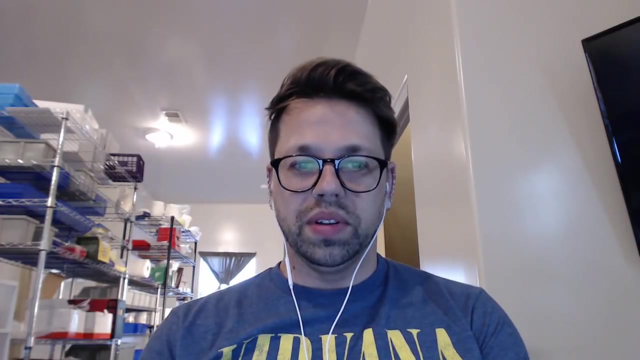 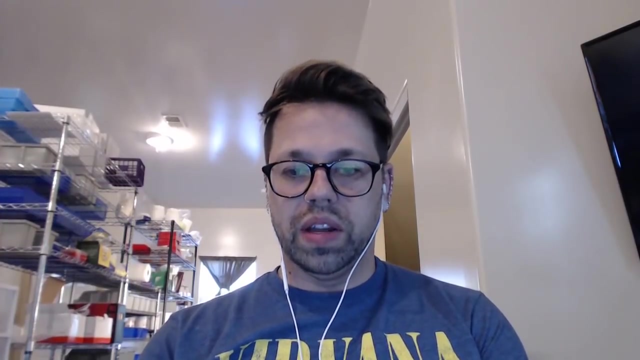 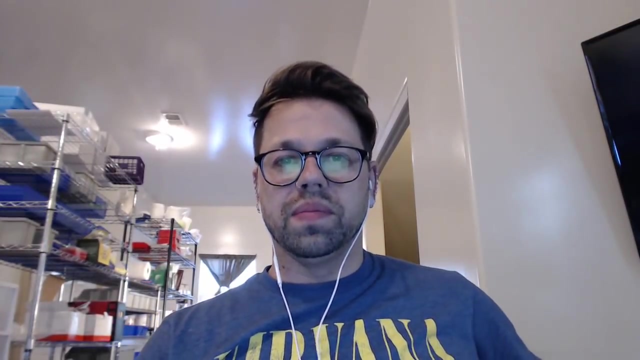 All right. So what should I add? You have it E-S-T-E-A-S-T-E-R-D-A-Y. Is that how you spell it? No, E-A-S-T-E-R-D-A-Y. All right, All right. So if you want to open up the syllabus, feel free to open it up. Otherwise, I'll just go along with it. 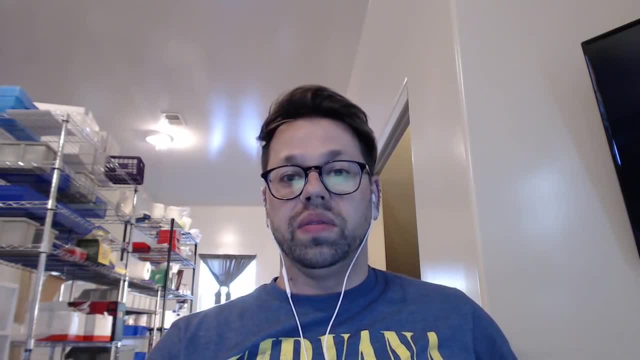 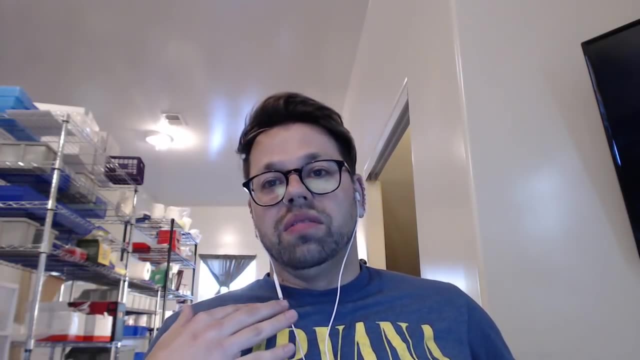 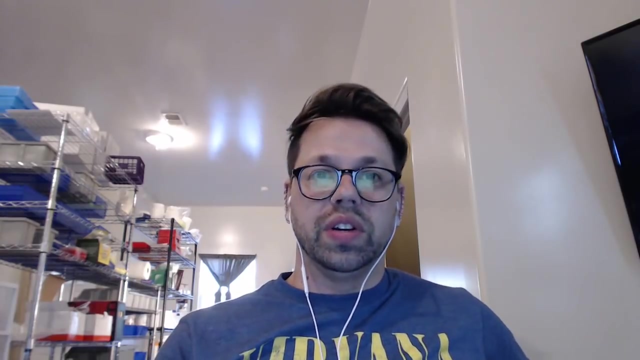 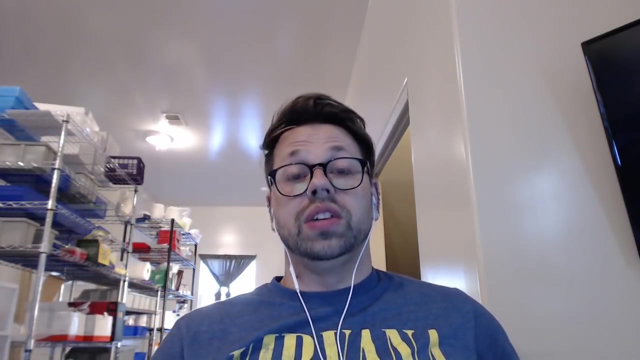 So this class is going to be a combination of theoretical knowledge and experimental knowledge, because we're assuming that you all have no knowledge in this. And even if you do have some knowledge in molecular biology, genetic engineering and those things, I suggest you still you know, follow along so that you're able to brush up on the knowledge and skills. 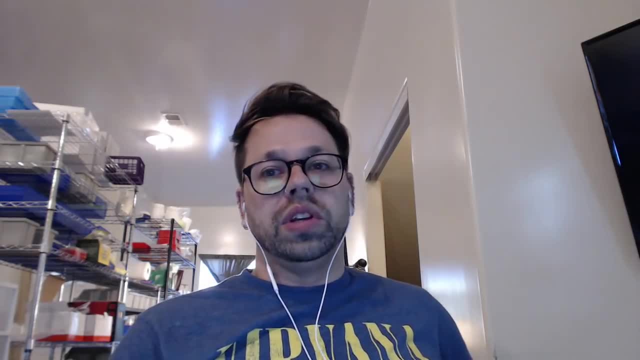 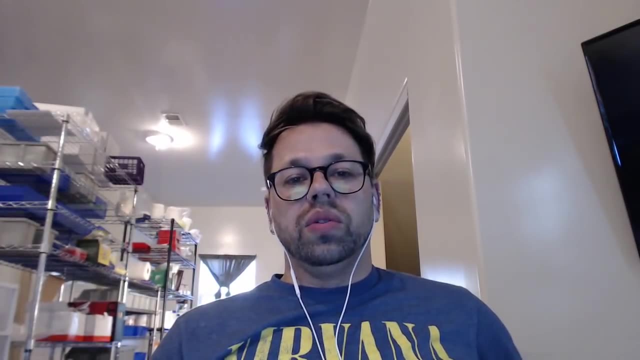 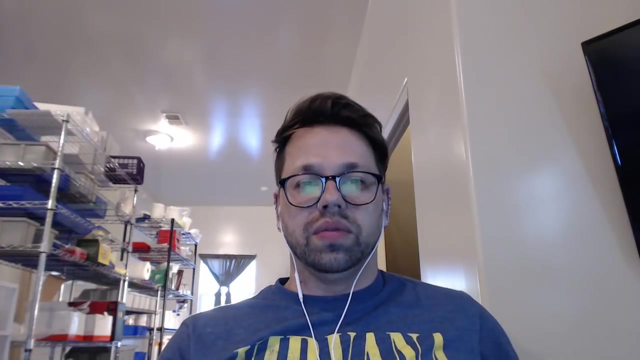 A lot of times we think we know stuff and we don't actually know it as well as we thought we did. So you know, pretend like you don't know anything and start from scratch while you're doing this class and hopefully you can pick up a lot of different things. 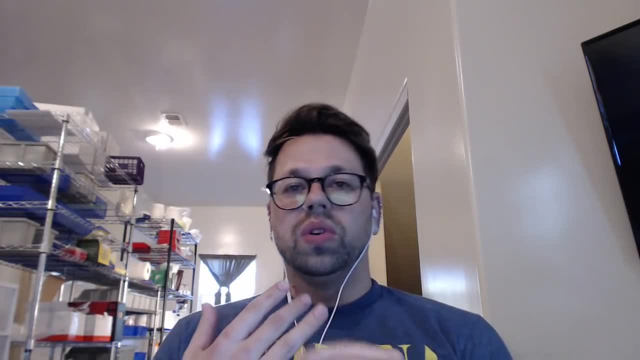 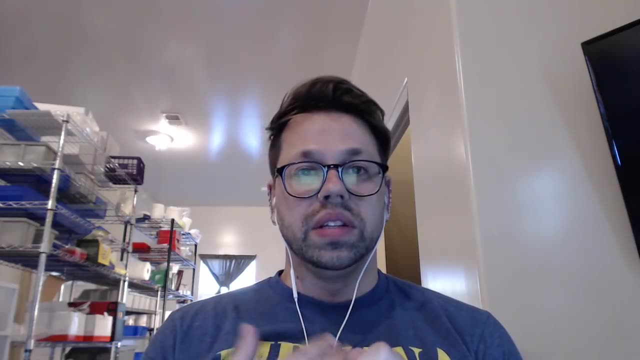 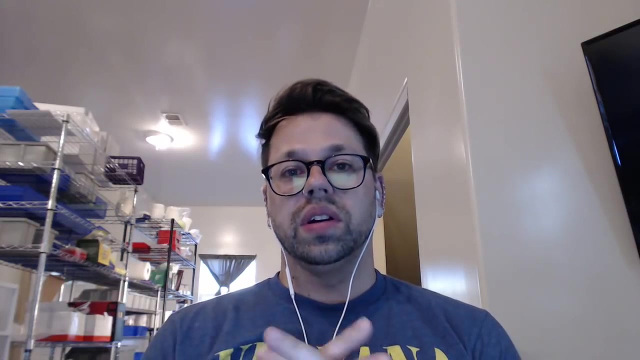 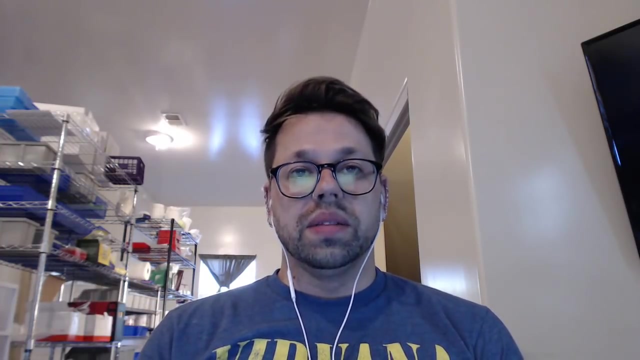 So the goal of this class? there's four different things We're going to try to learn about. We're going to try to learn about cells and DNA and RNA, protein and genetic engineering. Those four things are the main concepts we're going to look at, because those concepts are pretty much the concepts you need to know if you want to do genetic engineering, molecular biology, in the world today. 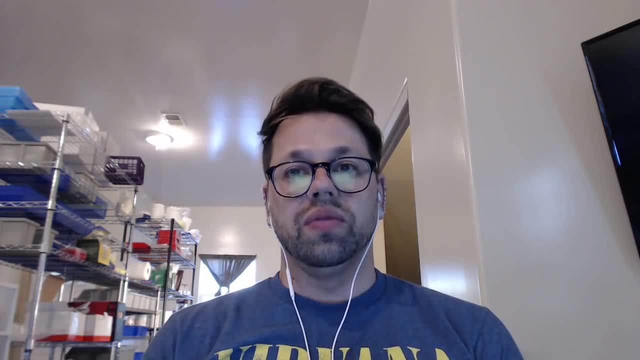 And some of them. you can have a little bit less Less knowledge For this class. obviously it's two months. It's going to be fast, There's going to be a lot thrown at you. What I suggest is just try to consume as much as you can. 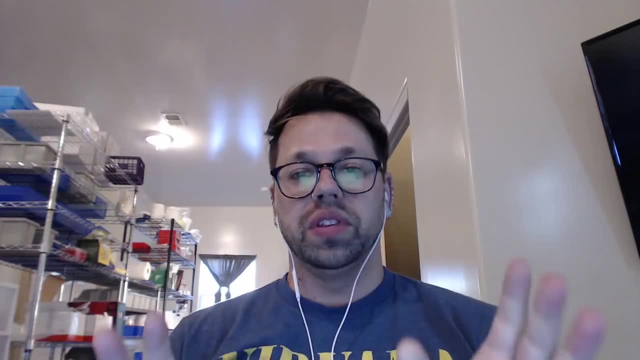 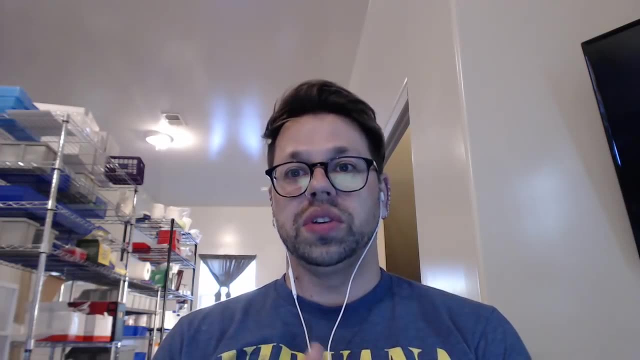 Don't feel like you have to consume everything. Read every paper, Read every chapter and every page of the book And do every experiment. Just try to do as much as you can, Because these things obviously take time to learn And you can't just learn it. 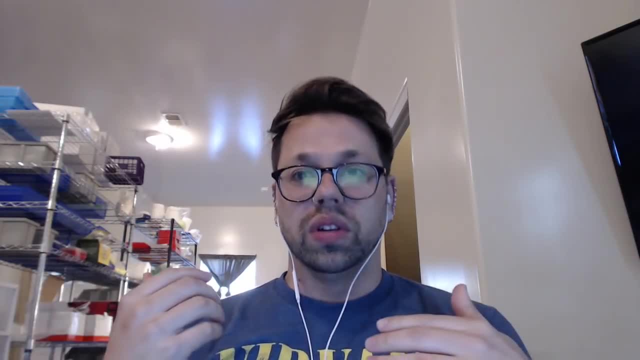 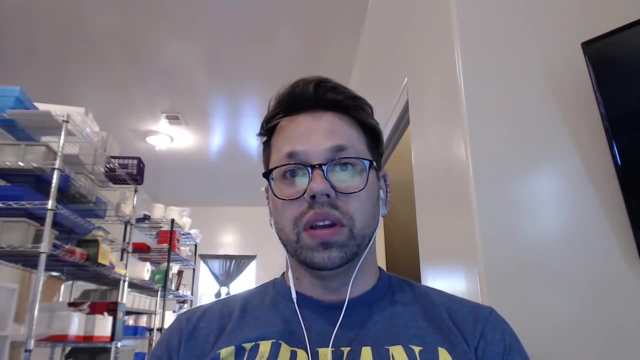 In two months or whatever. Two months will give you a great foundation that you can then go on to explore lots of things. But if you want to actually be really good at this, it's going to take a little bit more time, And that's okay. 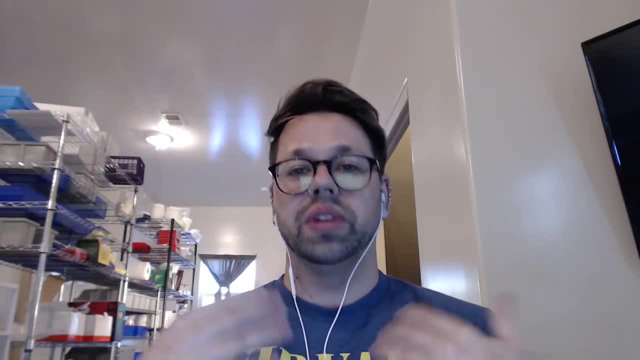 It's just constantly subjecting yourself to the information, Constantly putting it in front of you, Constantly being involved with it, Constantly talking with people. I recommend that You know, You go on social media: Facebook, Twitter, Whatever. 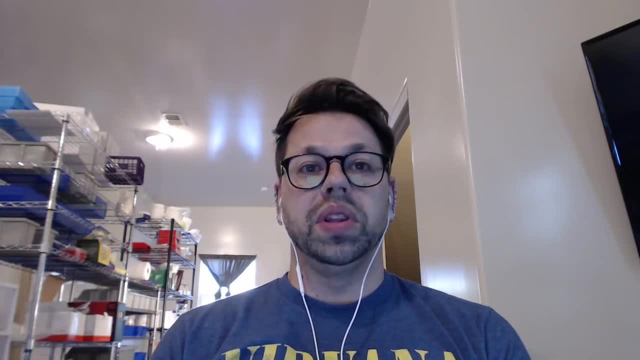 Find us And interact with the people that we interact with. You know, Get involved in a community. If you have a local biohacker space, Get involved in the community And just constantly be around this stuff So that you can grow as a scientist. 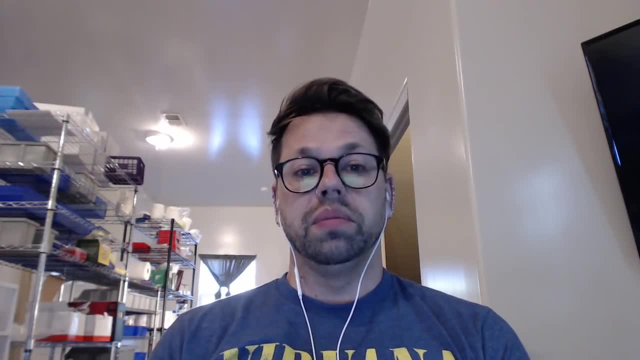 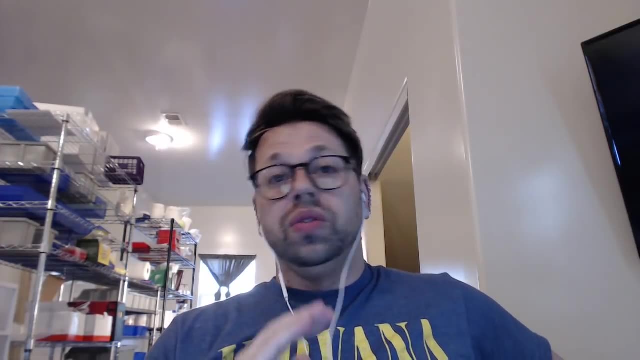 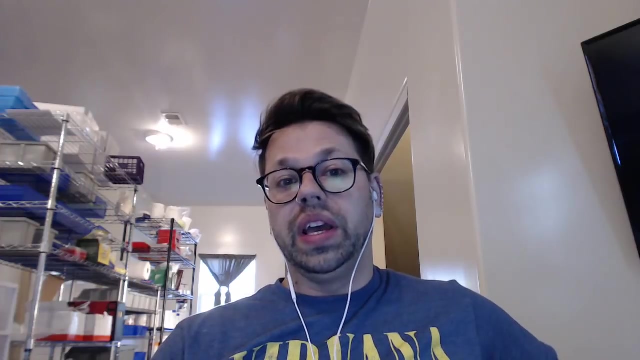 Because that's the goal Is to have everybody be scientists. So, like I said, The goal is to take you from Absolutely no knowledge- We're just pretending that you have no knowledge, Whether you do or not, And go all the way to doing CRISPR experiments. 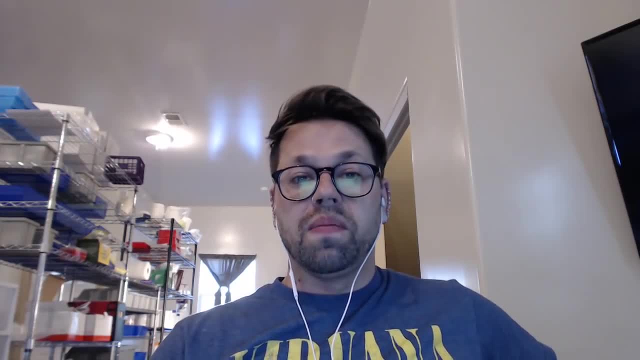 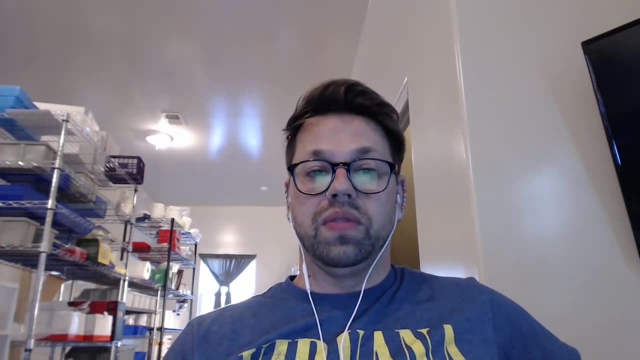 And genetic engineering experiments. Now The book we're going to use is Molecular Biology of the Cell And you can download a free copy. You can find that on Google Drive. It should be on the classroom And everything like that. Download the book. 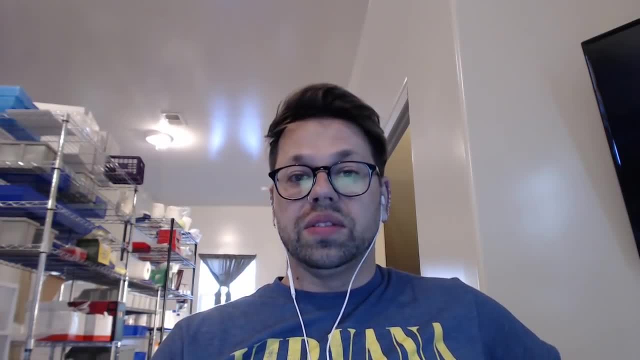 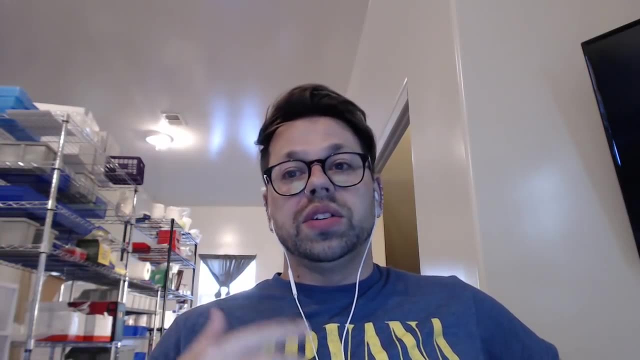 Now. Now It's a lot to read, Right? So Be prepared, It's going to be a lot, But, like I said, Just try to read as much as you can, Even if you only read, You know, A few pages every week. 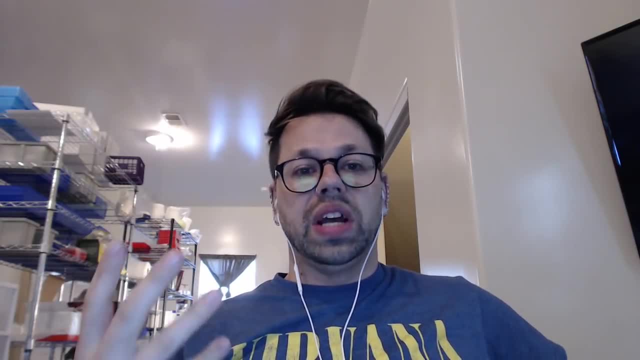 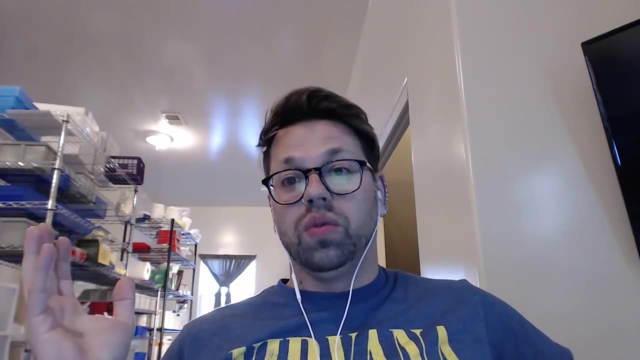 Just read something So you have some basal knowledge That you can then apply in the future. It's just constantly doing that: Reading just a few pages, A few pages, And eventually, over time, that builds up And it turns into hundreds and thousands. 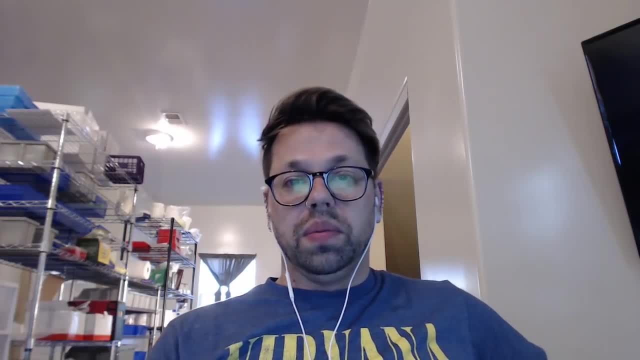 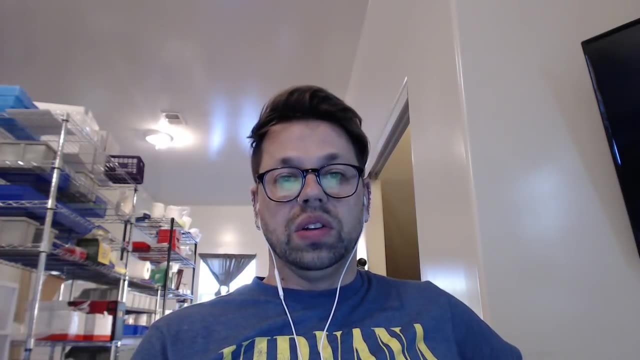 Of pages. Right, We're going to use a couple pieces of software A little bit later in the course, So you don't necessarily have to download them. Use them now, But they are Snap Gene and VMD. So 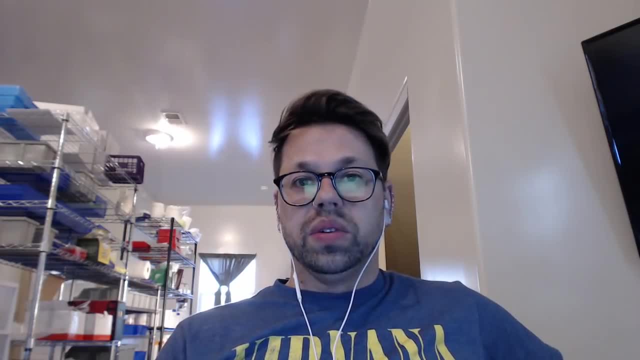 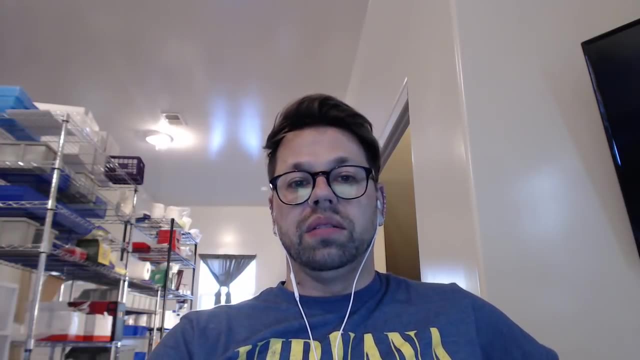 When you get a chance, Download those. I don't know exactly what week we will start using them in, But it's probably not for a few weeks, So don't worry too much about that right now. So If you are missing anything, 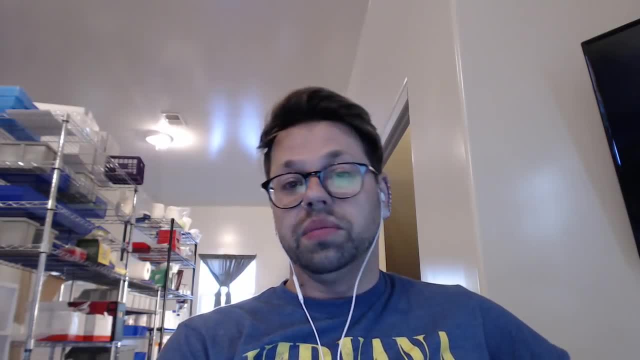 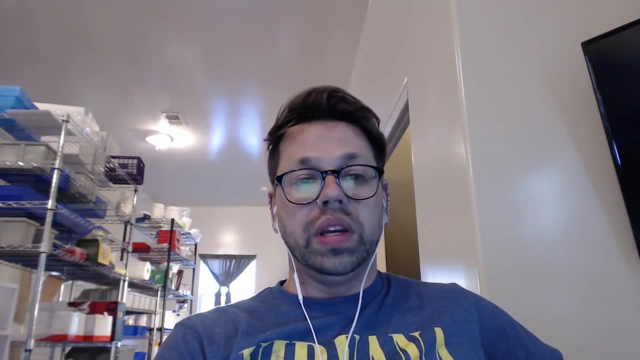 Or you end up missing something Or losing something Or breaking something During the course of the class. Just contact us And we'll help figure out how to get it to you. We'll make it right, We'll fix it up for you. 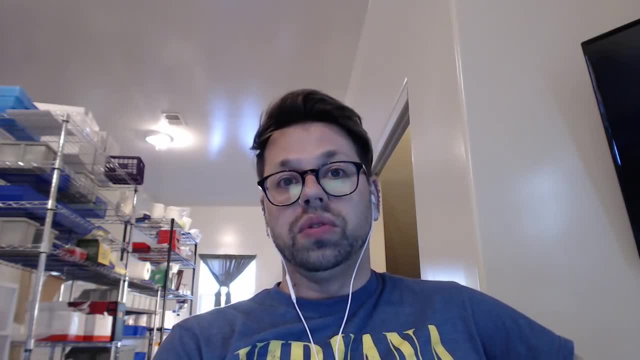 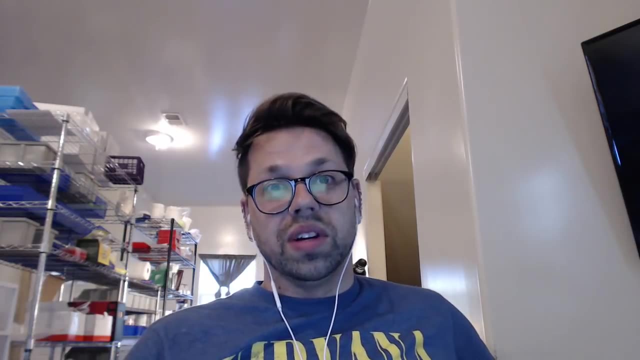 So that you can continue with the class. Our goal is to help you to be able to learn these things And do these experiments, Because once you become a good scientist, You're going to buy all your stuff from us, Right? I hope so. 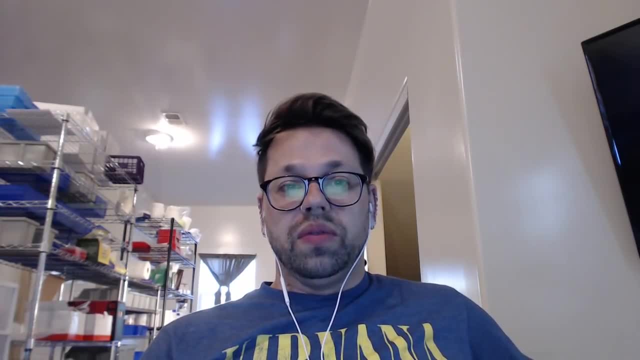 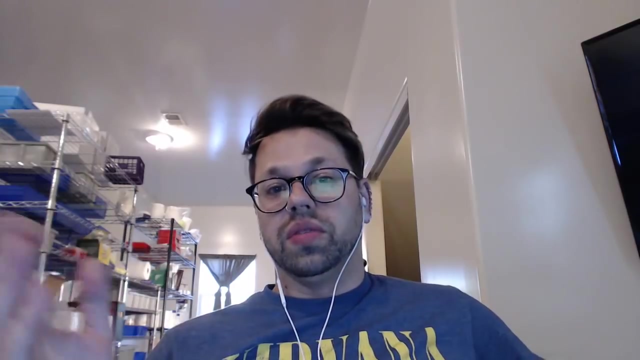 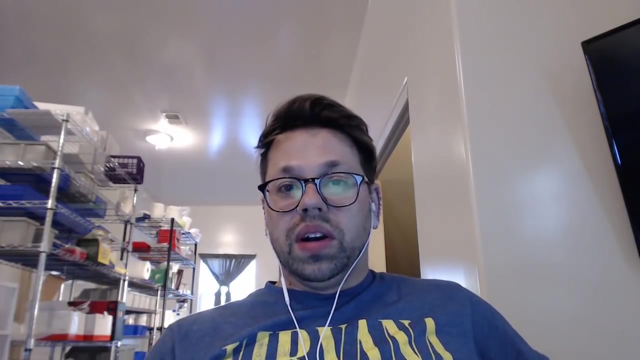 So if you scroll down to the bottom of the syllabus, It gives you a list of the chapters In molecular biology of the cell That you should read During different time periods of the class. Again, You know, I know it's going to be hard to read these things. 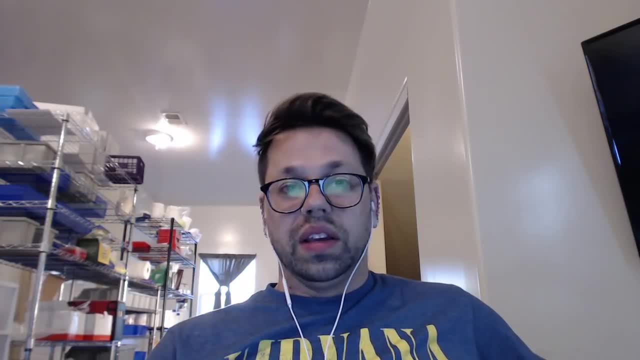 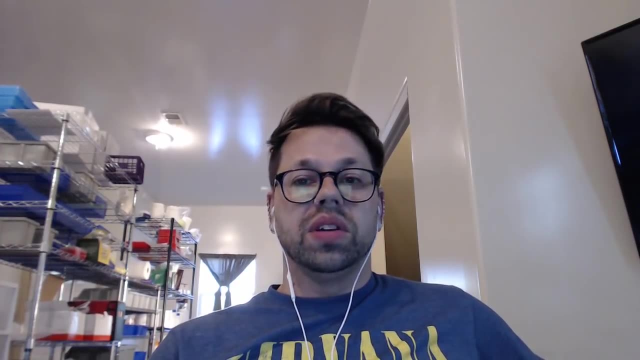 And put in the hours to get it done. If you can Like, that's awesome. If you can't, Don't be pissed off at yourself And don't be mad at yourself Or anything like that. You know, Just do your best. 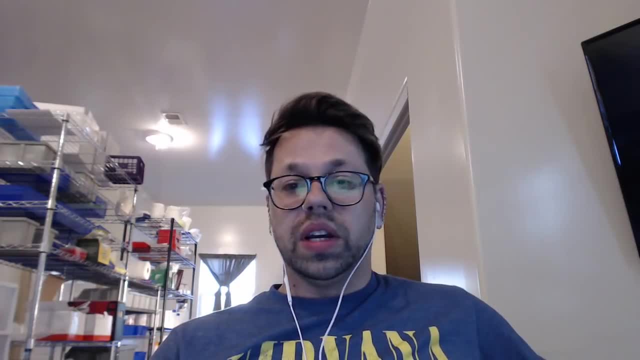 That's what this is about, Right? You're not going to become a genetic engineer Or bioengineer in one day. It's going to take a little bit of time, So just do your best with everything you can. Now part of the course. 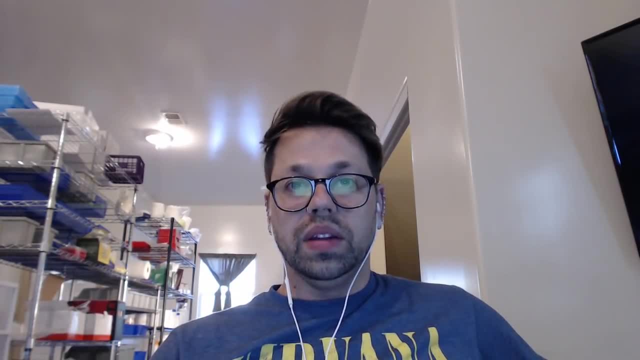 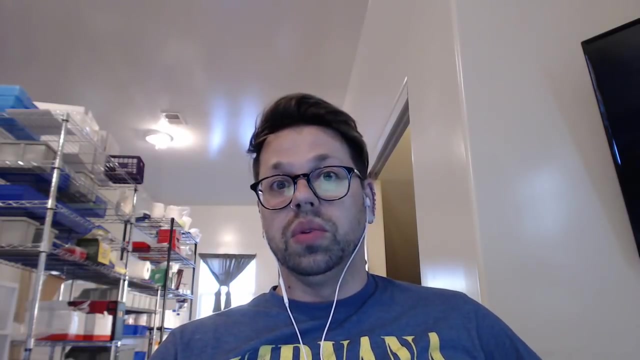 That is Interesting. that we're trying to do is We're trying to get you to read scientific papers. Experience reading scientific papers Is really important, Because if you plan on sticking with this stuff And doing it more, You're going to have to read scientific papers. 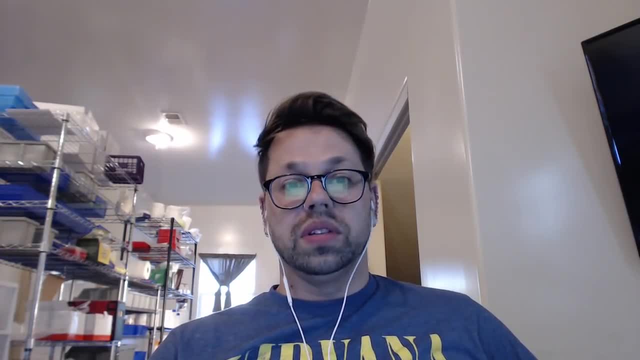 Doesn't matter if you like it or not, And you know I'll be honest with you, Scientific papers are boring as shit And they're hard to read, Like even for me. Sometimes I have to read a scientific Paper ten times. 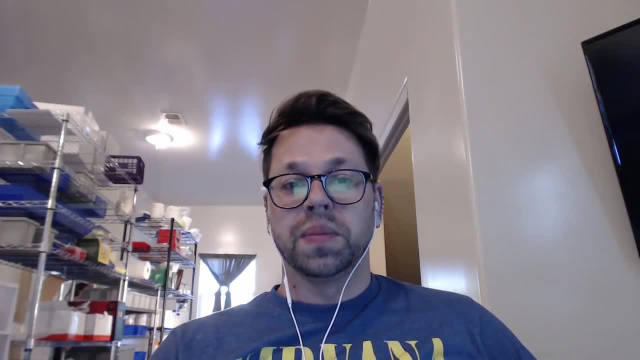 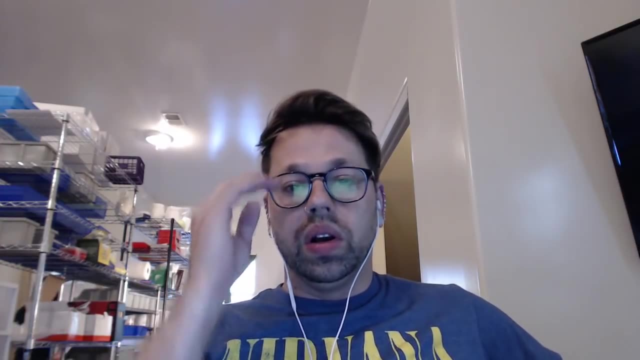 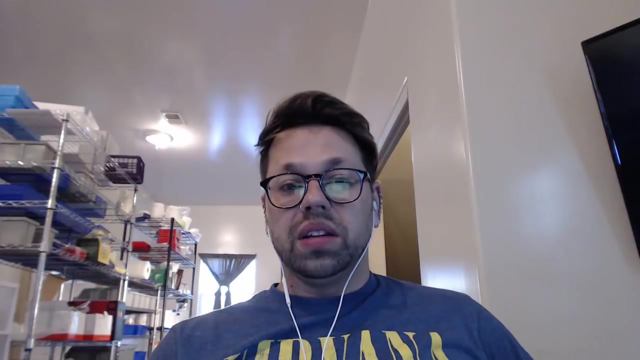 That's you know. In my field I got my PhD in, So don't feel bad if You read a scientific paper And don't understand it that much Or can't figure out what it is. What I suggest is You read scientific papers. 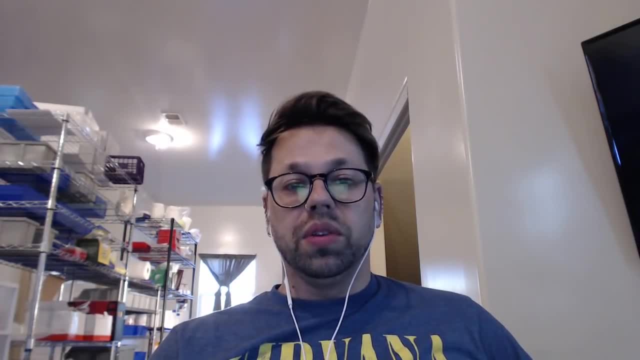 And as you go through- Go through slowly And just like look up some of the words And things that you might not know Or understand right You're talking. when you're learning Genetic Engineering and biology, You're learning a whole new language. 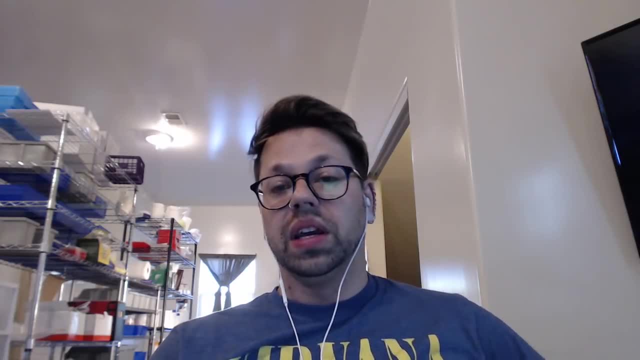 You're learning all these different words And things that mean something And you need to figure out what they all mean. So just go through And look up all the definitions of words That you don't know- Like that is a huge start. 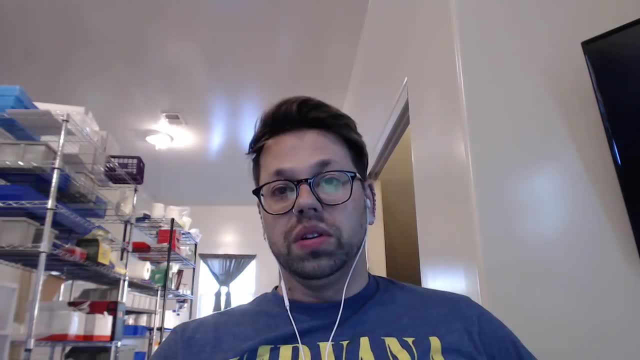 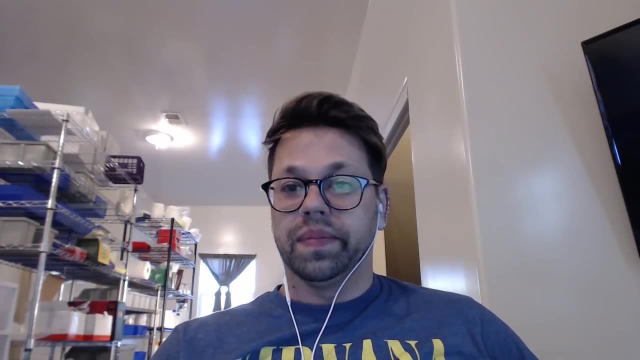 That'll get you so far, And you could also impress your friends When you talk about the difference between Pluripotent and totipotent stem cells Or something like that. right, Impress your friends When you're going out for a beer. 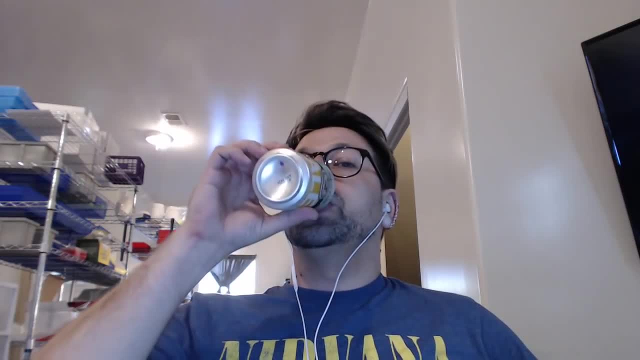 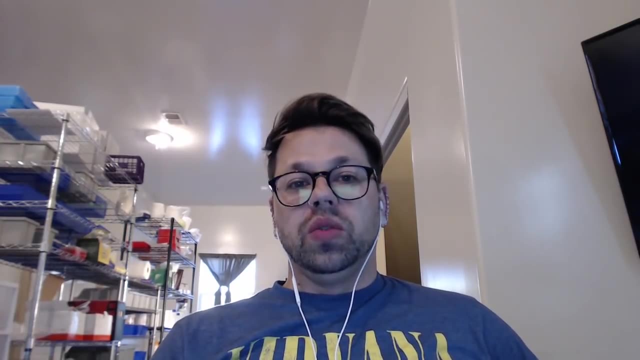 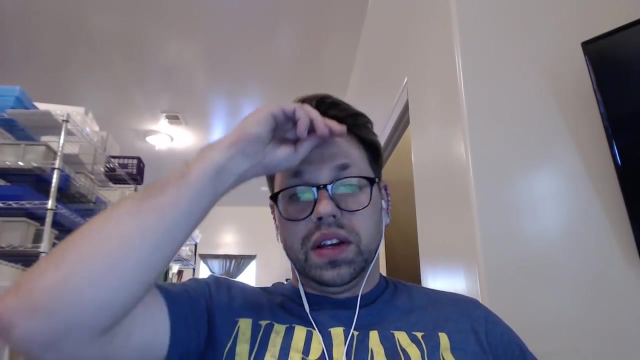 That's what I do, Alright? Yeah, so We divide the experiments up into weeks, But don't feel like you can't skip a week And remake up the experiments. Some of the experiments for some weeks Might be pretty short And just take you like. 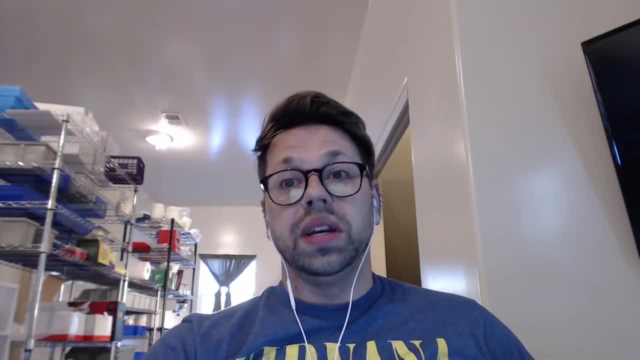 An hour or two or something like that, And others might take much longer. So You know, Don't be afraid to start some experiments And stop them. Usually there's a lot of stopping points In experiments, So that you don't have to do it all at once. 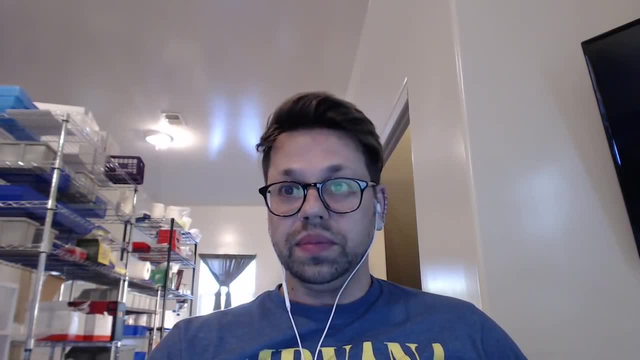 So you can, you know, Say, make some plates on a Wednesday night And then do the experiments on Saturday. That's what I would suggest is, You know, Just doing it, Doing a little bit at a time, Don't overwhelm yourself. 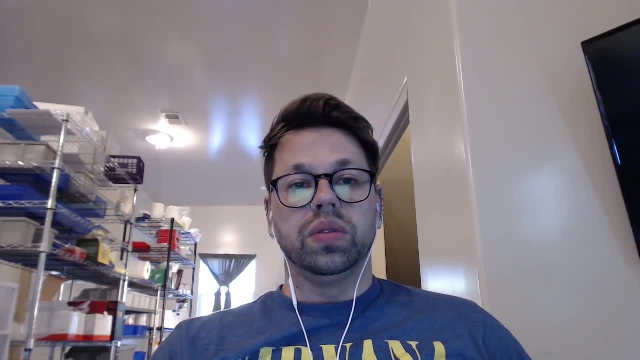 Don't try to do everything at once. You know, Read through the protocols. I think somebody was mentioning how You know They need to read through the protocols A little bit more carefully. You know. You know, Read through it. 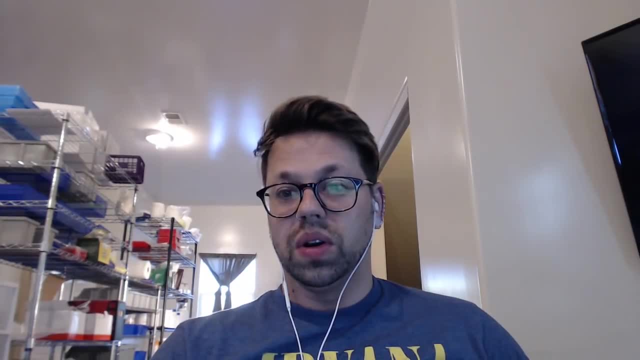 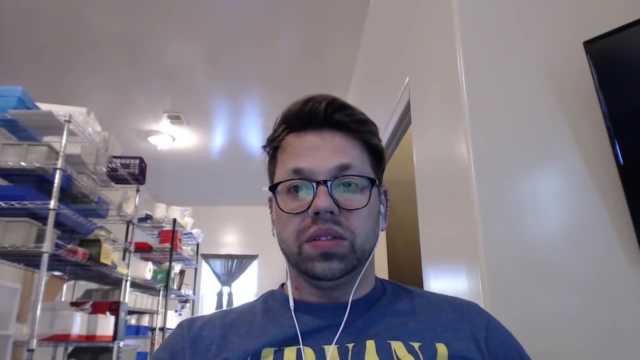 And ask questions. You know That's what the class, The Google Classroom, is for. Feel free to You know. Ask us questions, Ask whatever you need. We're here. We're here for you all To learn. So. 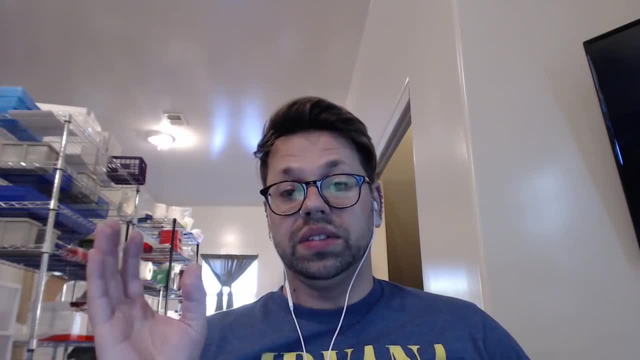 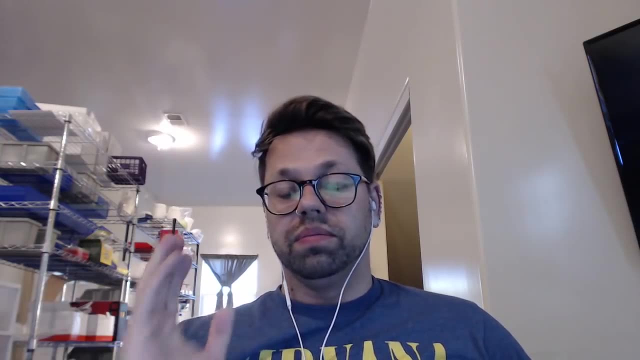 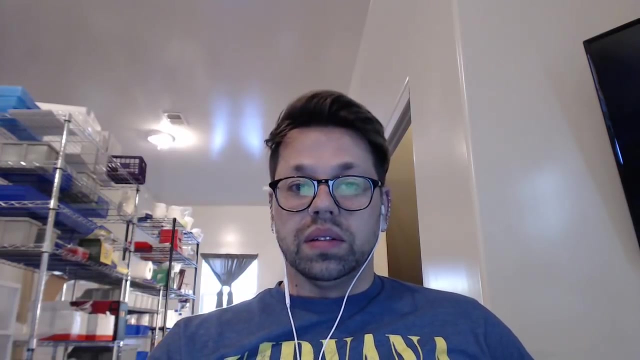 Ask us questions, Constantly ask questions. When we have these live classes, It's the perfect opportunity to ask questions, Because We are going to Be here to answer your questions, Right? So Let me see: Do we got anything else we need to? 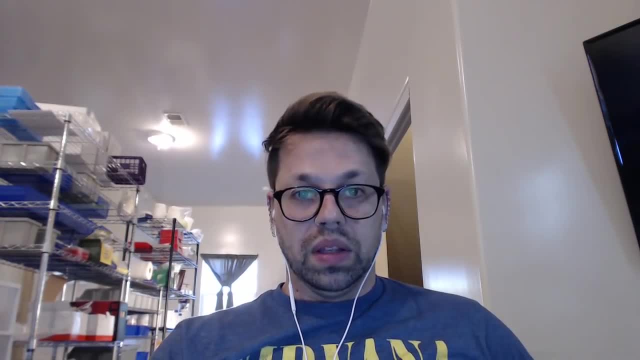 Go over, Describe and explain. I think that should be About it. If you have Any questions About the syllabus Or anything like that, Feel free to Again ask And we'll We'll figure it out So. 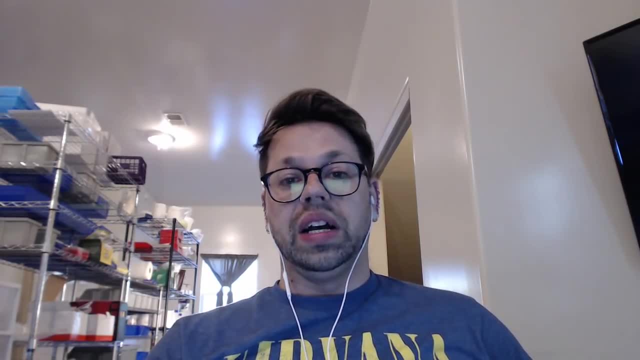 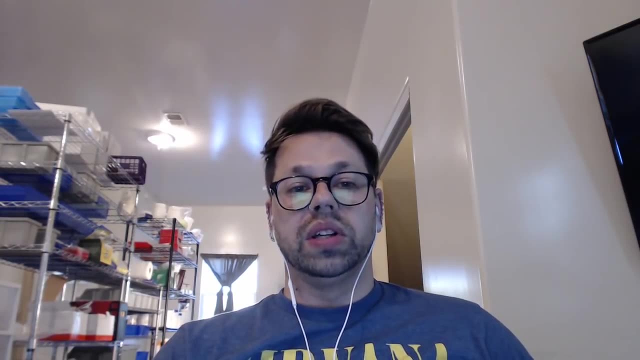 Week one And two We are going to focus on Cell biology And learning Some basic Lab techniques. Now, some of these things. They're marked as assignments. That was just an accident. You don't have to turn anything. 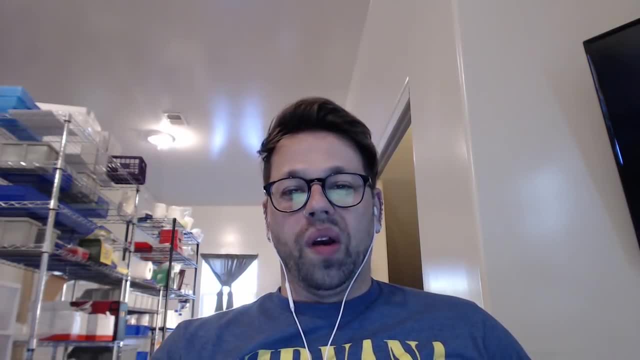 Turn, Turn these things in. But I appreciate People who are turning them in. You know That's, That's great. It means a lot to me. But Don't worry about turning them in, Just make sure you read them. 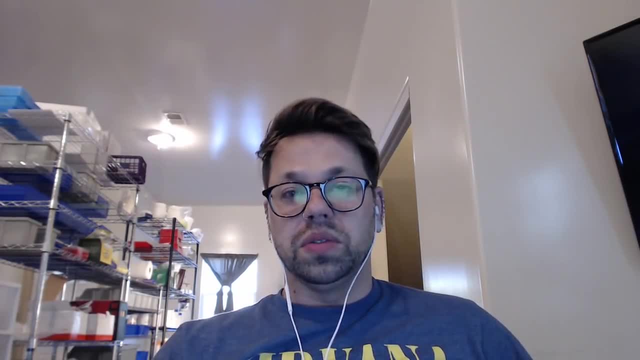 And go over them And figure out what's going on. So each week We should have like, Or every You know Week or two, We have these Read me firsts. So Make sure You obviously Read those first. 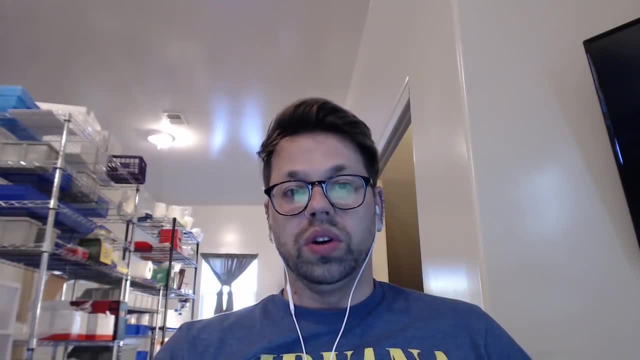 They'll give you an idea Of what's going on, What you should know, What you should be prepared for, What papers you should read And stuff like that. So this week We're going to learn How to use pipette. 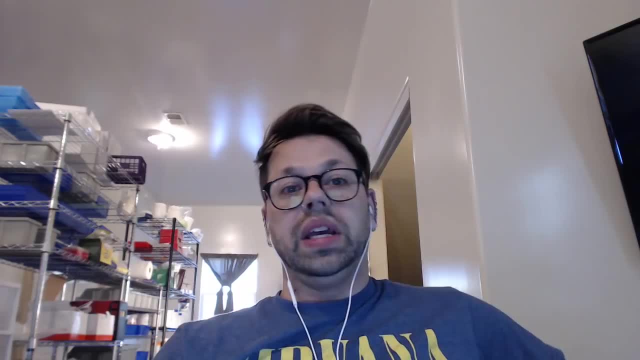 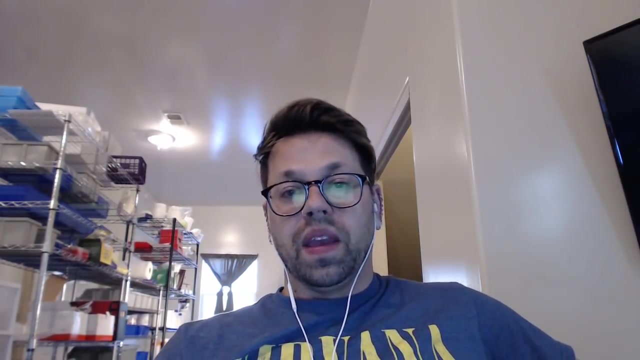 And scale And Make plates And sterile technique In the next two weeks Um Do some cultures And, You know, Just learn How to work with Basic molecular biology Lab supplies And Make sure you You do this stuff thoroughly. 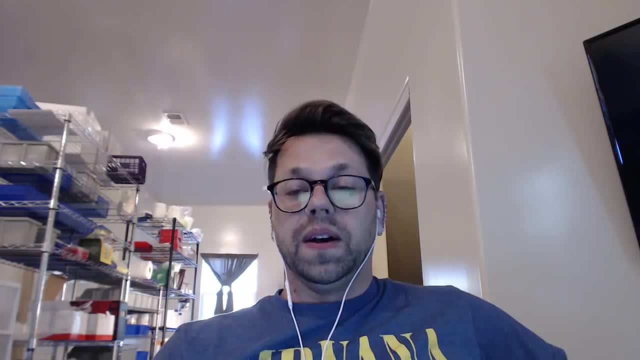 While pipetting Might seem simple And easy And, Uh, People Underestimate it. It's probably The largest Place where people make Errors- Professionals And People just starting Alike Like You, make errors. 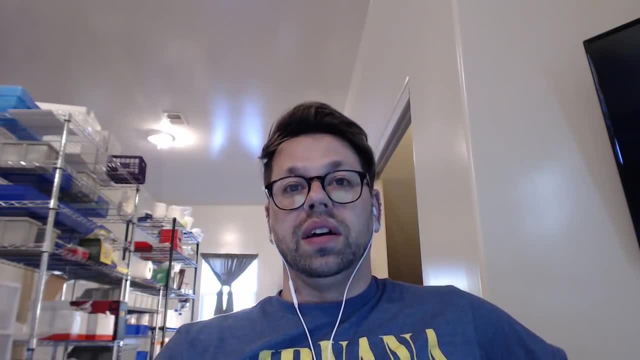 Doing pipetting, Not paying attention To your pipetting, Um, Not being good at pipetting. So What you want to do Is You want to Make sure that, A hundred percent, You know how to pipet. 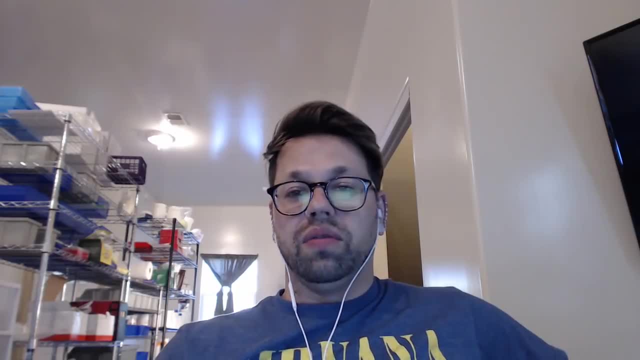 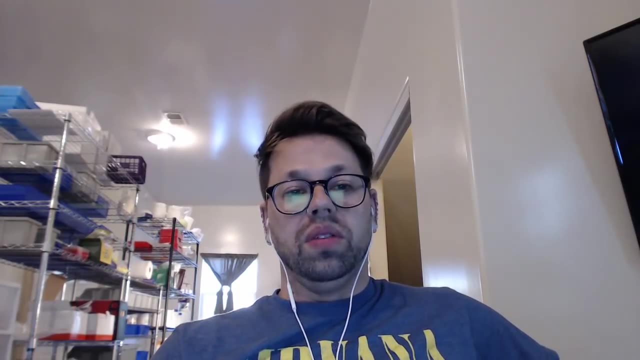 And A hundred percent, You're always Looking at it, Focusing on it. Make, Making sure you're doing it Correctly, Right, Because, like If you add the wrong Amount Of liquid Or Or solution. 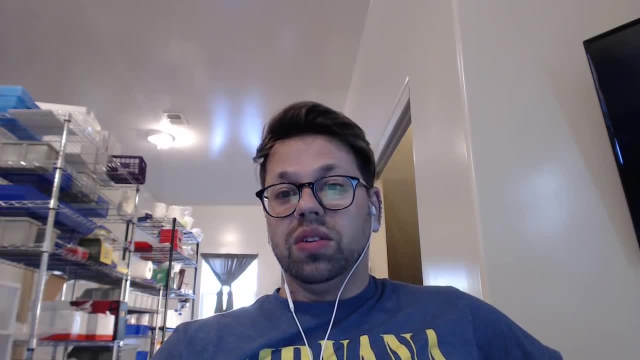 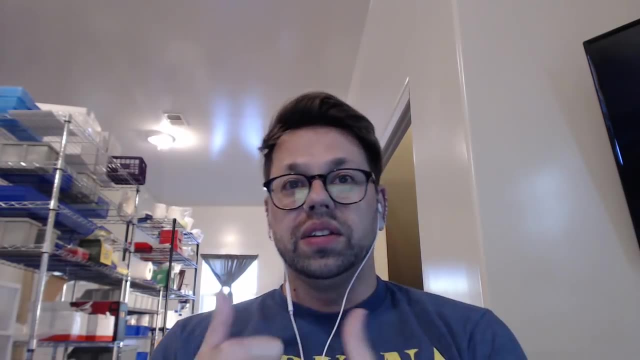 To your, To your experiment, Like: Obviously It's going to go wrong. If your equipment's not working, Obviously It's going to go wrong. So You need to make sure your equipment And And you Are. 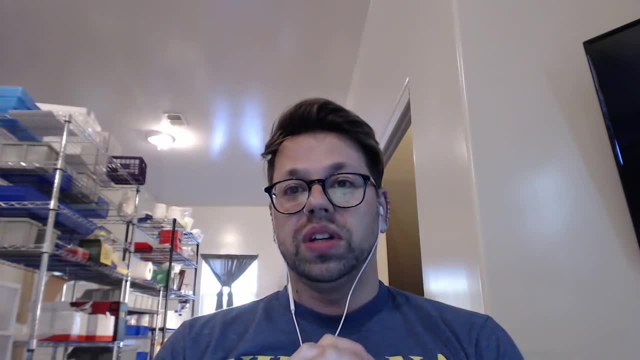 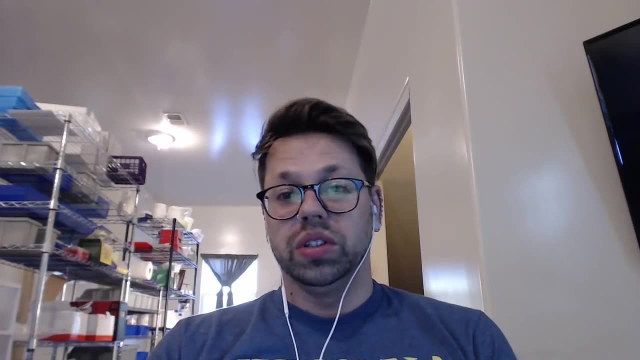 Using it correctly First, Before anything happens, Right? So Make sure you Go over that pipetting Protocol Experiment A bunch of times And Jill's going to show you In a little bit How to use some pipettes. 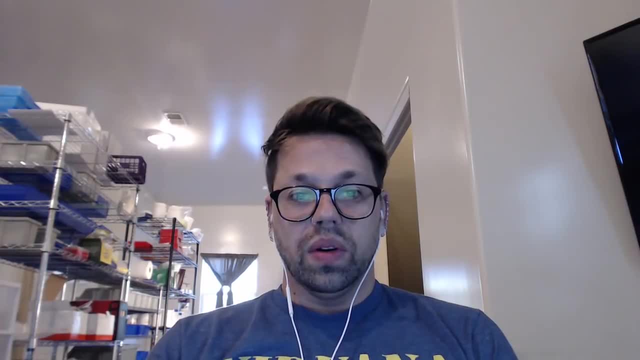 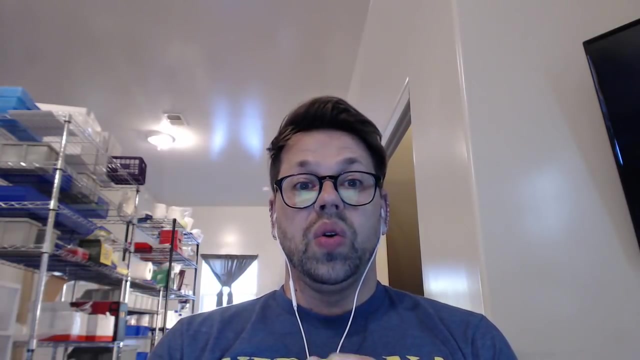 So Over the Next Two Weeks We have Two papers, And They're both Related to cell biology. One is On How To create Embryonic stem cells, Which is a really cool paper. 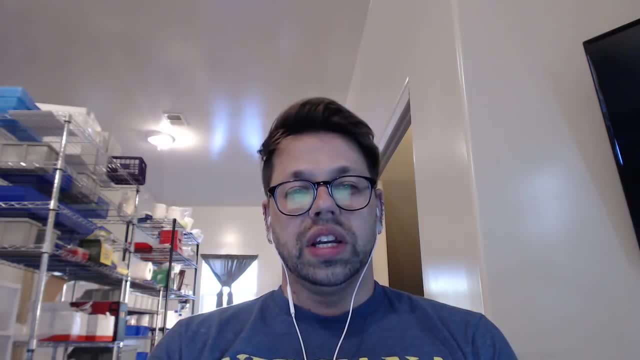 And it just discusses a little bit About Genetic engineering And how you can Genetically modify, Genetically modify An adult cell And turn it into a, A pluripotent stem cell. Pretty, Pretty cool, It's. 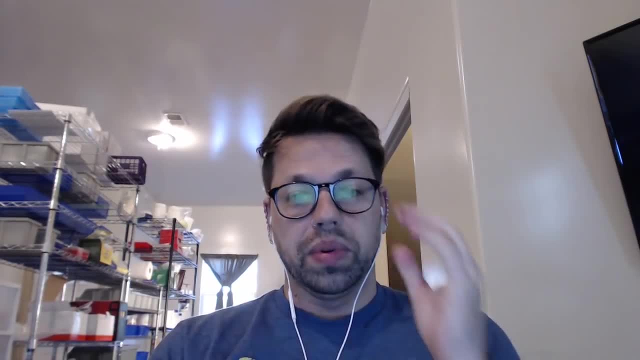 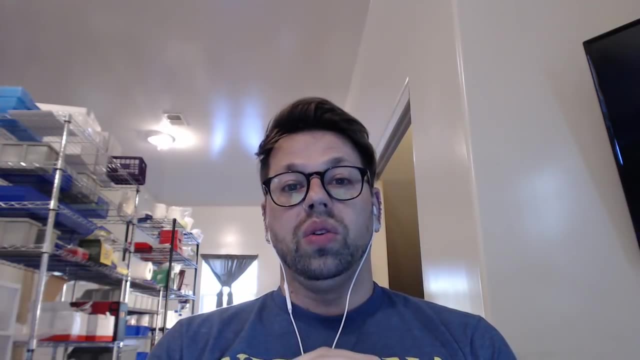 Something that hopefully Will capture your imagination. And the other paper Is about The creation Of a bacterial cell Where the whole genome Was Made Using DNA synthesis Rather than coming from another bacteria, So that was a pretty epic paper. 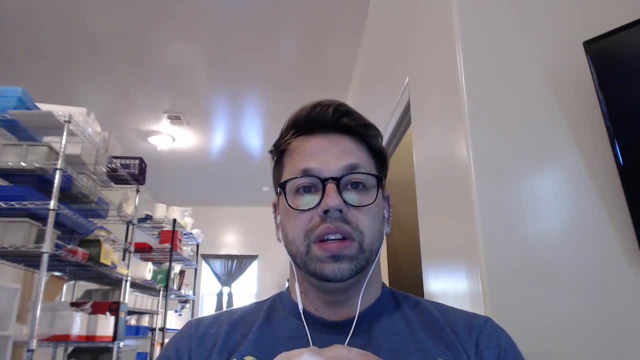 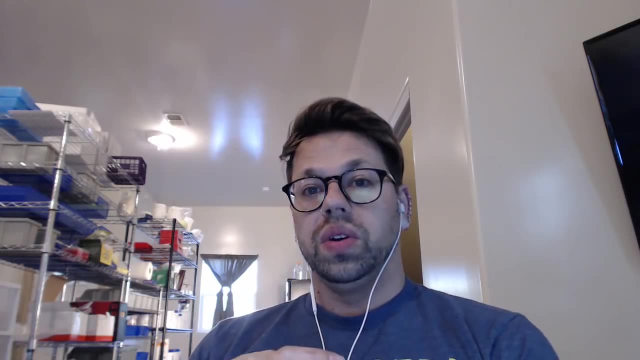 When it came out And people were really impressed. Now they're trying to Make Synthetic genomes For yeast And even humans, Hopefully in the next few years. So You know, Things are moving along With that stuff, But it's. 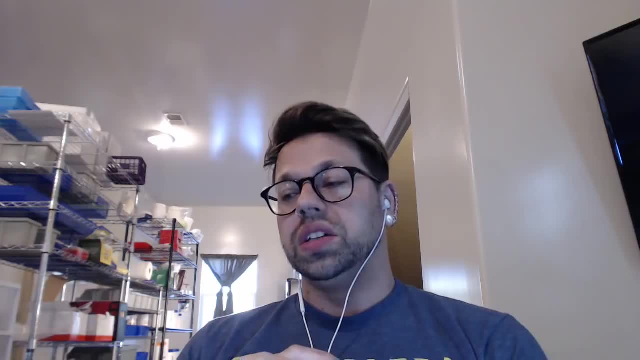 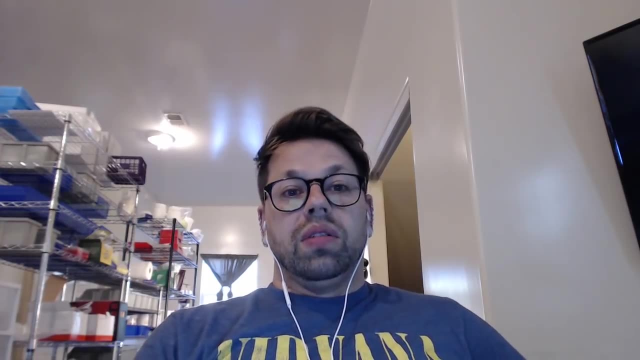 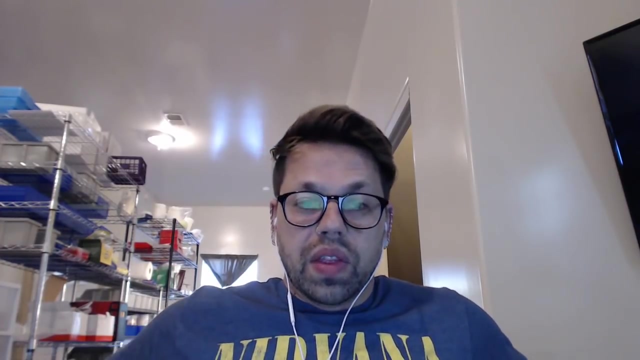 It's really interesting Just to Try to imagine What, What we can do And what can happen, Right All right. So There are A few things That You need to Remember when We're talking about cells. 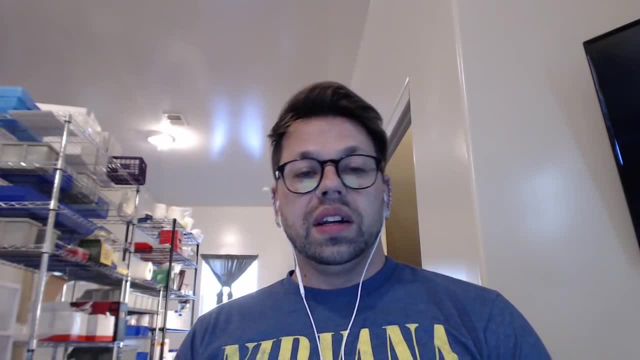 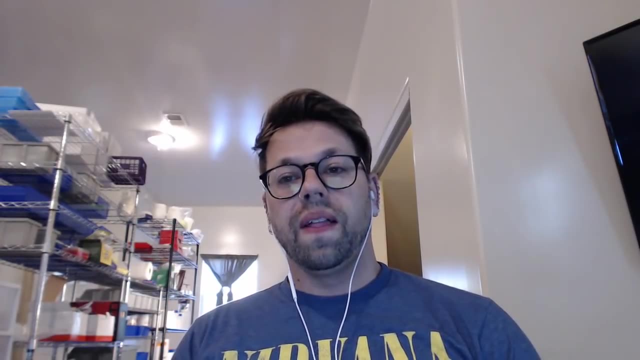 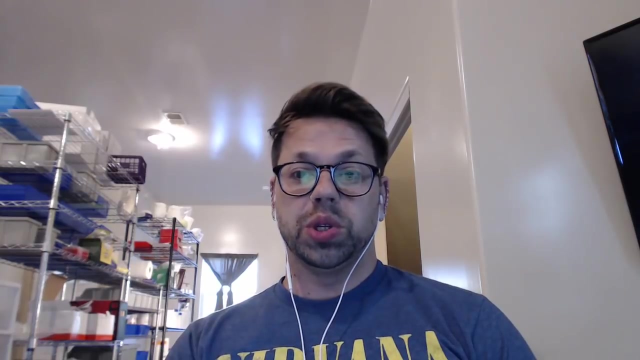 Right. The first Is that, As far As we As humans Have figured out, Cells only come from Other cells. Now There's been some work By people To try to create Synthetic cells, Cells from scratch. 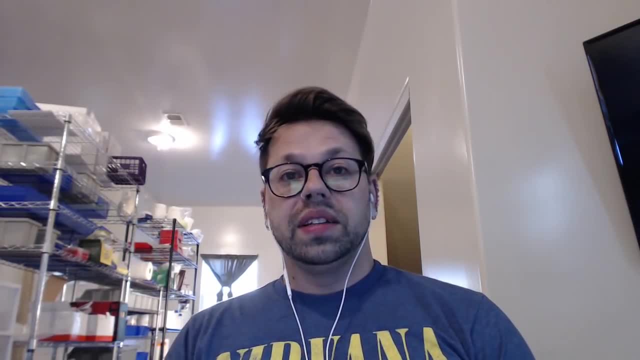 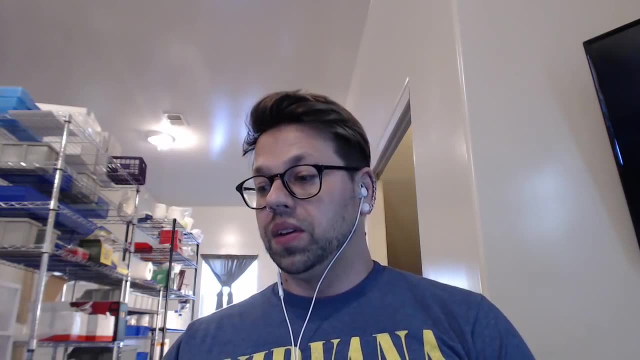 And all this other stuff. But, But Cells, All the cells That we know Came from Other cells Which You know. For me, Every time I think about it And talk about it Kind of blows my mind. 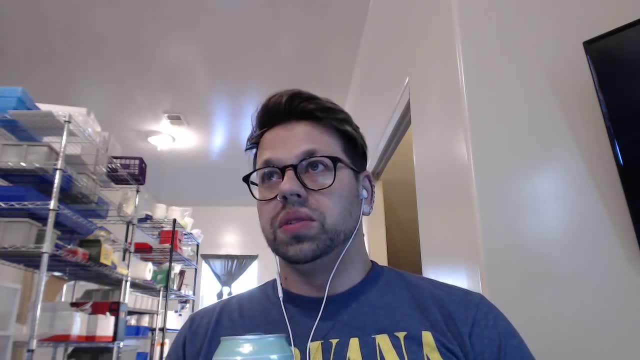 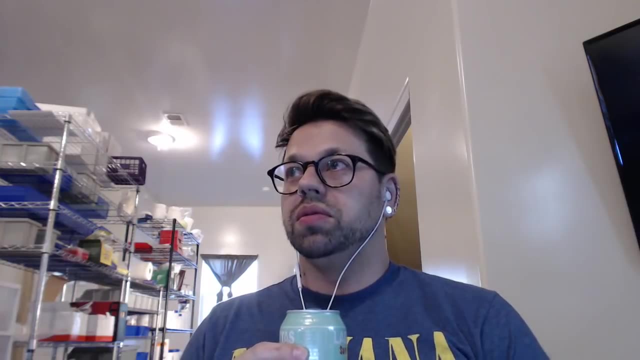 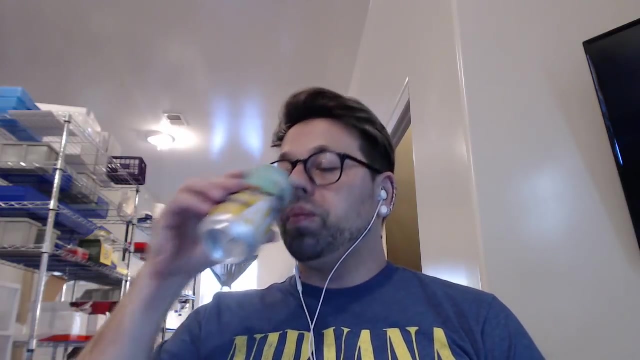 Right That, like That's. all we know Is cells from other cells. We We don't know Cells That Have been made from scratch. I thought we were A lot further along Technologically- Technologically. But 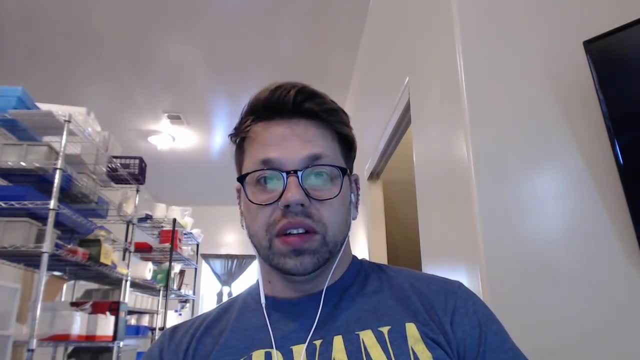 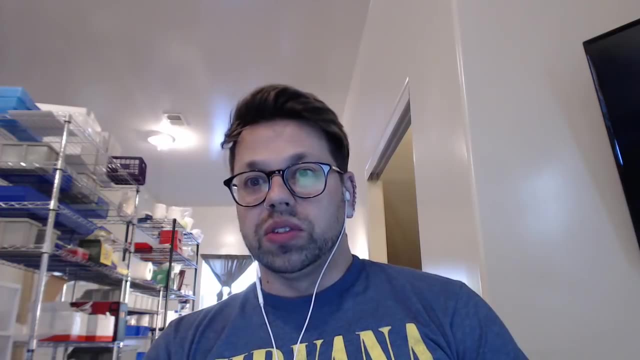 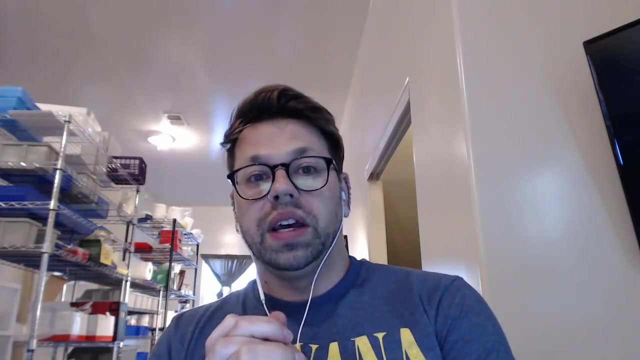 Yeah, It's. It's pretty cool, though, Right? Because cells Are self-replicating, Self-replicating matter. So When you genetically engineer cells, What you're basically doing is You're genetically modifying Self-replicating matter. 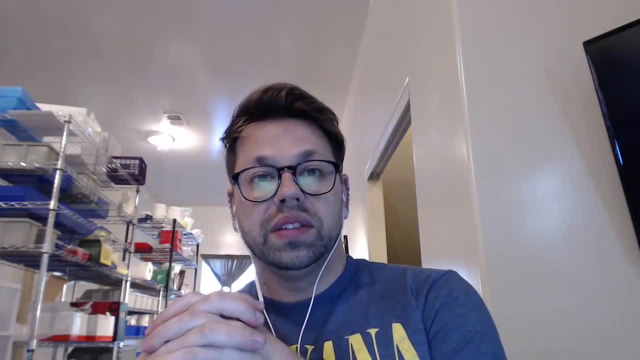 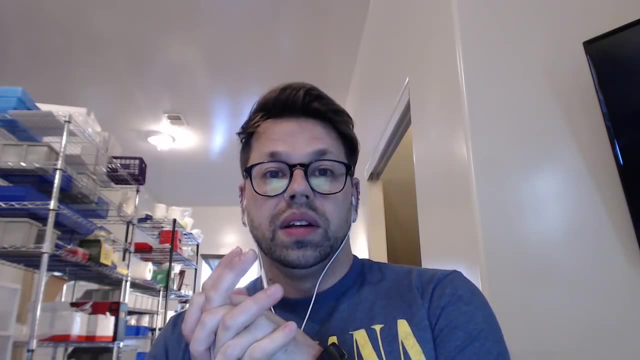 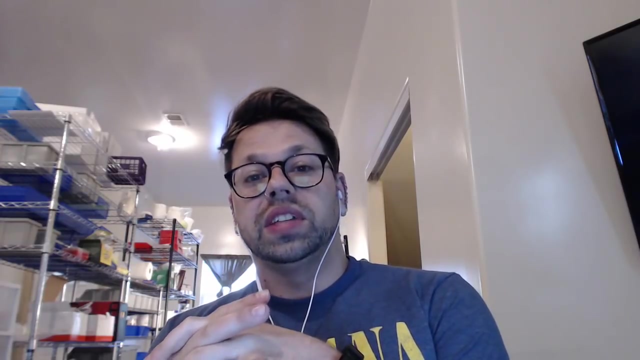 Right, They can grow into stuff And build stuff And create stuff. So It's something that is Pretty cool, At least To me. So Cells Come In All different shapes And sizes, So when you're talking, 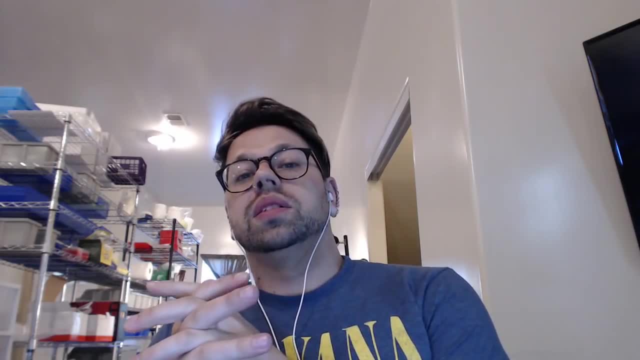 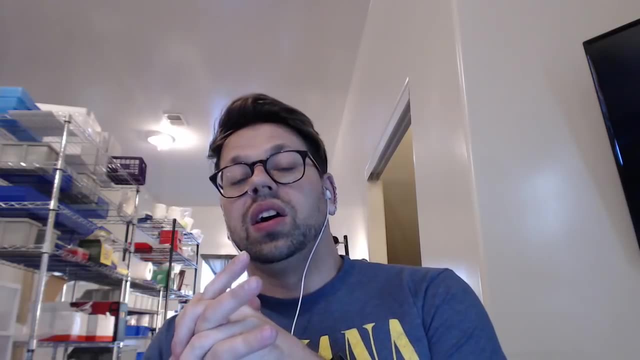 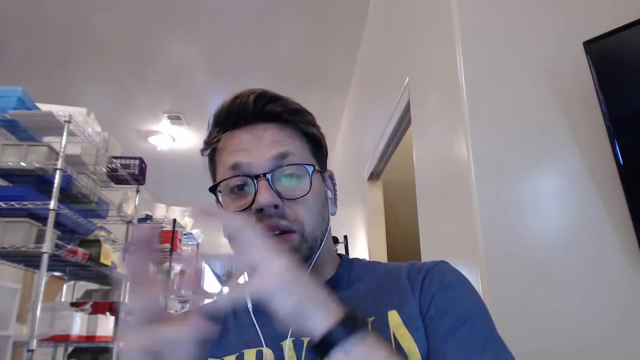 When people are talking about cells, It's It's very Like you need to know What type of cell People are talking about. Right Bacterial cells Can be, And usually are Extremely tiny Right And Are generally hard to see. 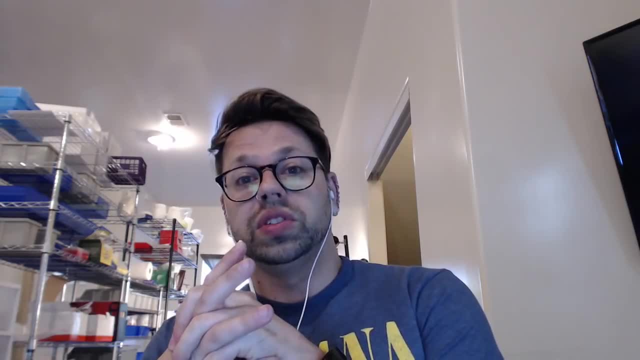 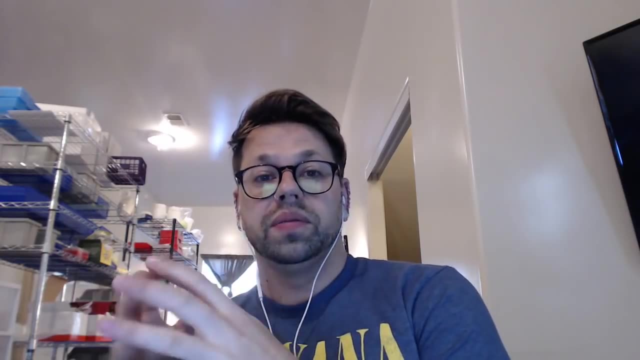 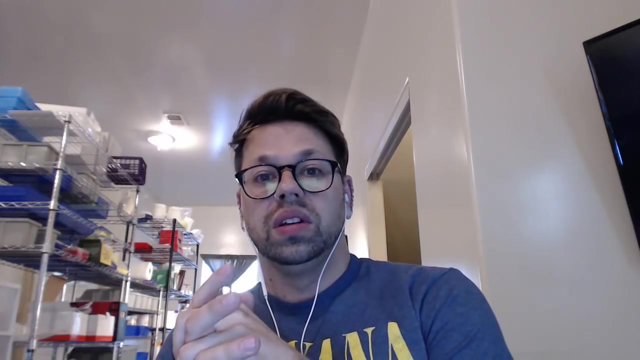 Under A light microscope Or, just, like You know, A normal microscope That people would use Every day. Yeast are A little bit bigger. Plant cells Have different cell walls And different organelles. Right Human cells. 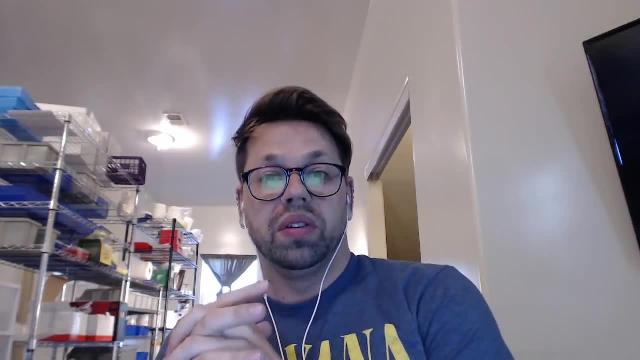 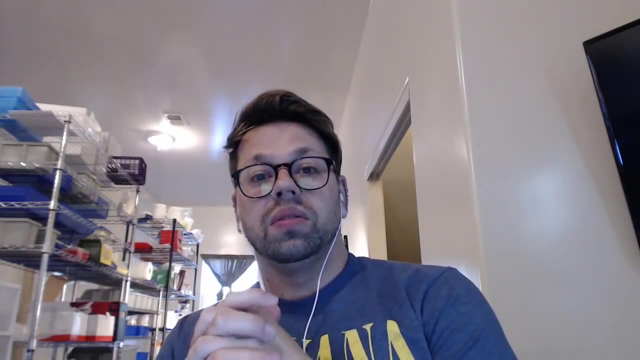 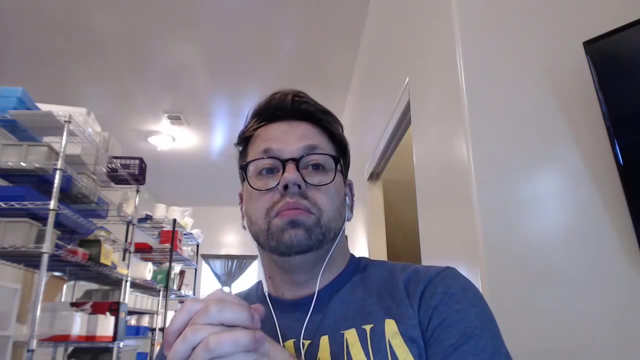 And mammalian cells Are really big, Bigger Than both yeast And bacterial cells, And different than plant cells Also Right. So When you're thinking about Genetically modifying An organism, The type of cell Matters. 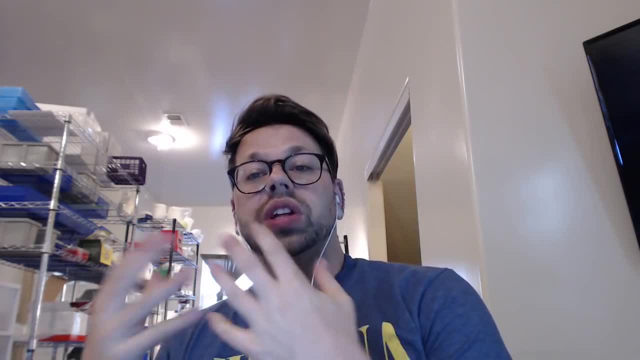 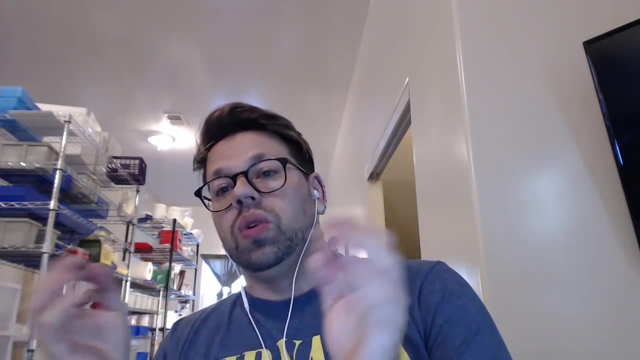 Right. It's going to be a lot Easier to Genetically modify A cell Like A bacterial cell Because It's cell walls Are more permeable- You can get stuff in easier- Whereas a plant cell. 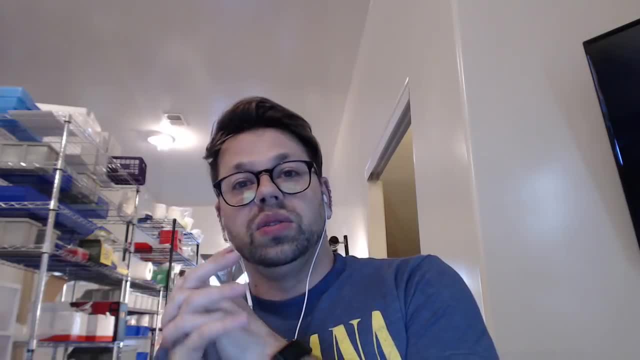 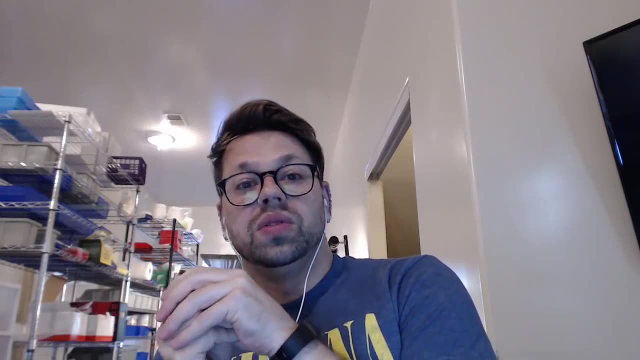 You know That has. What is it Like lignin And cellulose Around the outside. It's a lot more difficult To get stuff Inside the cell, So they use techniques Like gene gun Or Agrobacterium. 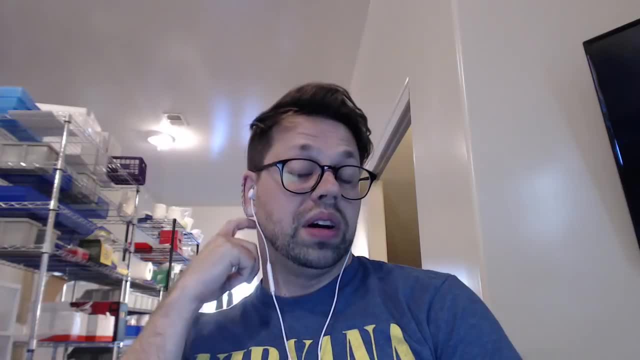 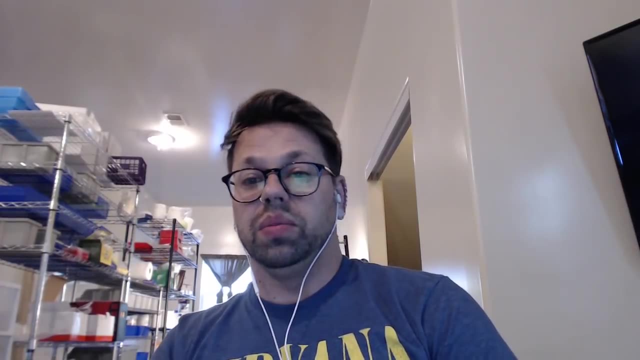 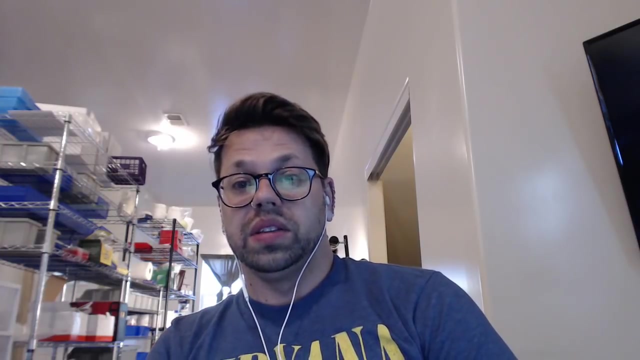 To get DNA Inside the cell Plants are A little bit harder To genetically modify, But not Not Definitely Not Impossible With a, A DIY method Or somebody In a home lab. It's Something that 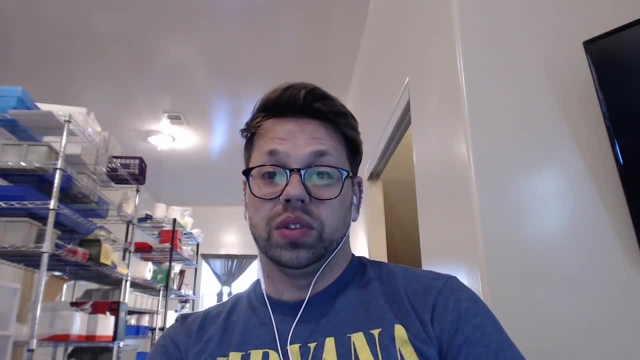 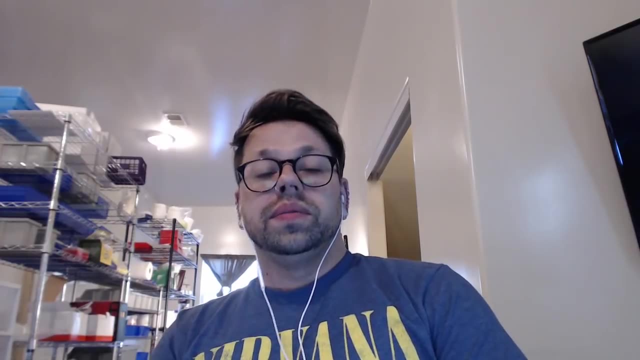 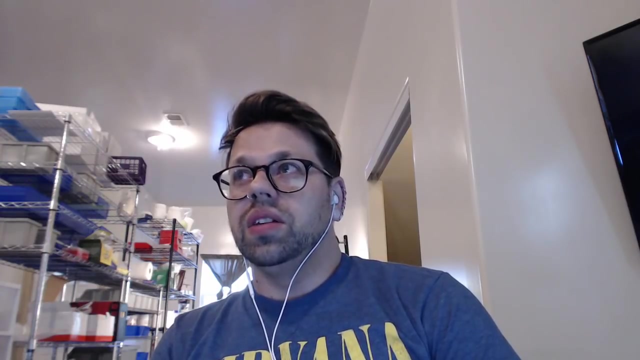 You know, You can learn With practice And over time, All right. So All Living cells I always get, So viruses are Variants. I don't think they're cells. They exist in a capsid Right. 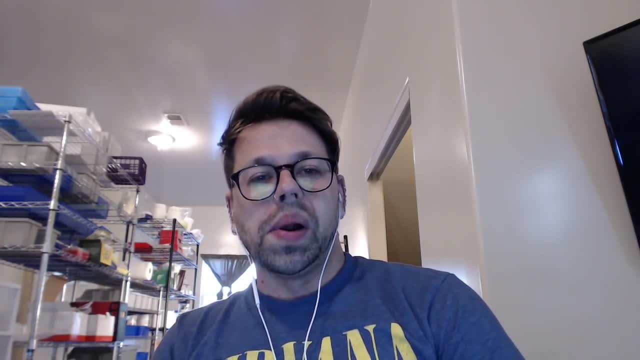 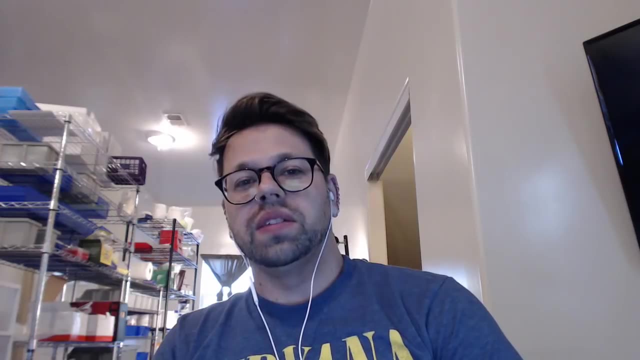 They don't consider Virus capsids Cells. I have written down All cells of DNA And replicate their DNA In the same way And I don't know if that's true And I'm trying to, You know, Prove myself wrong. 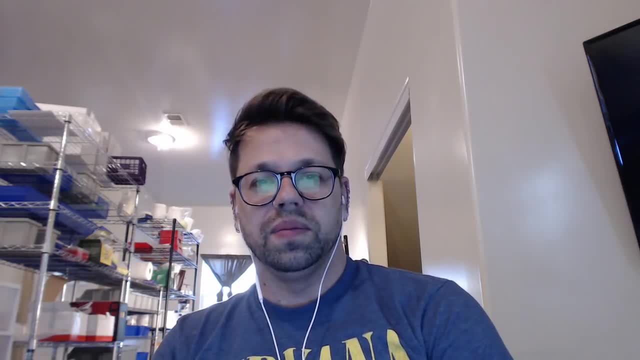 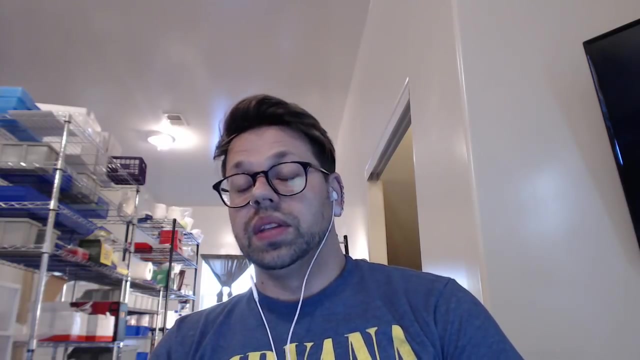 But I can't think of any Anything at the moment. But, yeah, So all Organisms That are living- So excludes viruses, Technically, Let's not count those As living right now- Have DNA And They replicate their DNA. 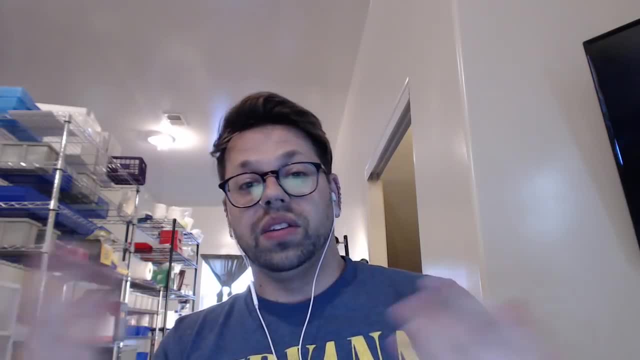 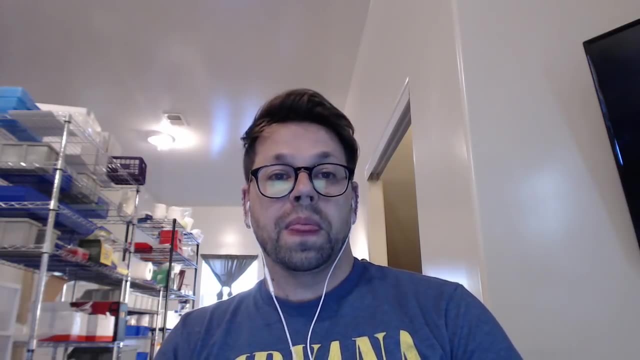 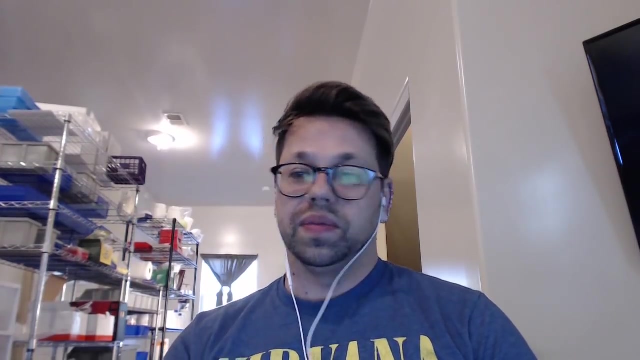 They, And Replicating the DNA Is how they replicate themselves. Right, And the DNA Is what they use To become alive. So DNA, As they always Tell us, Is the building block Of life. I don't know what that means. 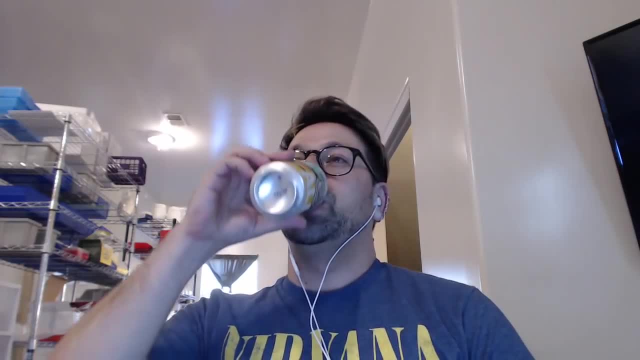 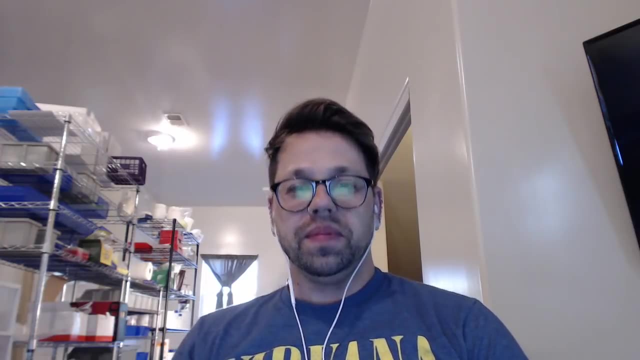 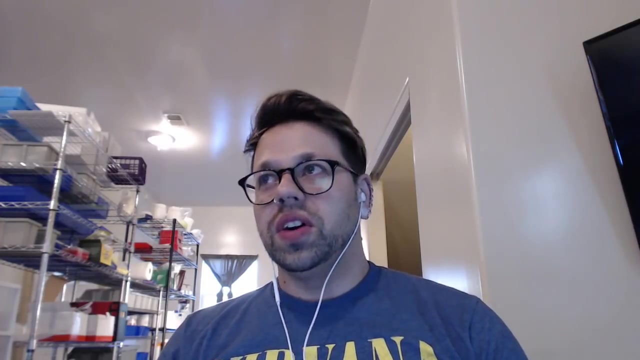 Don't, Don't ask me, Um, But it sounds important, It sounds very important, Um, So. So DNA, Isn't That actually the thing That does anything, Though, Right? So We always talk about DNA. 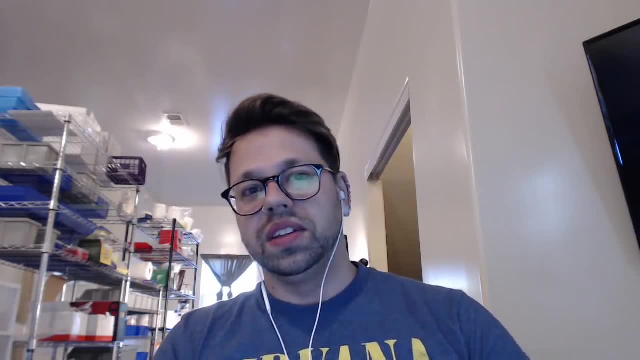 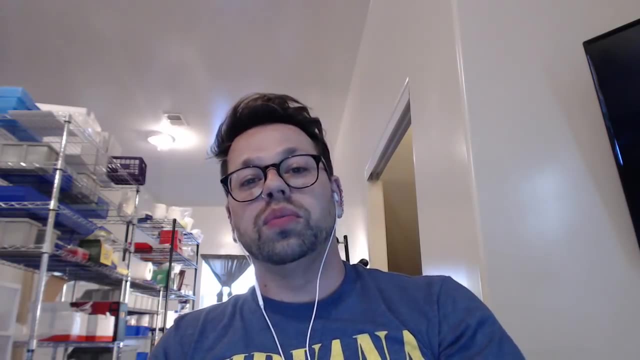 And how awesome DNA is And what DNA does And all these things, But It's not actually DNA That does anything. The DNA Is turned into RNA And then is turned into proteins, And proteins Are the important part. 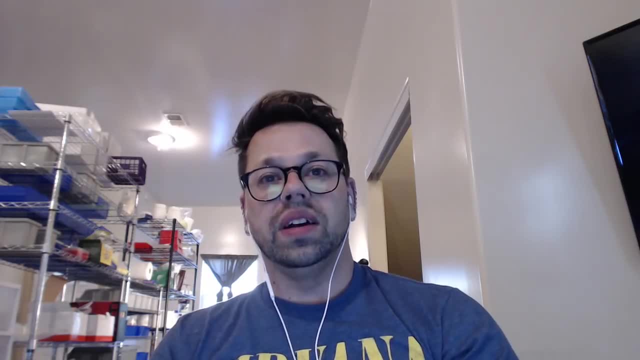 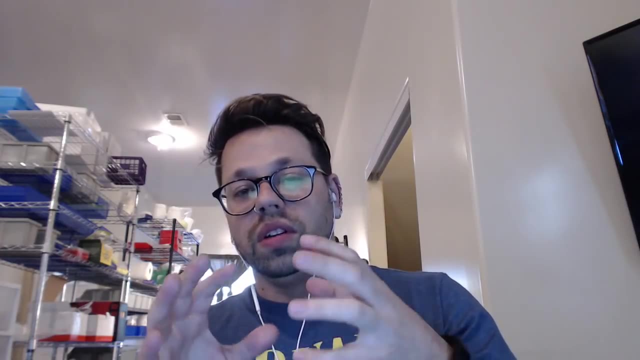 In cells. They are what Makes cells, You know, Alive, So to speak. They are Literally Like these little Nano machines That can move around And do stuff. So like The way you move your muscles. 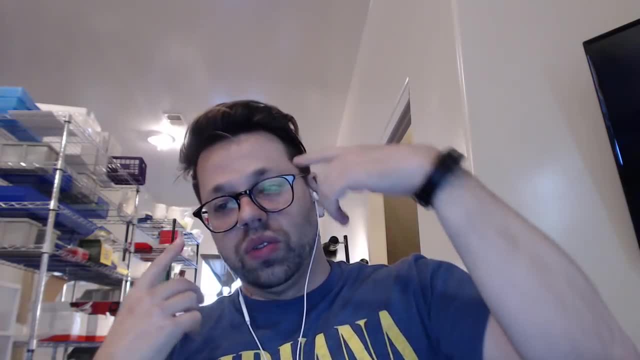 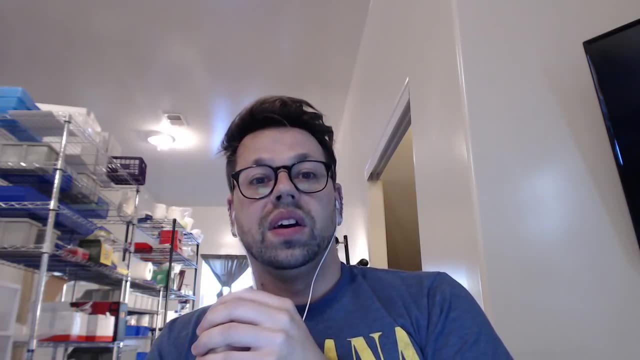 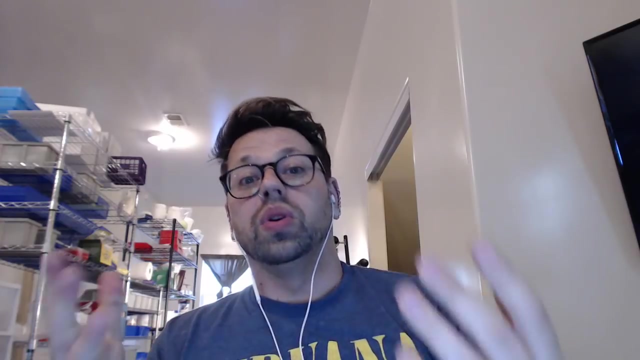 The reason your heart beats, The reason that You know Your brain works. It's all because Of proteins. So proteins Are Are probably more The building block Of life Than DNA, I guess. But proteins Are the important thing. 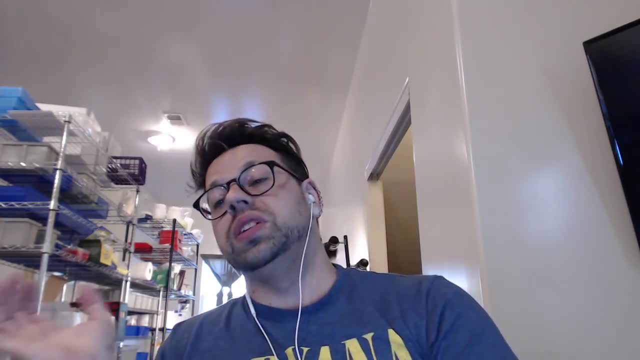 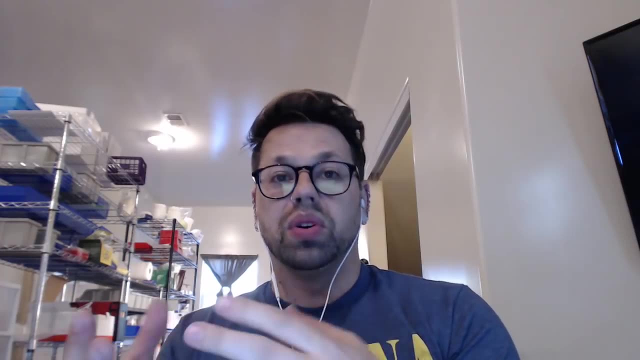 So when you're trying To genetically Engineer something, You're trying To put DNA In the organism, But The only reason You're trying To put DNA In there Is because You want to make Some protein. 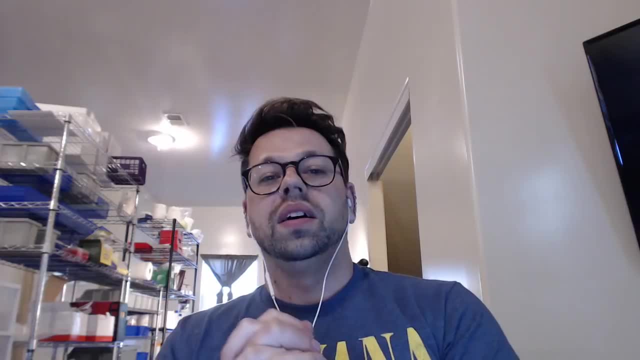 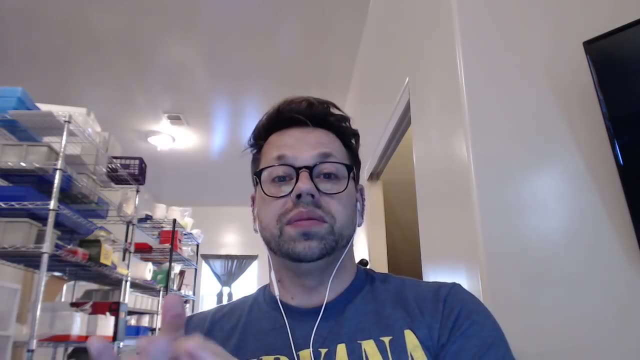 Usually. Sometimes you want To make RNA Or something like that, But generally, Let's just say You know, For most cases You're going to want To make protein. What does that protein do? Maybe that protein Replaces a disease gene? 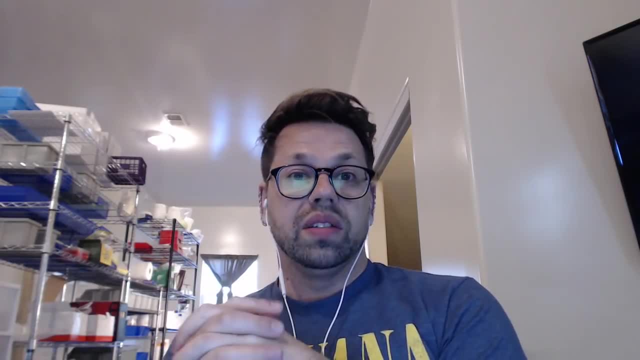 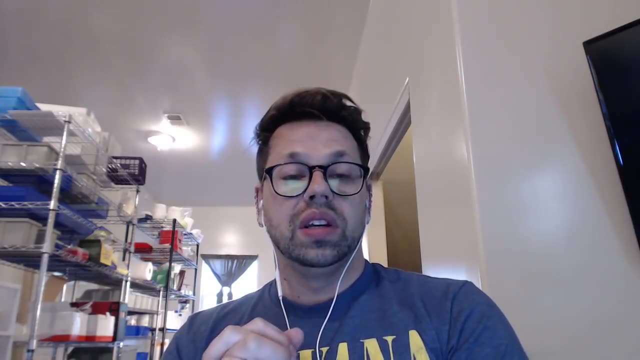 Right. So unlike Cystic fibrosis, There's a mutation In the gene. Maybe you want To replace That gene. So You have DNA, Make that protein And you know Muscular dystrophy, You have the dystrophin gene. 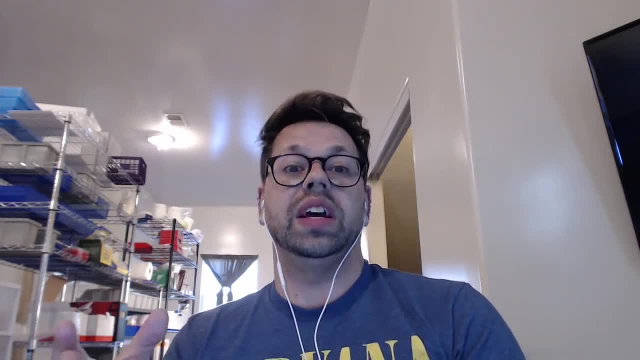 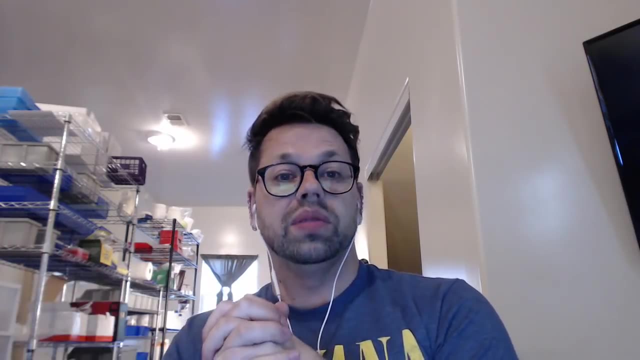 And things that are messed up, And so maybe You just want to put in A new copy Of that gene To make it Function better, Or maybe you want To add in some new genes That do something Completely different. 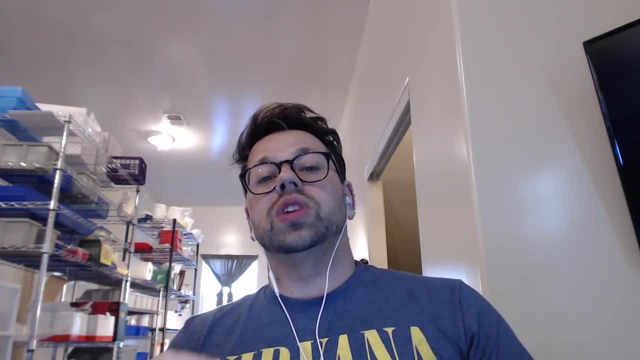 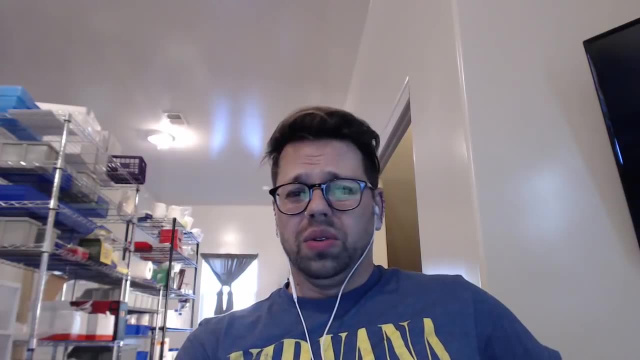 Right So. But what you're trying To do Is you're trying To put in these genes To make new proteins, To make Cool things For Maybe not cool things, I don't know, Maybe you're really boring. 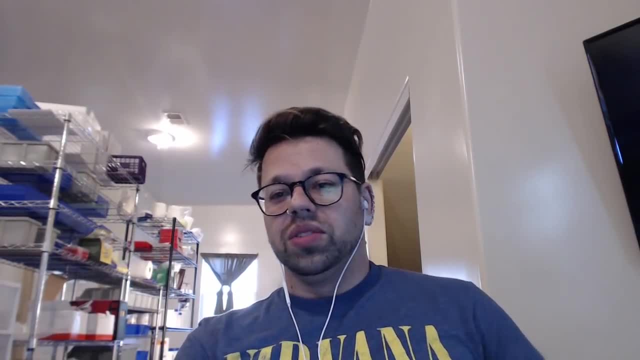 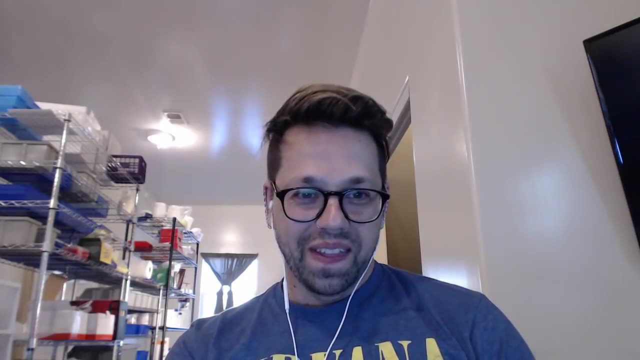 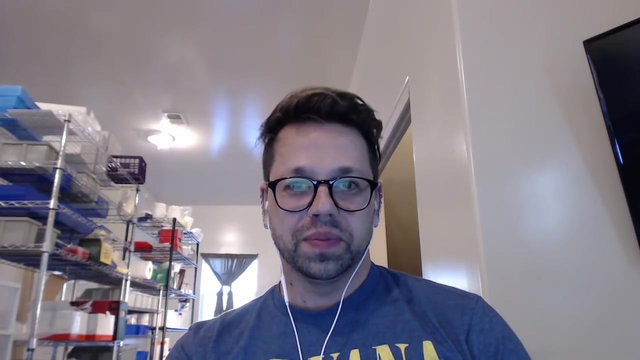 Diatoms. Oh man, Ted, Ted's really trying To throw out the tough questions Early. How do Diatoms Replicate Diatom Reproduction? All right, Here we go, Let's see. Oh no, 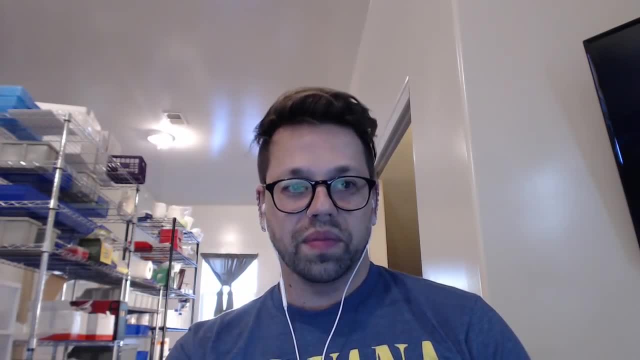 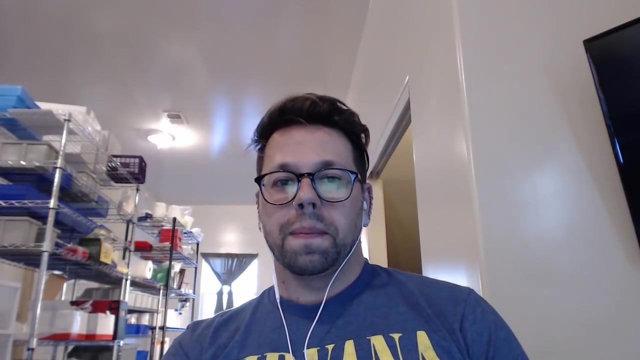 They Diatoms Reproduced By binary Fission. So Yeah It's, It's Similar To like Bacteria, Things like that. So So All right, So Proteins, We're going to learn. 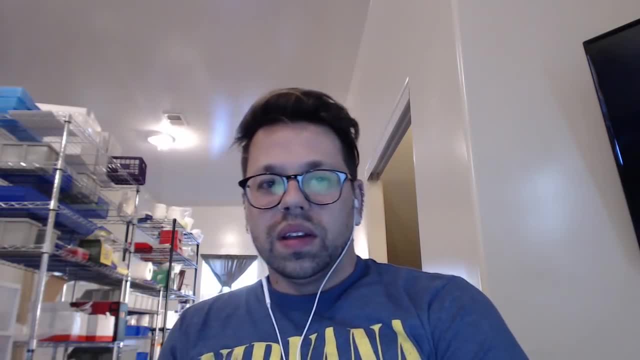 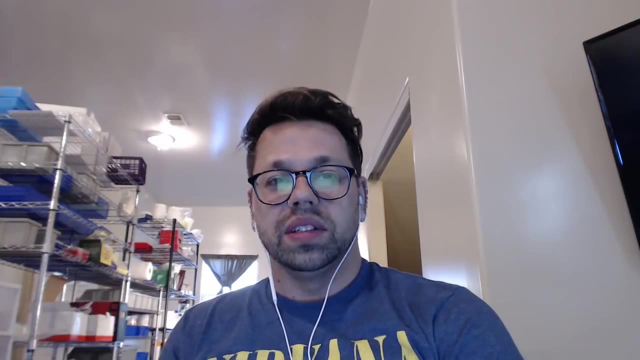 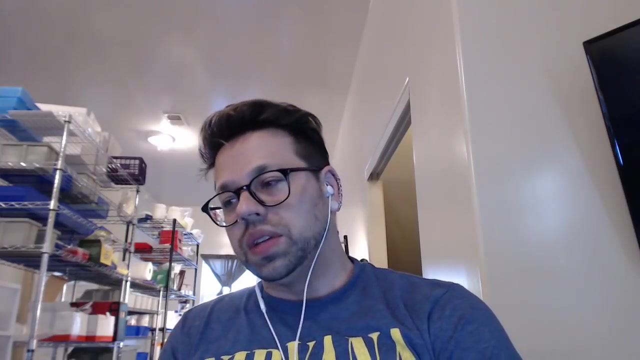 About proteins. Understand That like The amount Of DNA In an organism Isn't related To its complexity, So Genome size Is not Related To the sophistication Of an organism. Sometimes It's easy To get caught up. 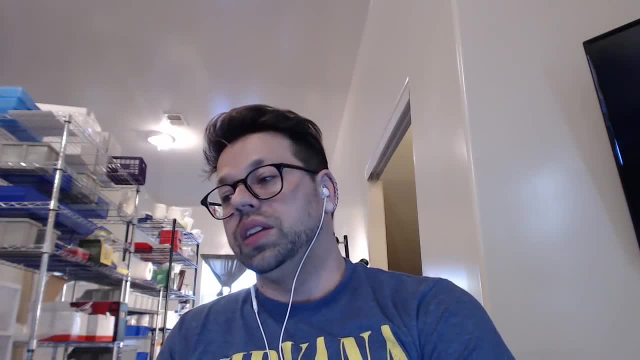 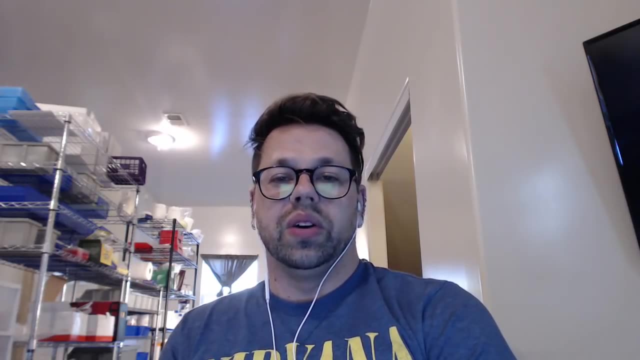 In that, Because you can be like, Well, Most bacteria Have tiny genomes And humans Have big genomes, But Despite That Easy To pick out Numbers Like Plants Will have Way more, Way larger. 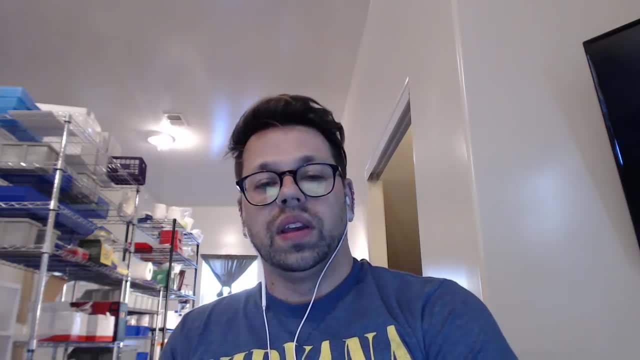 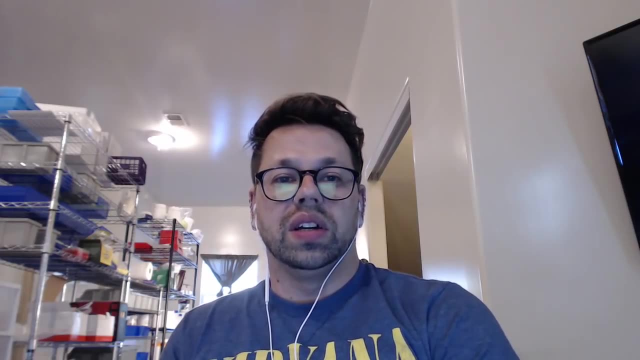 Genome sizes Than humans, And I think, If you look At the list Of genome sizes, There's a lot Of cases Where There's, You know, Non-animal That has Genome sizes Bigger than animals. 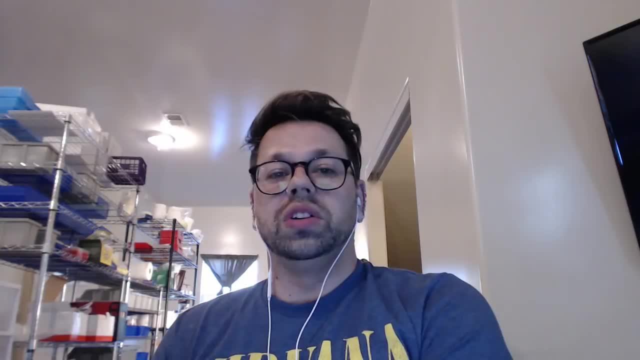 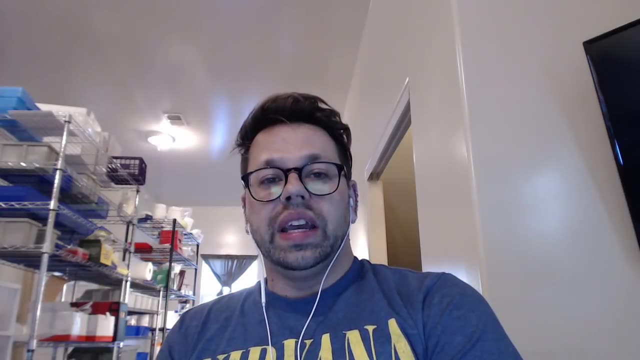 So You know, Don't get caught up Too much In genome size And genes And things like that. It's DNA Is Important, Only in the fact That Let's say It makes Proteins. 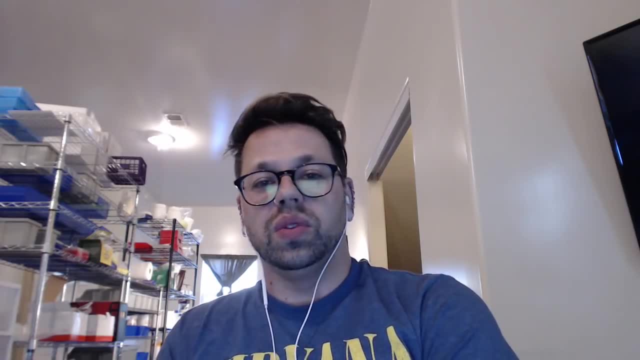 Pretty much. There's a lot Of other stuff In DNA That's useful, But Generally The important part Of DNA Is the protein making And what those proteins do, Whether they turn you Into a plant Or a human. 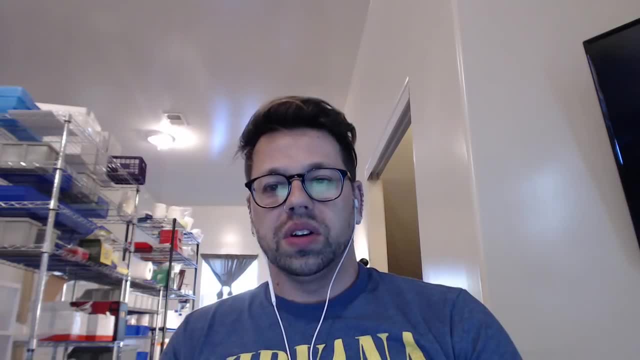 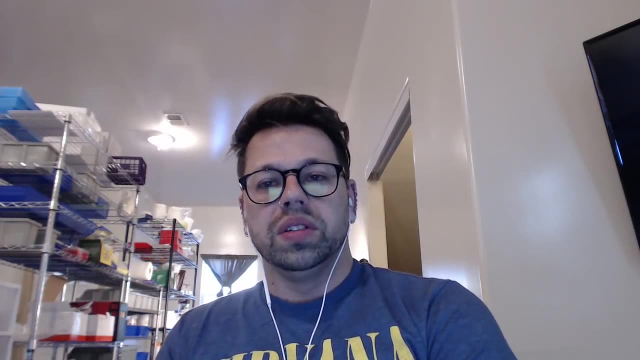 I think we might have a paper When we get to the DNA section That talks a little bit more About this. But You know, Model organisms Are Bullshit. So When you hear About people Trying to use 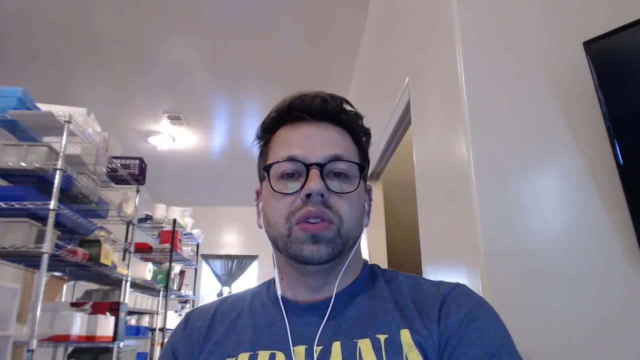 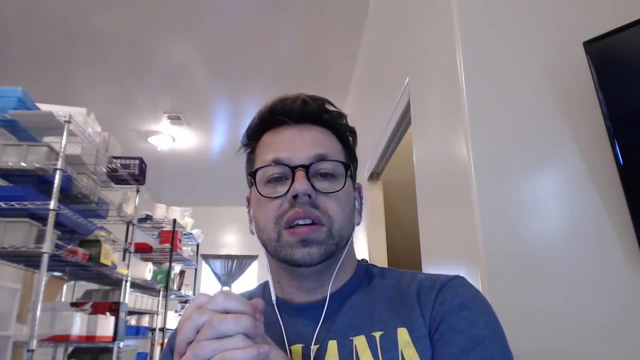 Mice, You know, To Test stuff For humans Or things like that, You have to understand, Even though the DNA Might be just A little bit different, It can cause Huge Differences In terms of Immunology. 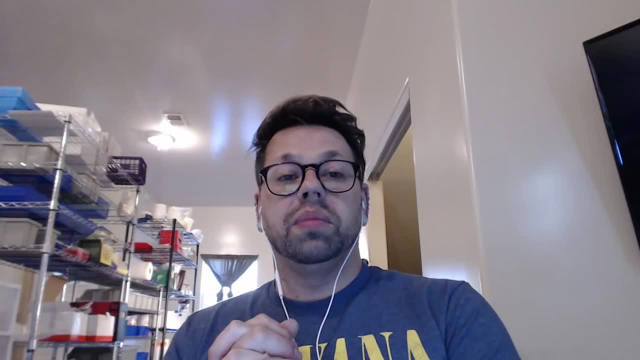 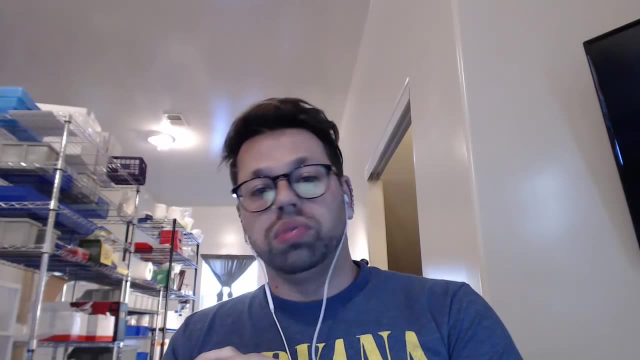 Metabolism, All these things. When people say That they made Like A Drosophila Fruit, fly, Live longer, And They try to relate it To humans, Don't believe them, Don't trust them. 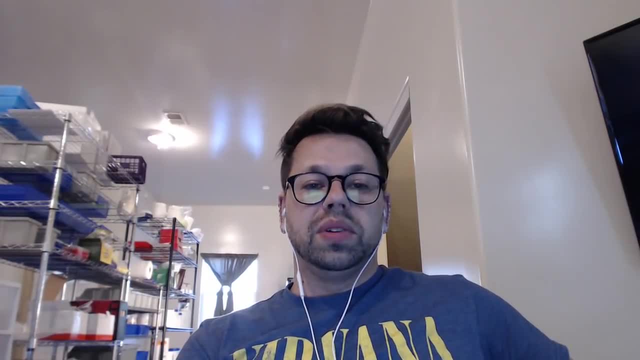 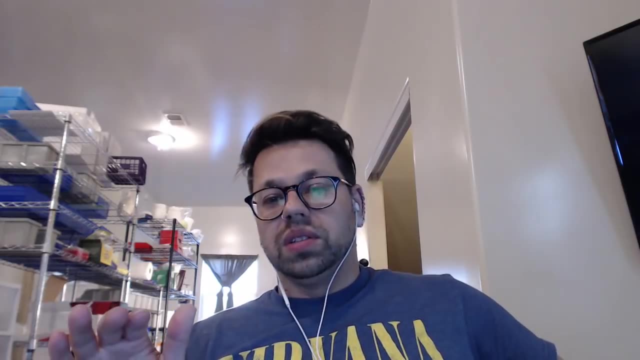 At all. Whenever anybody Doesn't experiment In mice Or Not in humans, And says It's related to humans, Don't trust them Immediately, Think they're skeptical, Right, Immediately be skeptical Of them, I mean. 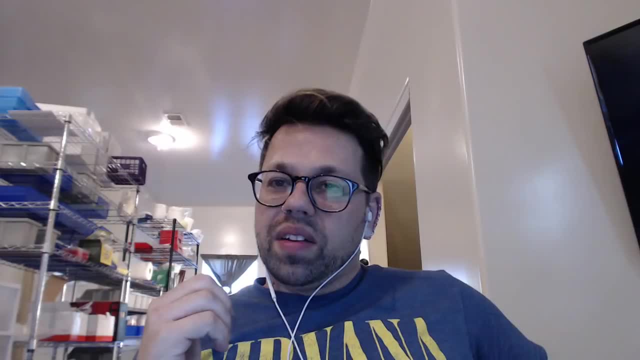 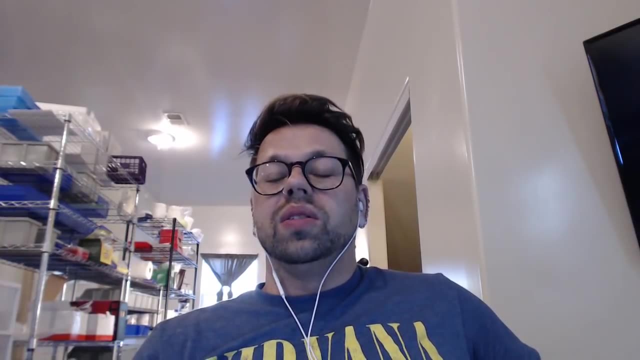 Hey, Brandon, What's up? So? So, Even though DNA's might be Slightly different Or be similar In size And all this stuff, They're not the same. Be skeptical, Right? That's The. 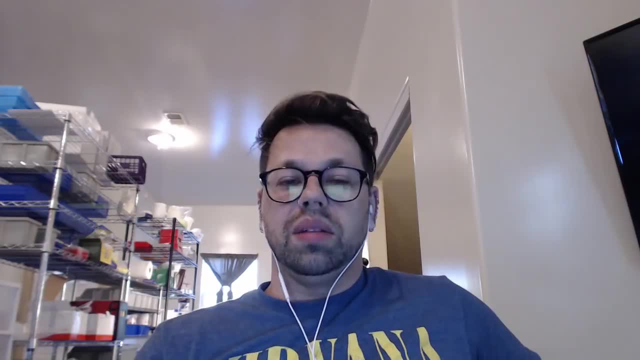 One of the best qualities Of a scientist: Be skeptical- Not about everything, But You know, Try to be Skeptical About, You know, Things that Aren't People are trying to extrapolate, Right? So 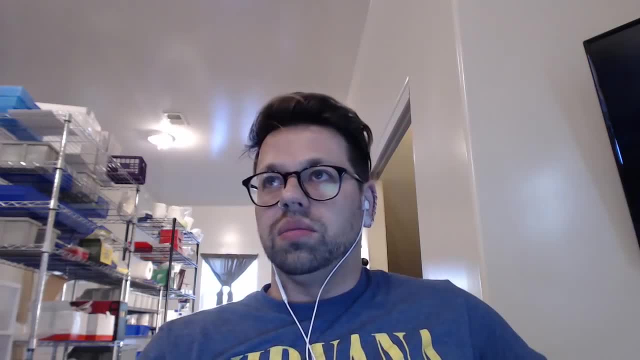 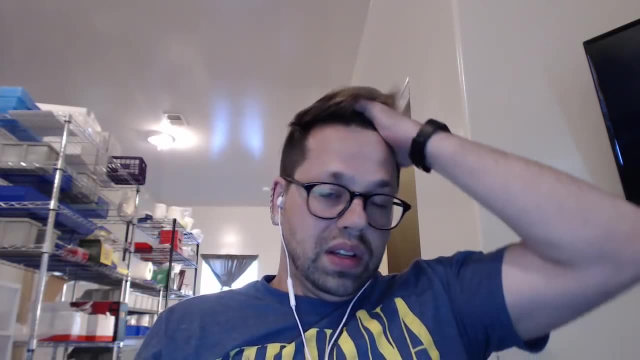 Especially when they're trying to extrapolate Medical data Or Some Cool thing From Mice Or Worms Into humans. Now, When you think of DNA And you think of Proteins And you think of 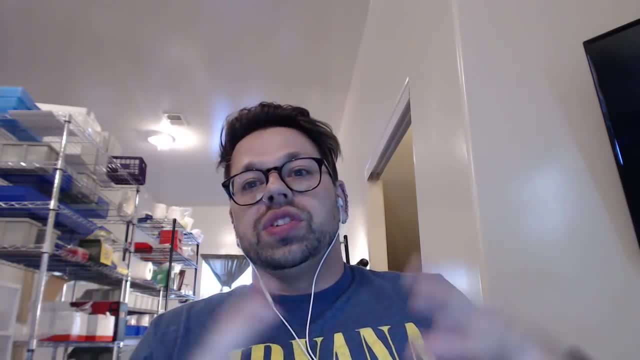 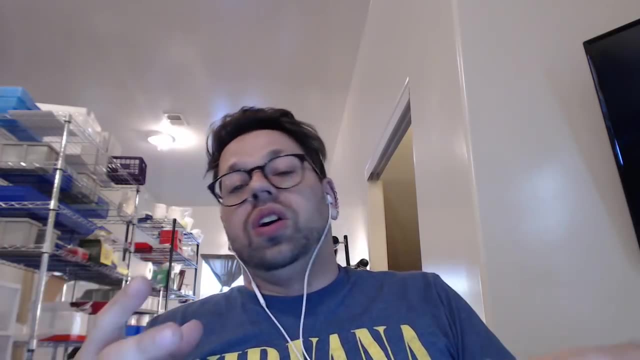 All these things. Now, Basically What they are Is they're just Little Molecules, And a molecule Is just composed of atoms. And what does an atom look like? I don't know? A cloud of electrons Or something. 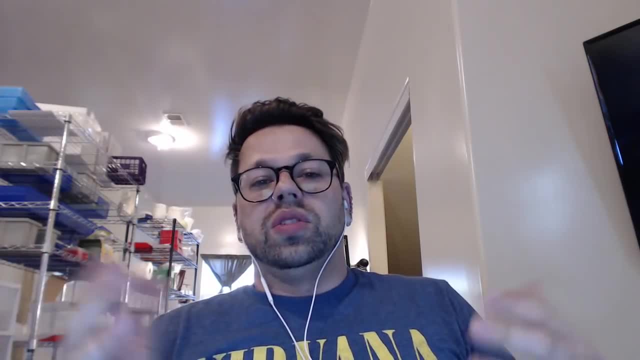 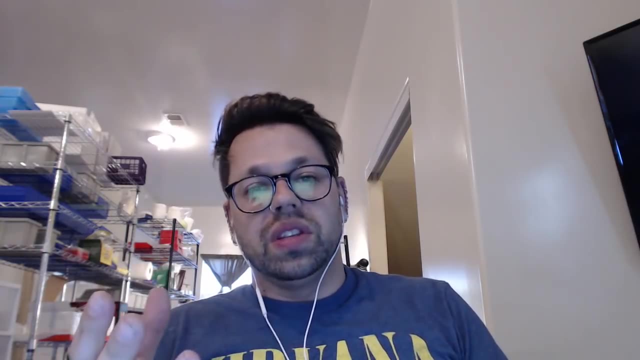 Like We don't really Look at atoms, So It's, It's something That you can't really Visualize, But You know There are representations And things we do To visualize These things. So 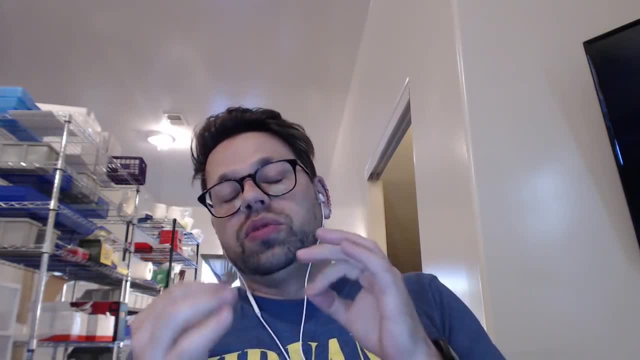 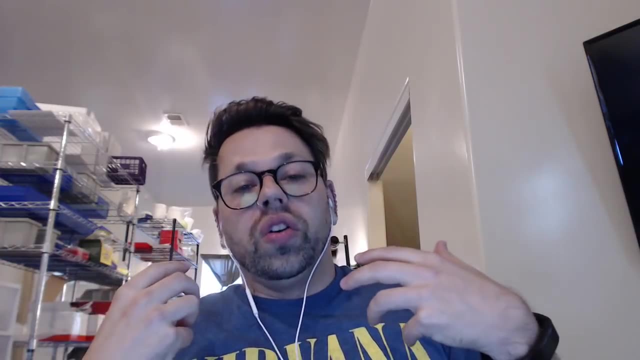 These molecules Of DNA Are physical Objects, But they're so Microscopic That You know It's hard For us to conceptualize them. But These things Are composed Mostly Of just Five different things. 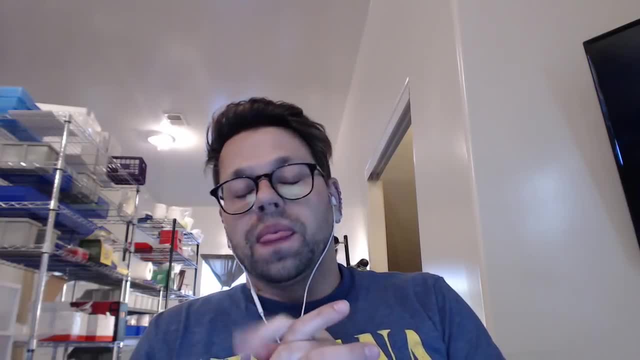 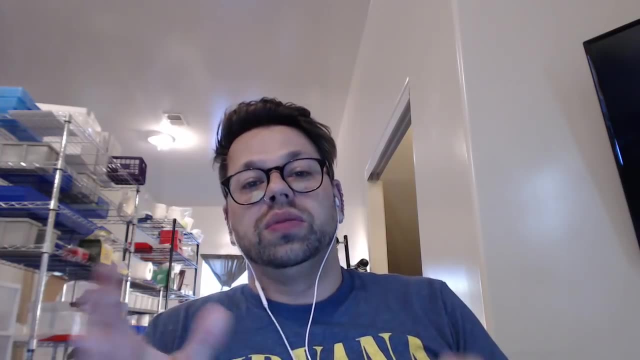 Hydrogen, Carbon, Nitrogen, Oxygen And phosphorus. There's some other stuff Like sulfur And things thrown in there, But generally These Five Atoms Make up The large majority Of things In cells. 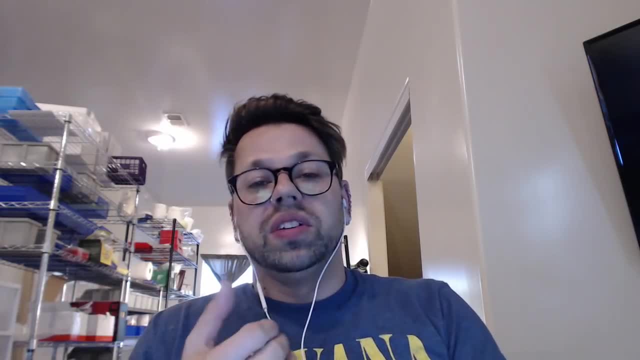 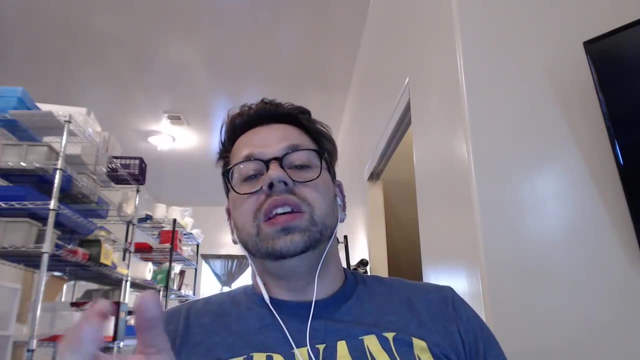 So If you want to grow cells Of any type, Whether it's yeast Or bacteria, Or plants Or human cells, Basically, If you provide them With These Five things, There's a good chance They're going to grow. 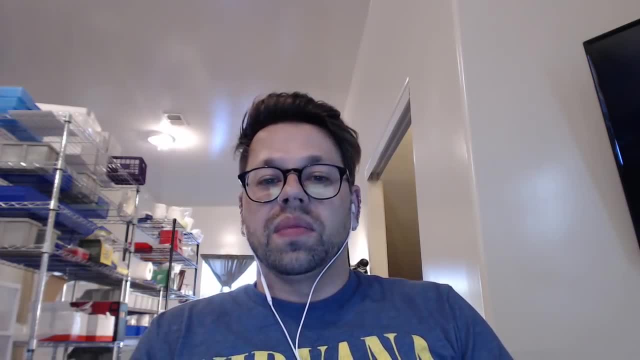 Or You know, At least Survive In some way. So When you're growing your cells, When you're growing things On agar plates, When you're growing things In media Or whatever, Understand that these medias. 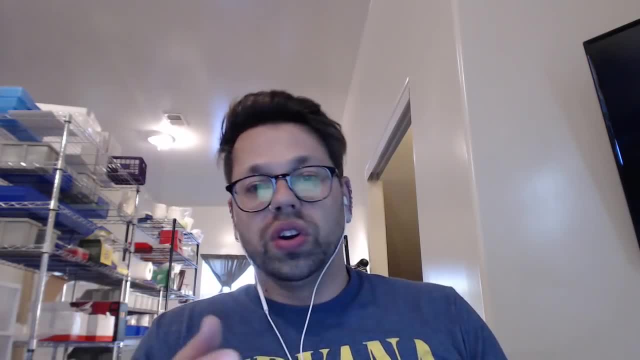 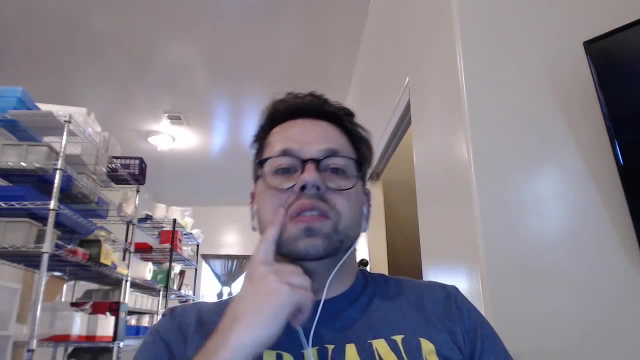 Basically, That's all it is. You're feeding these Organisms Sugar And some phosphorus And some nitrogen, And That's pretty much it, Right. So The main component Of a lot Of these medias. 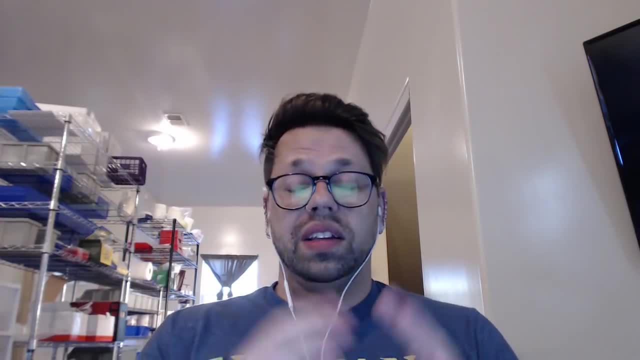 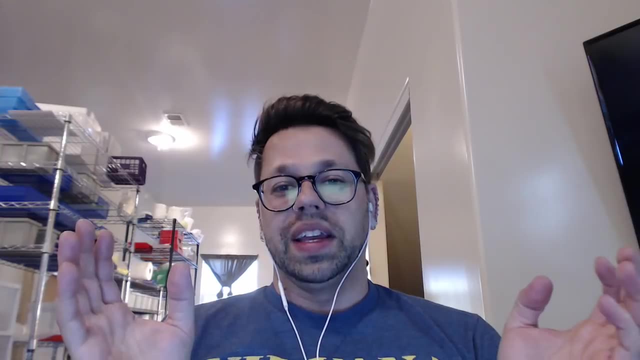 Is things like Yeast extract, And yeast extract Is exactly Like it sounds, Is basically Just some yeast- That Everything has been Extracted from them And Provided to you So that you can You know. 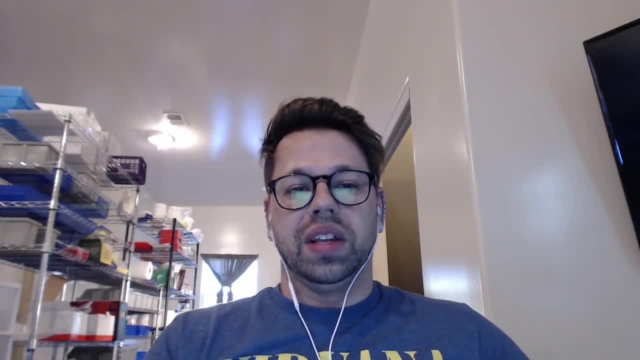 You can use All the The good parts Of the yeast That kept them alive For your organism. Right, Alright, Alright, Okay. So Everybody Following along, Everybody get this. Everybody have an idea What's going on. 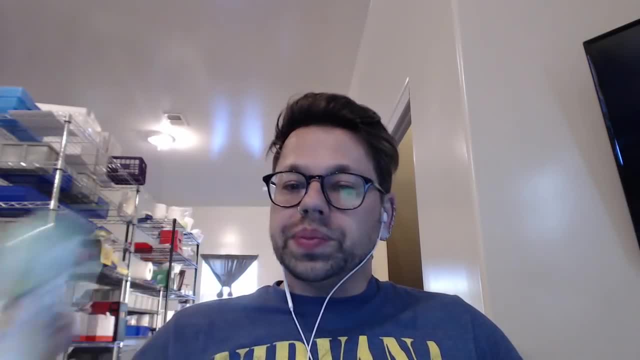 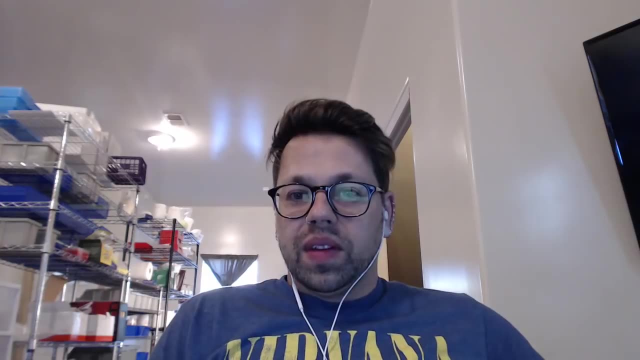 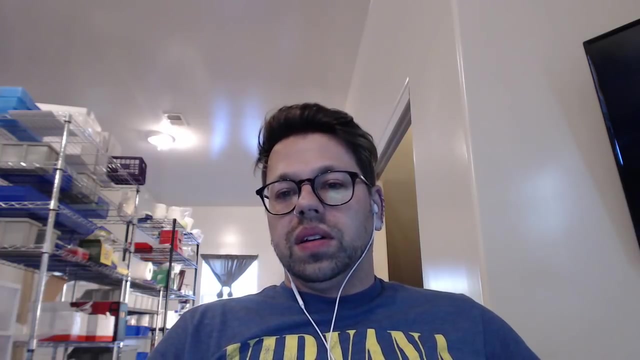 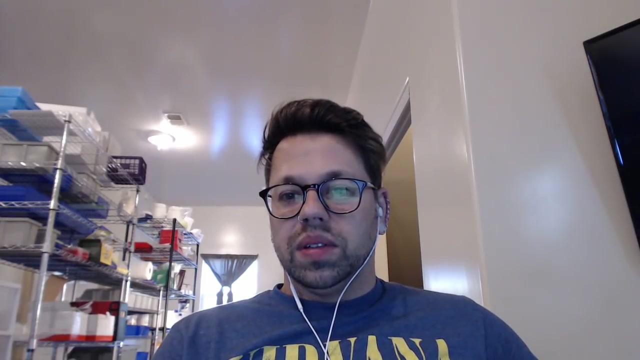 Pretty good. No, Ted, You have no idea What's going on. We're talking about planks. Oh, Don't worry about that. Yeah, I mean, I mean Questions, Questions, Jill, Don't, Don't. 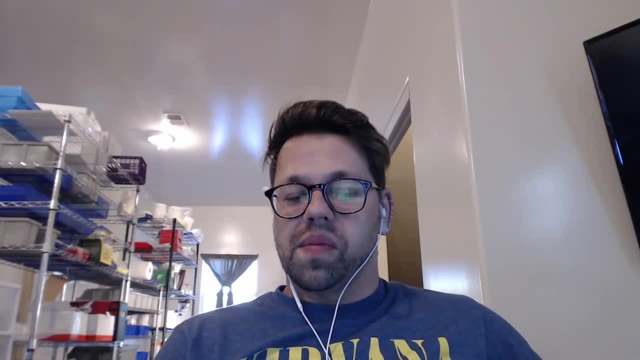 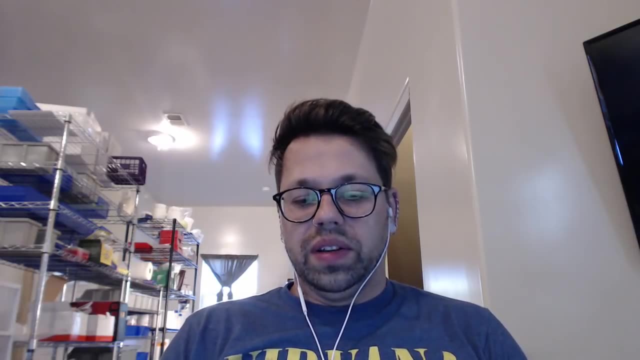 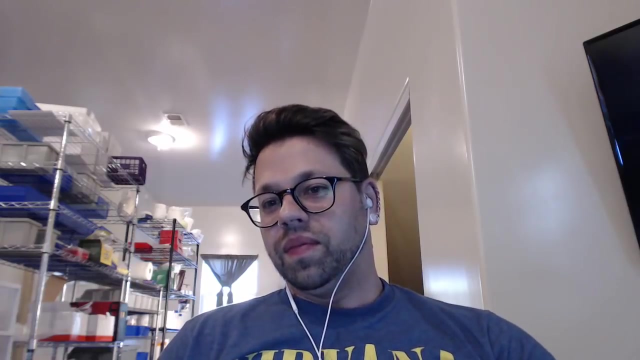 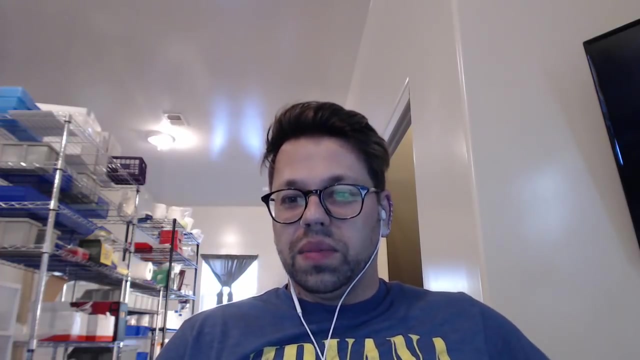 There's link to info. I'm making my own Gene gun. Come on, What do you got? What do you got Somebody? Somebody's got a question. How's my myostatin going? It's not something I'm working on. 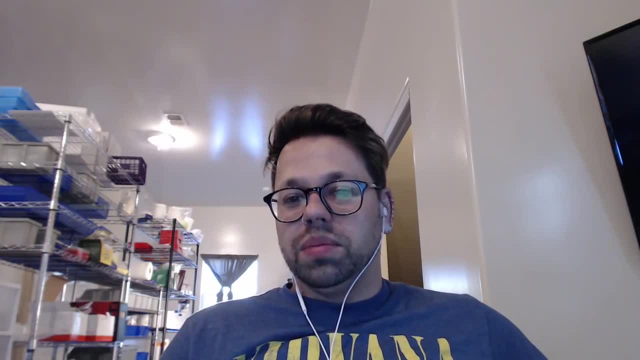 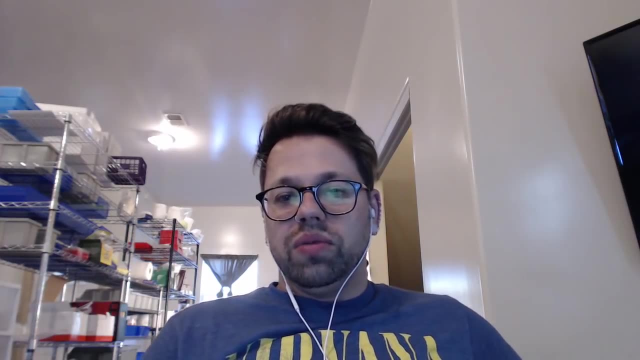 It's not something I'm trying to get. I don't really inject myself with stuff anymore. Sorry, Ted, I hope I didn't disappoint you. Brandon, You could find a copy of this live stream right here on YouTube If you click on the Odin. 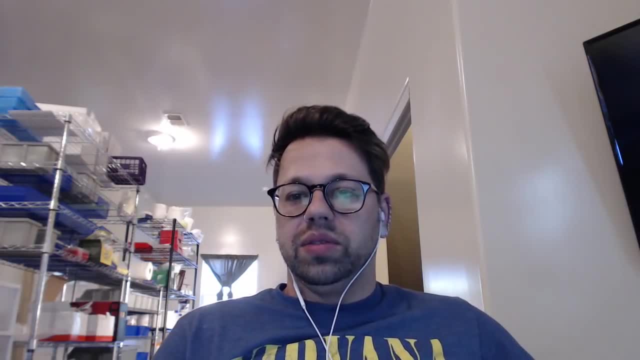 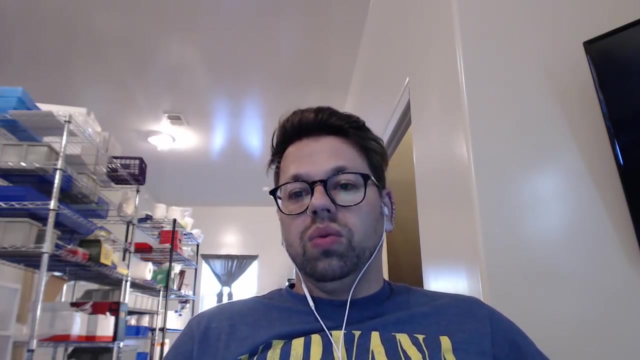 Go to the channel. There should be a playlist that has this live stream. Yes, Trey, That's a good question. Our proteins, What determined the cell specific function? Exactly Right? So the different proteins in the cell will determine how specifically that cell function. 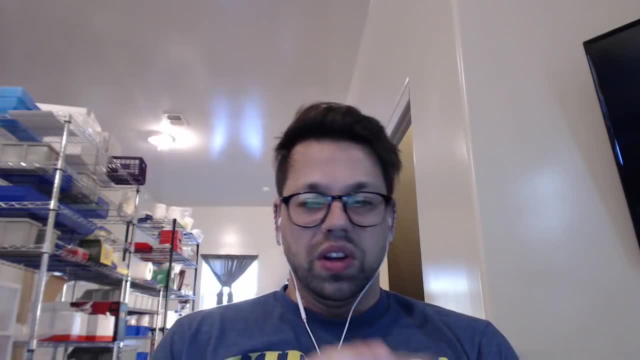 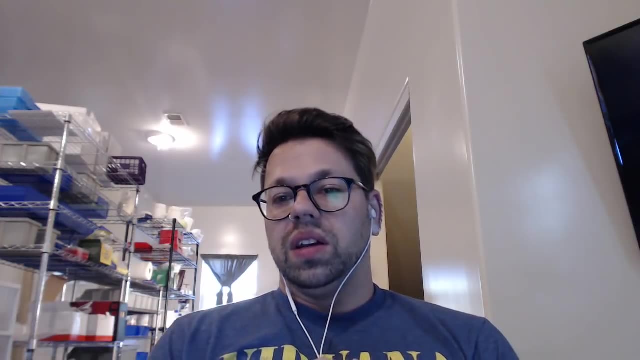 So if you start- Let's say we start with like a stem cell, You know Totipotent stem cell- in an embryo, That can become Anything Right. Then what happens is, as the cell gets subjected to other proteins or molecules, it starts to differentiate and this differentiation causes different amount of proteins to be in the membrane in the cytoplasm. 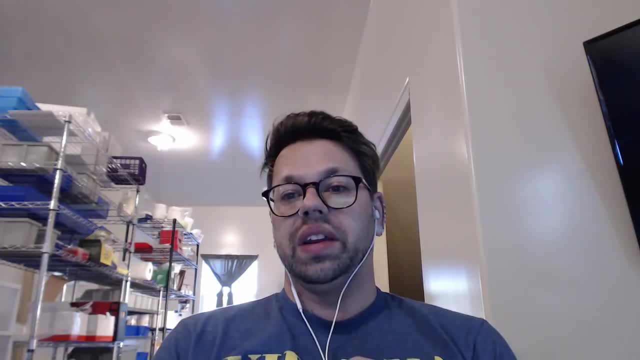 It causes the shape of the cell to start to differentiate And basically the proteins, All, All, All cells generally will have the same genes, but the proteins inside the cell and the proteins that are regulating those genes will determine the cell specific function. 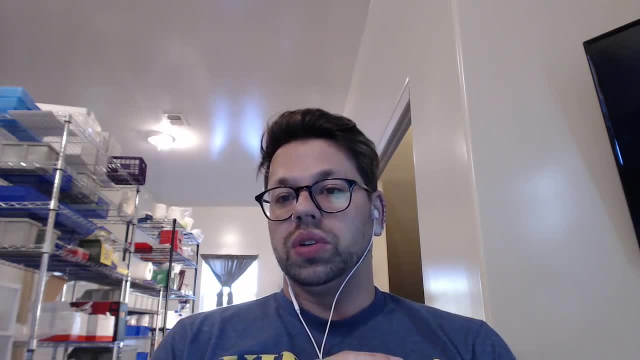 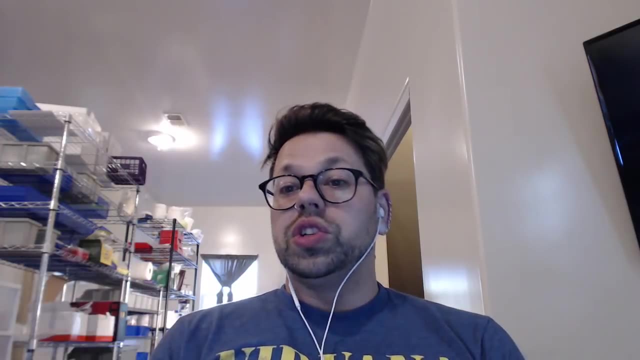 HP Waller. How do papers on model organisms pass through? if they're bullshit, Who are they convincing? Well, so you have to understand that when people are just publishing something, they're just publishing a paper, Right, So generally they're not making grandiose claims. 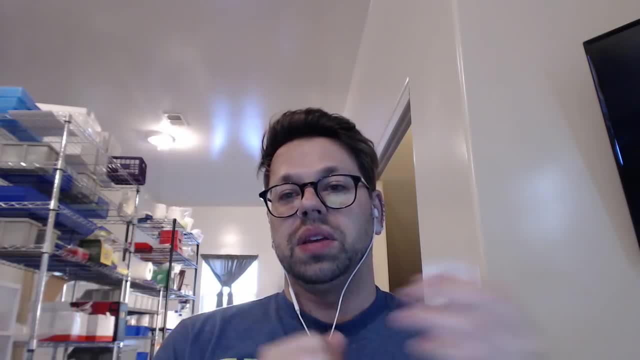 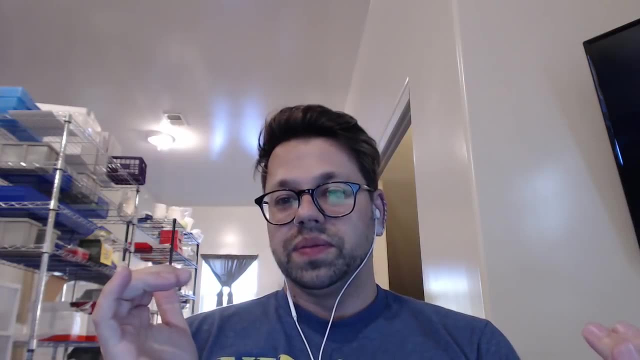 It's usually when the media gets Ahold of it and they they see this paper that they like cured cancer. I mean like they've cured cancer in mice at least 10,000 times. right, They've cured every type of cancer in mice. 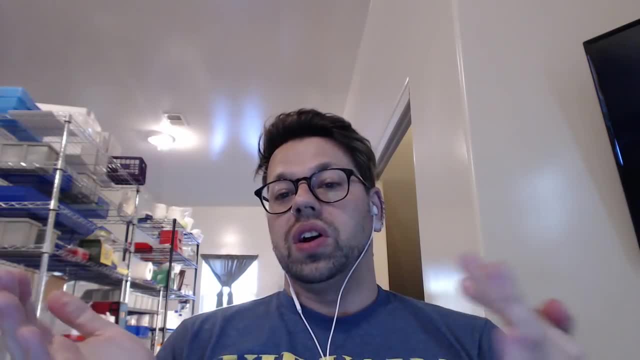 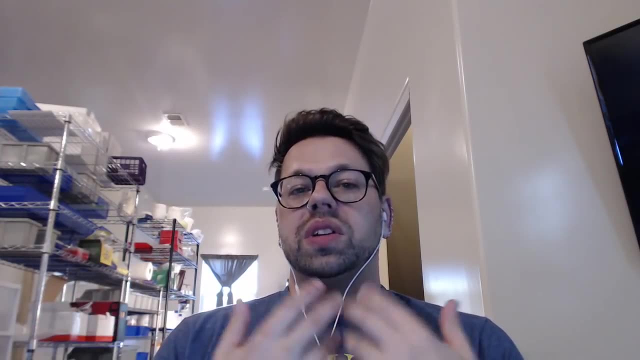 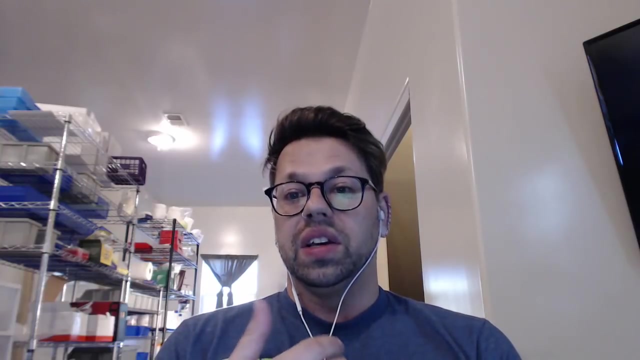 So it's not necessarily that the papers are bullshit. It's that the way they're portrayed is bullshit, right? It's when scientists look at the paper Generally- you- they look at it with with skepticism. They understand. They understand the mechanism and the function behind this. 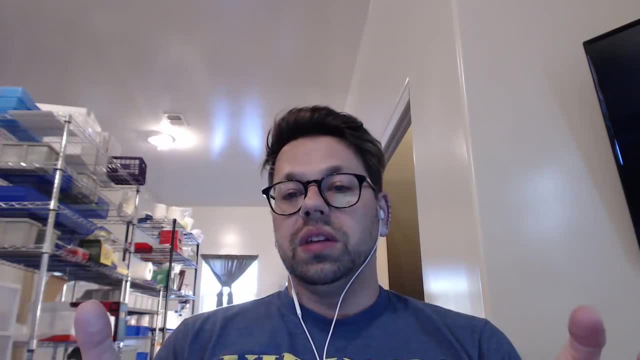 But They they understand the limits of it. A lot of people don't understand the limits of how How a mice relates to a human or how a fruit fly relates to a human. They think that these things can just be interchanged. but they really can't. 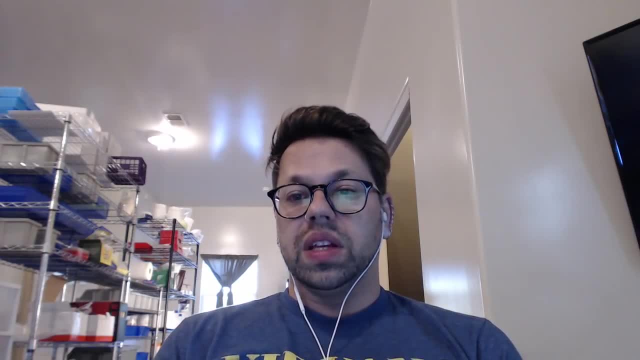 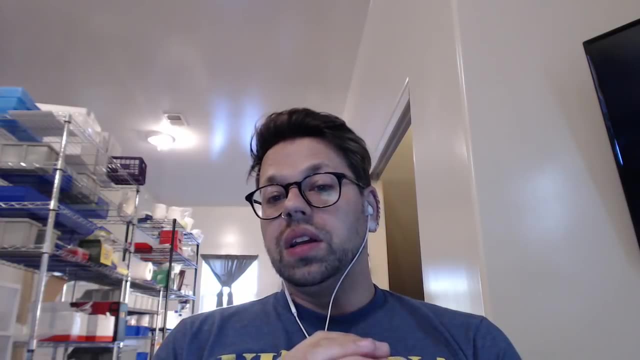 Right, Mr Metric, In this class. and what do you teach? enough info to make bacteria manufacture custom proteins- something other than GFP? I mean, you can use the knowledge from this class to make bacteria make custom proteins, but we don't go through exactly how to do that right? 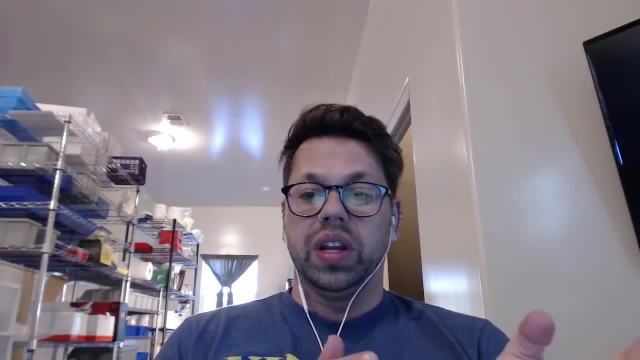 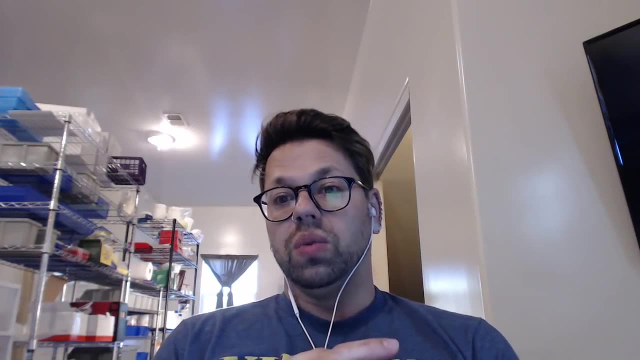 Like all you have to do is take a plasmid you want and put it in bacteria or yeast the same way you learned in the class. We don't teach you how to manufacture that custom plasma, No, In the 102 class it's way more in depth and it requires other equipment like centrifuge and things like that. 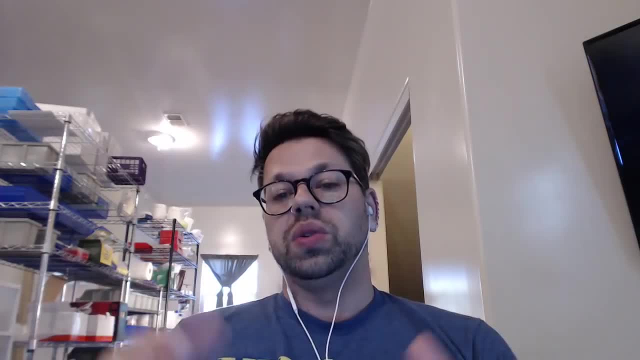 So in the 102 class we go over that stuff, But in 101, we're just teaching you how to, how all of all this works, Right, So how to actually genetically modify the organisms like that. There's plenty of information. you'll learn that in this class that putting in more is will be overkill. 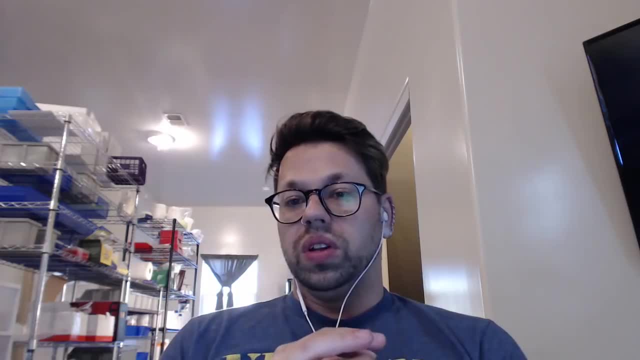 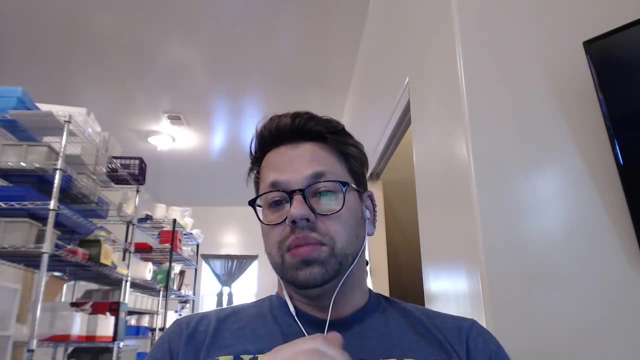 Does epigenetics play a role in the expression of genes? Ted, yes, it does. What way, how and what? That's complicated and not exactly understood. But some people say certain epigenetic things silence genes. but not all genes that have different epigenetic markers are silenced or have different expression levels. 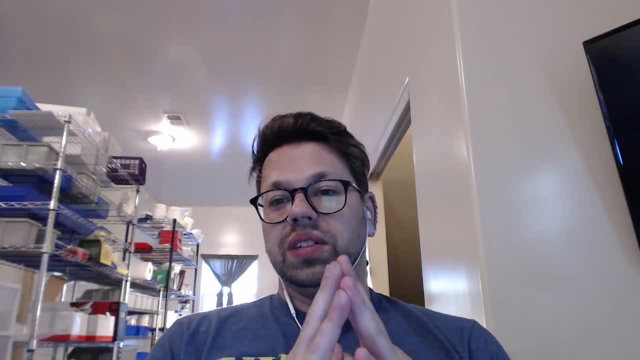 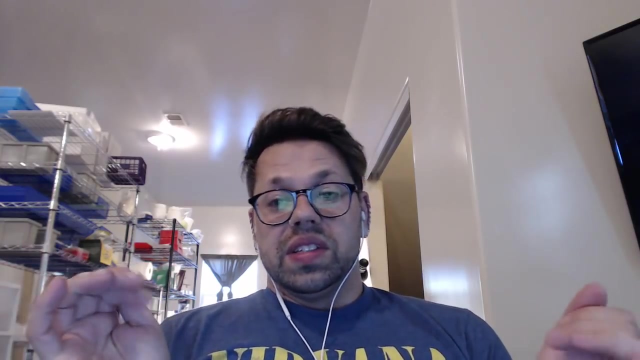 It's complicated. It's complicated. Epigenetics is kind of still It's still magic. How does one cell become a toenail and the cell right next to it become flesh? Oh, so this Dixon's is like cell. This is developmental biology. 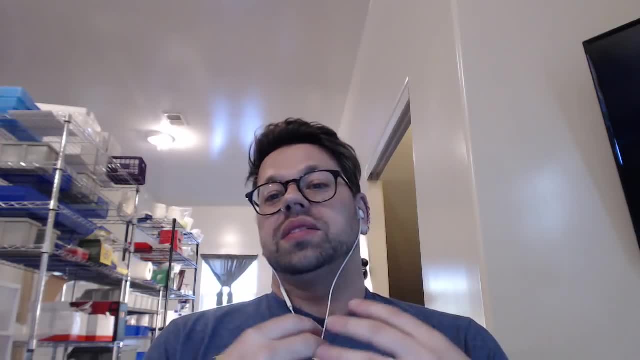 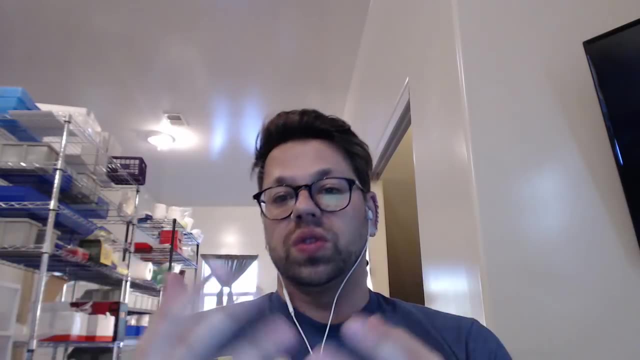 It gets into And basically it's this complex symphony, I guess, so to speak, of cells in proximity to each other interacting with each other and secreting certain molecules, And basically it's just this complex symphony. you know, there's a bunch of molecules and factors that tell each other what to become right. 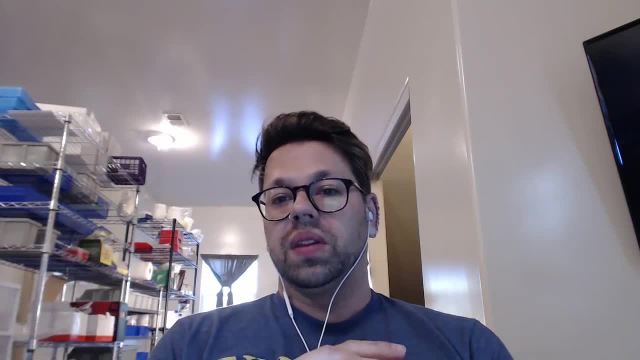 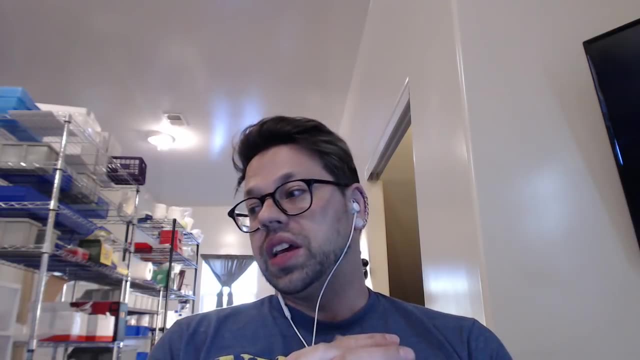 And basically it's just this complex symphony. you know there's a bunch of molecules and factors that tell each other what to become right. So you can imagine if, say, you were a tile on the floor and you had instructions that said: if three, how many are there? 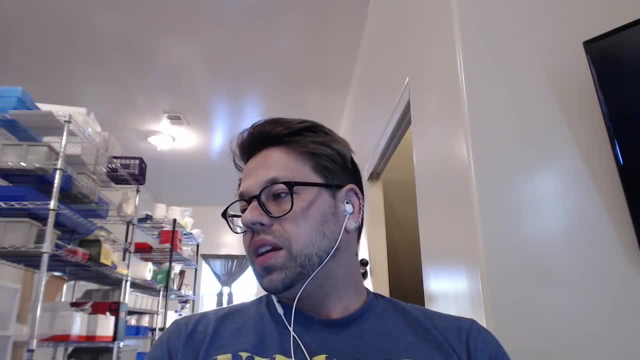 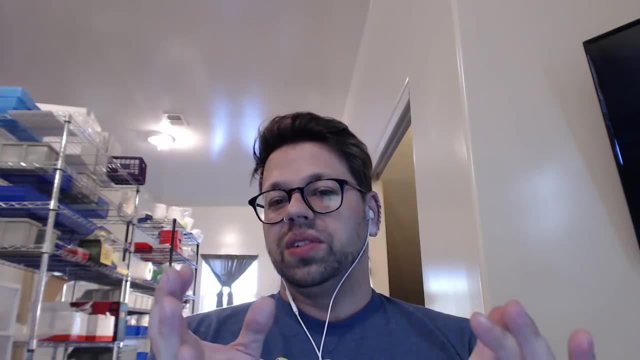 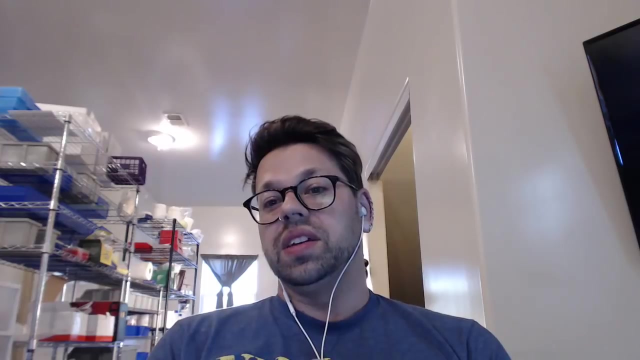 There's one, two, three, four, five, six, seven, eight, eight. So if you have a three by three grid of of tiles and you're the one in the center, if you have, say, five of the other tiles that are a certain cell type, it says, well, you know, you should become. 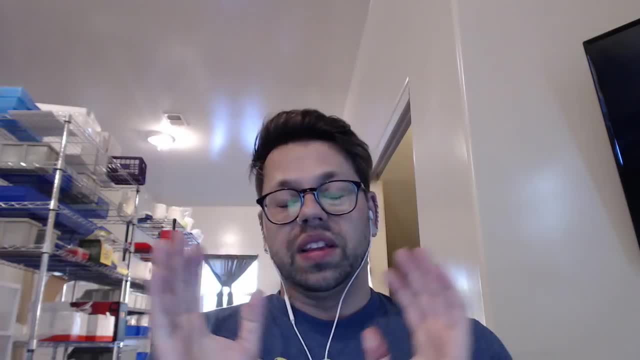 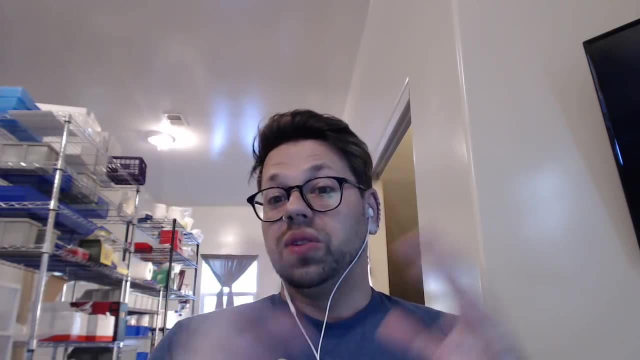 that cell type right, something like that. that's not exactly how it happens. obviously it's more complicated. that depends on the tissue and all these other things, and i don't even know how every tissue becomes everything. but if you want to look up developmental biology and look up the way these 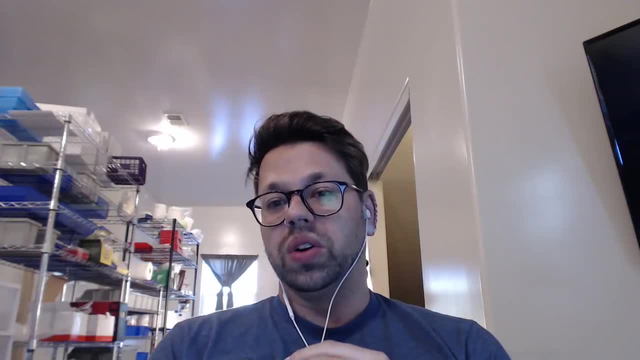 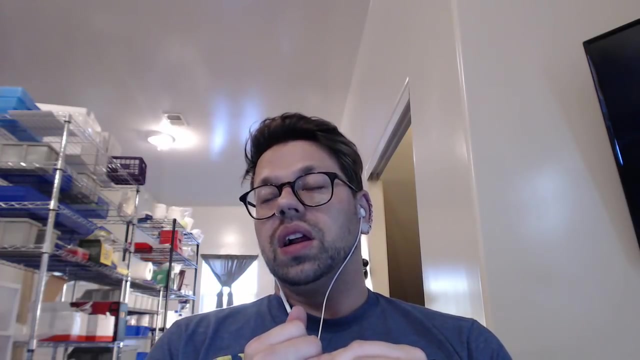 things go. they have it pretty well mapped out in some model organisms like drosophila and c elegans. is there a better way to go than animal models and strip trying something in humans? um, not necessarily, but i think we right now um fail to use larger mammals. 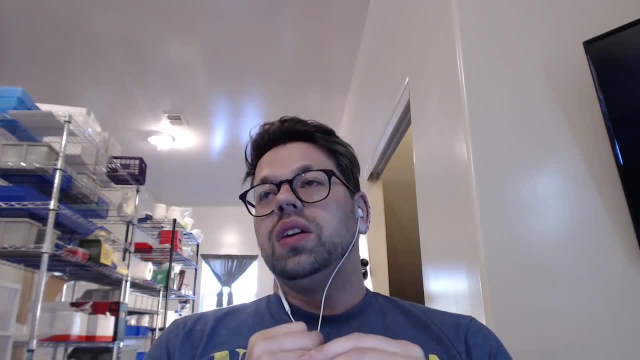 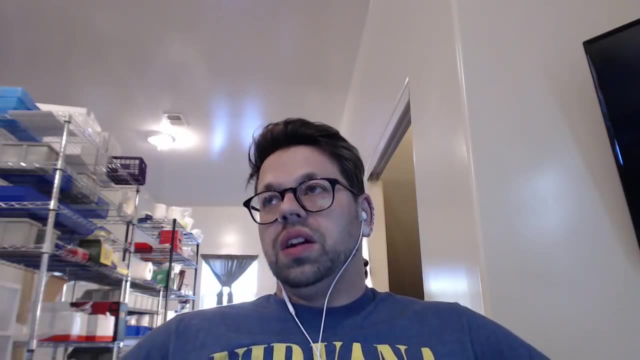 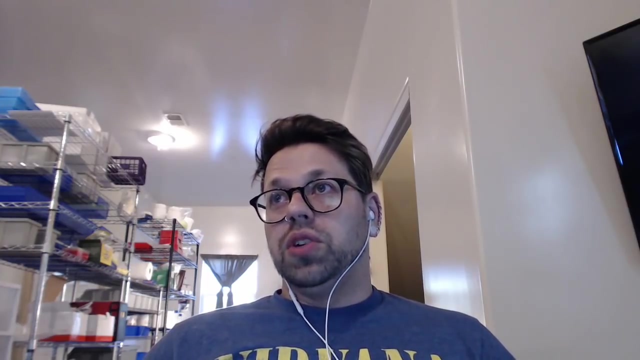 you know, we, we should, we should be using more larger mammals in our research or animals that are more close to humans. the thing is that things start to get really into ethics and ethical and expensive and what it costs to keep these animals and work with these animals and use these animals. so science is this? um fancy dance between how much money. 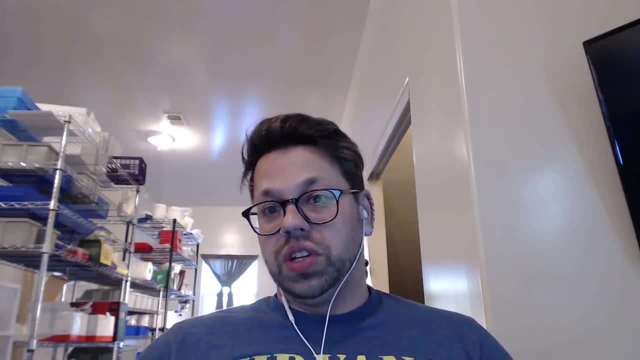 you want to spend, how much we know about that particular organism and how much effort you want to put in right. so if you're using a large mammal, say like a dog or a pig or a horse or a goat or something like that, uh, generally there's a lot less information than you'd find in, say, mice. 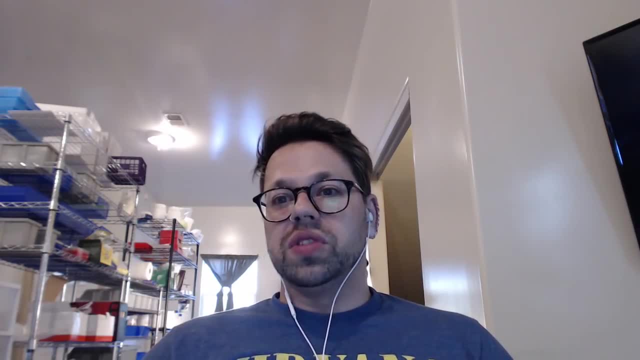 right. so what that does is it forces people to, you know, repeat the cycle and constantly use mice, because mice is where all the information is um. so you know, ted, there's not much difference between metabolic pathway editing and gene editing. metabolic pathway editing is just a, a fancy phrase people use to try to, you know, get more money for. 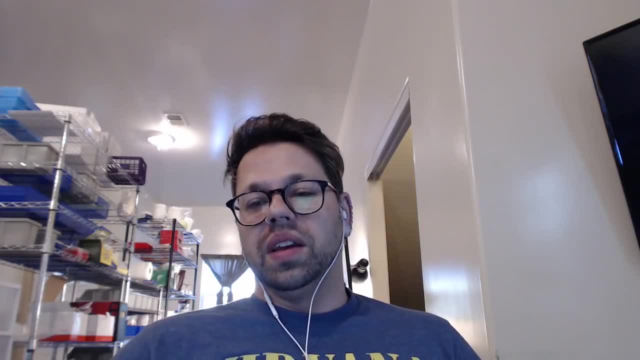 their companies. but all this metabolic pathway editing is is say, putting in more than one gene that would function together synergistically to make something happen inside a cell. right, so it's, it's. it's generally not any more or less complicated. now, if you want to devise novel metabolic pathways, that can start to get complicated, or if you want to take 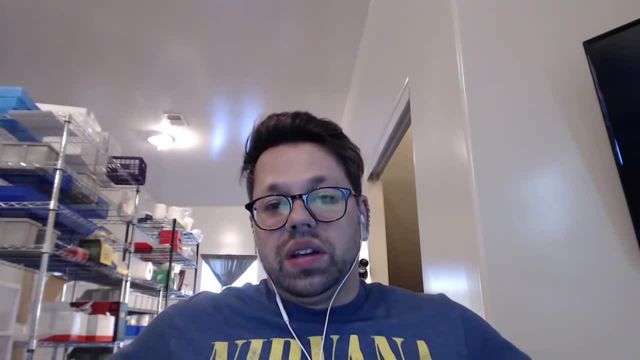 a pathogen that's not going to be as complicated as a gene, that's going to be as complicated as a cell, or a cell that's going to be as complicated as a gene, that's going to be as complicated as a cell pathway from another organism. and you know, make say, thc and bacteria or something that could be a. 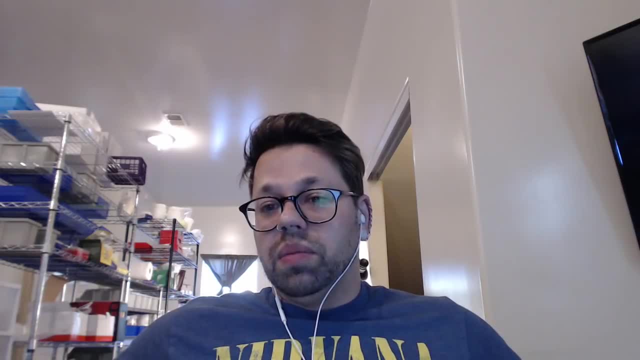 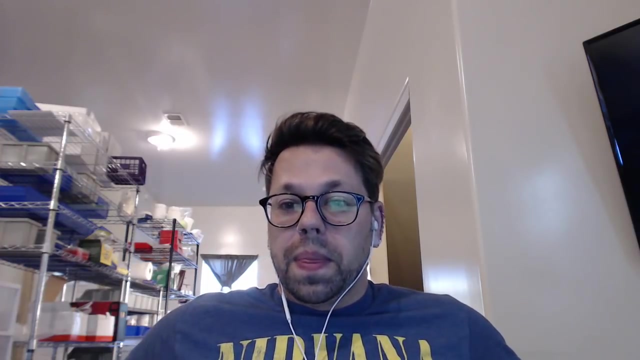 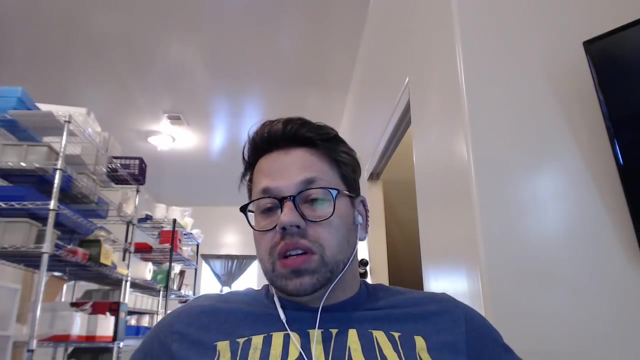 little complicated, but generally metabolic. uh, metabolic pathways, you know, they can be pretty straightforward or as complicated as you want, depending on how complex you're trying to do. yeah, uh, sebastian, it really depends what type of cell you're trying to work with and, uh, what type of you know thing. 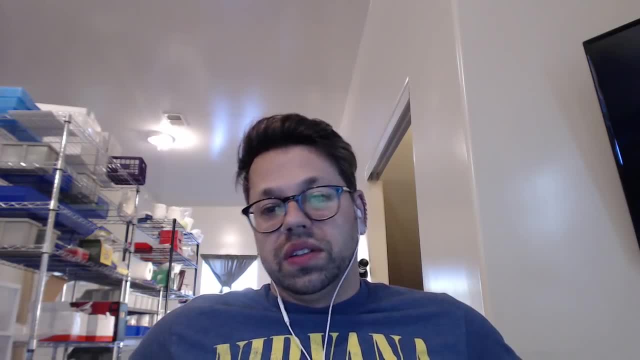 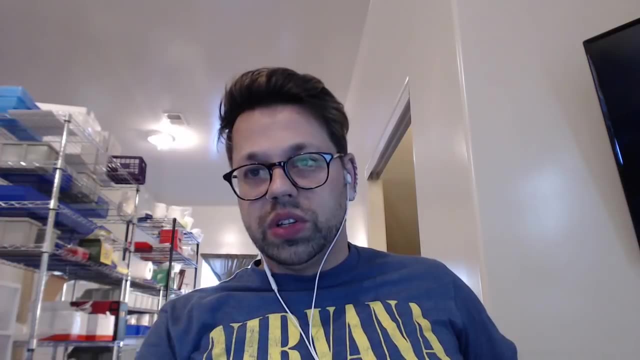 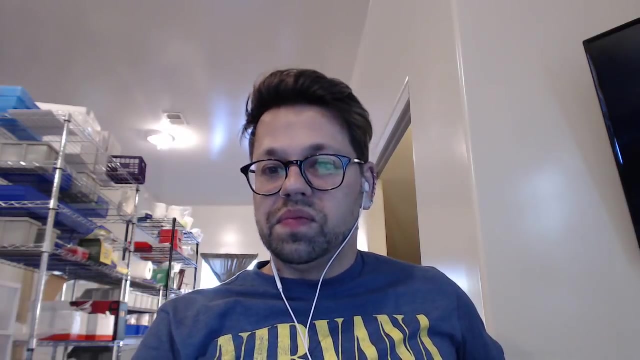 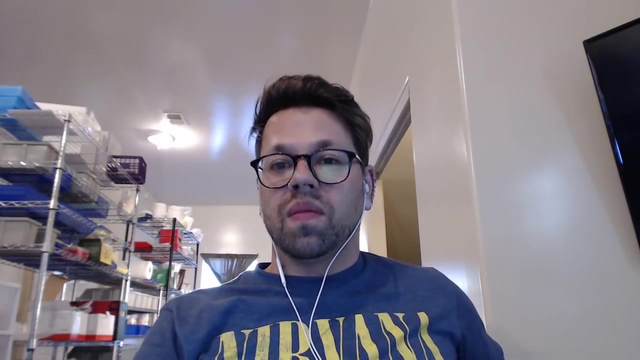 you're trying to get it moved towards. there are plenty of cells that move towards things, a lot of cells. i think one of the papers we might have in here is like using genetic engineering to cause human cells to move towards light, which is pretty cool. all right, any other questions before jill? i don't know why i have these headphones on, because 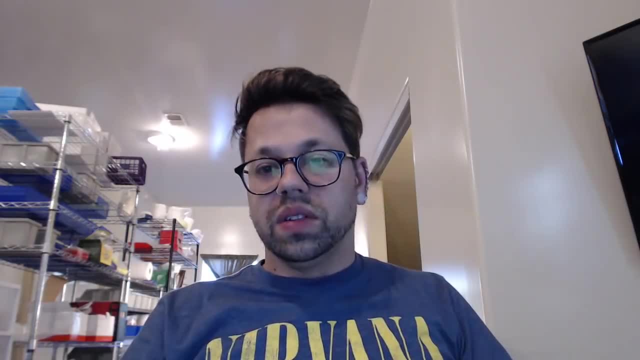 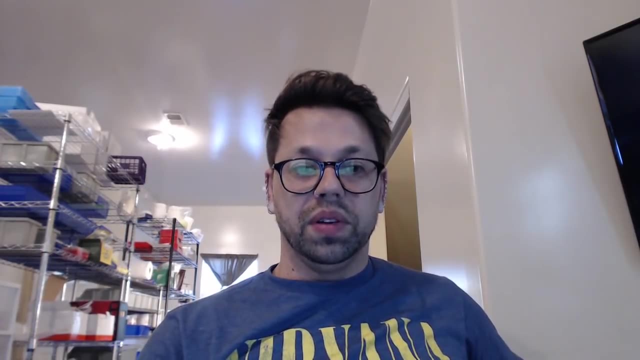 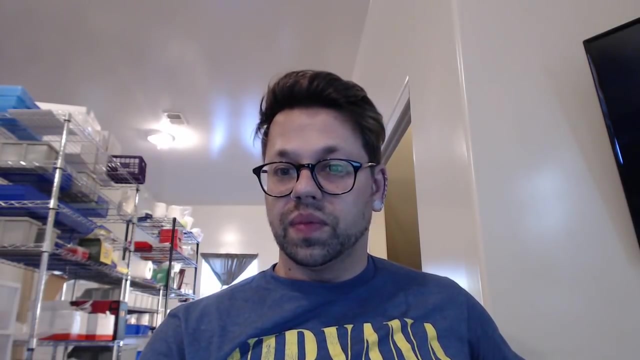 there's like absolutely no sound. i guess you all could probably hear me even without the headphones, right, can? can everybody hear me? can people hear me jill can you? yeah, looks like the mic's working. you can hear me. the transportation of cc9 or cc13. is there better vectors or virus? 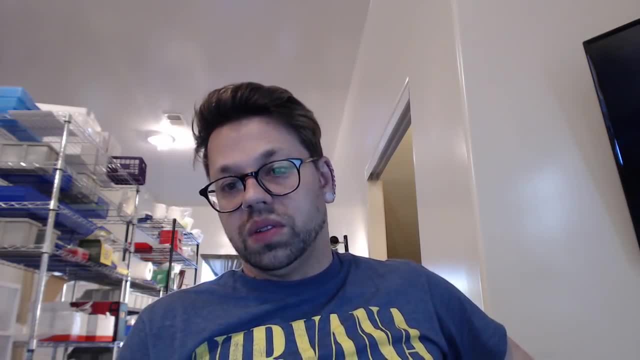 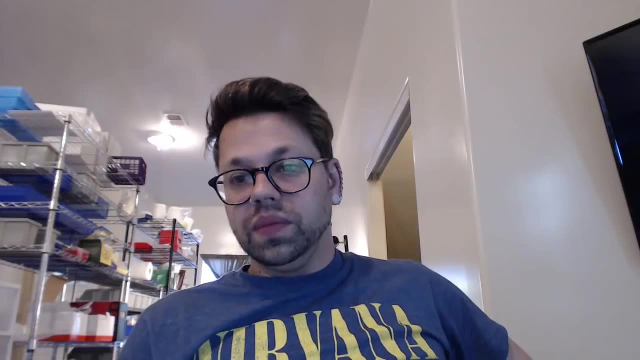 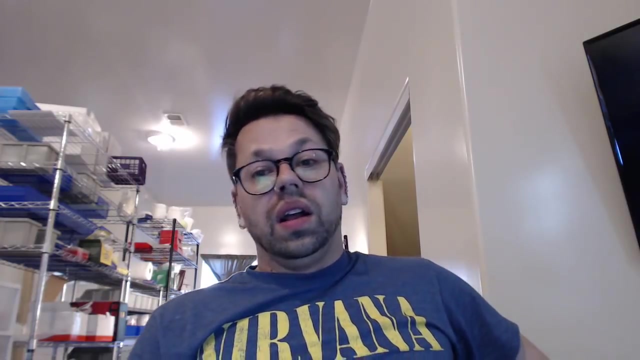 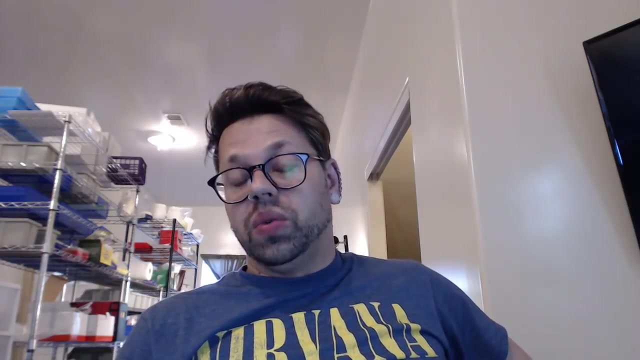 is example: using a respiratory virus versus h1 to reach particular cells, cellular dna types. what do i prefer, genetic engineering or protein engineering? okay, so, brandon, that i don't know anything about cc9 or cc13, so i'm not going to be able to tell you what the 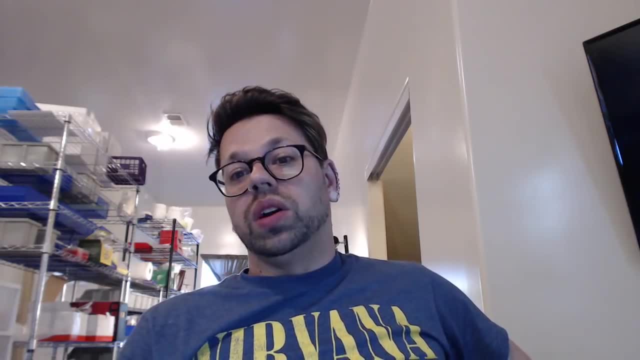 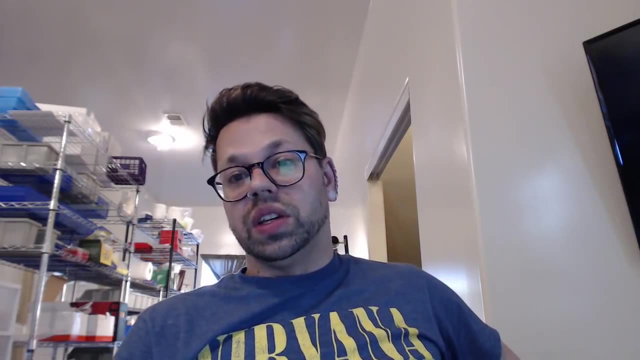 best vector is, and that depends on a lot, right? it depends on where it's trying to be transported, to what kind of protein. it is what it's doing. there's a lot of different things. so generally you don't want to use different types of viruses, right, uh, unless you're talking about different. 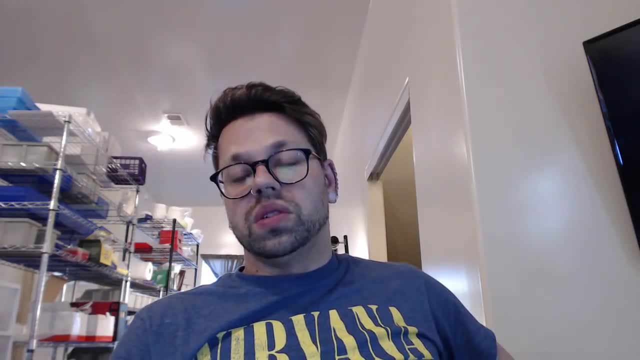 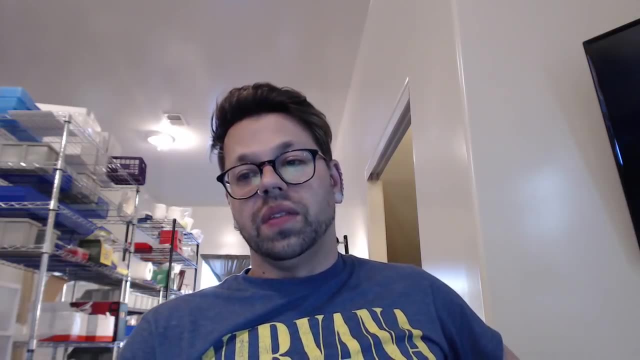 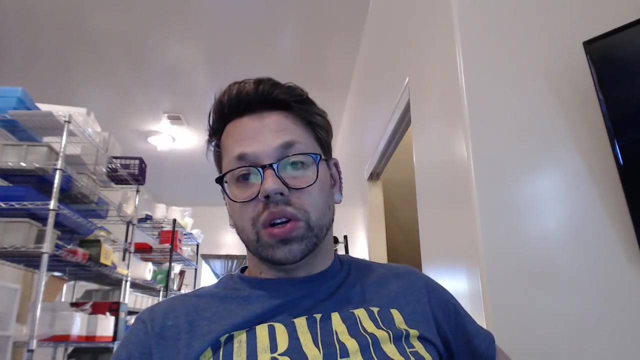 aav serotypes like you don't just want to use. you're never. no scientist is going to use a random respiratory virus to put a gene into a human body, because these viruses have so many other things in them that could do bad things generally. you want to put a virus in your body that's non-replicative- replicative, so it doesn't. 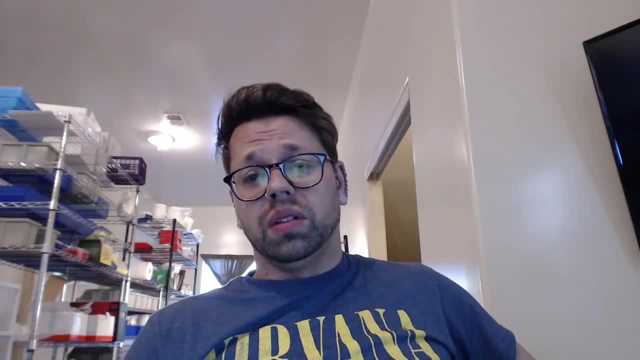 replicate, because you can imagine, if you start infecting yourself with replic replicating viruses, your immune system is going to freak out and, uh, it's probably going to cause something bad. so generally people focus on aav serotypes, adeno associated viruses, so you should look into those. 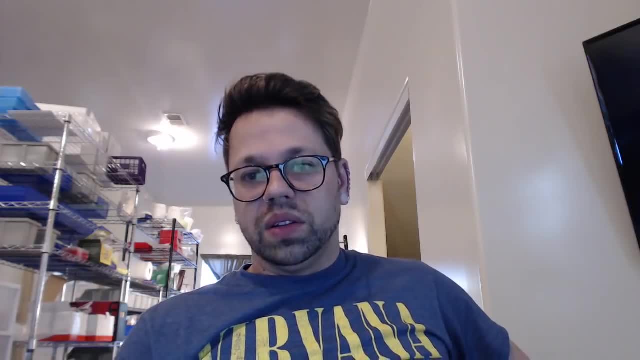 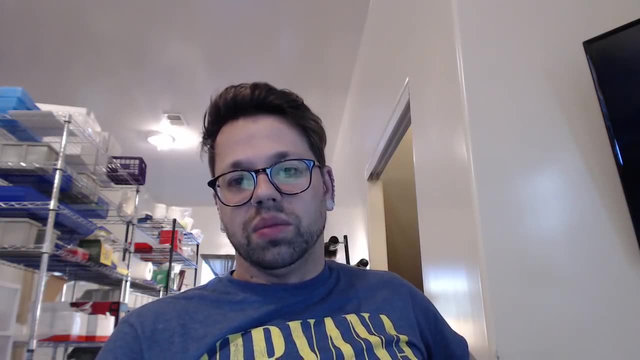 and see if people have used any of those, the sudarshan. what do i prefer, genetic engineering or protein engineering? i don't know what that means, but i think it's a good idea to look into engineering. oh, that's a tough one. protein engineering is cool, but it generally is not. 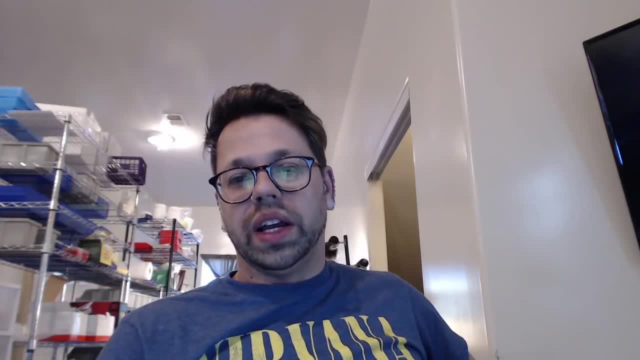 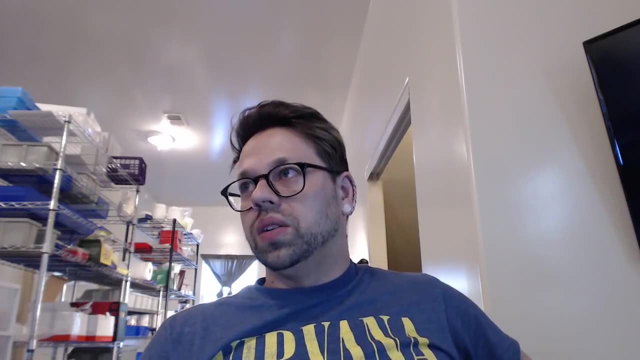 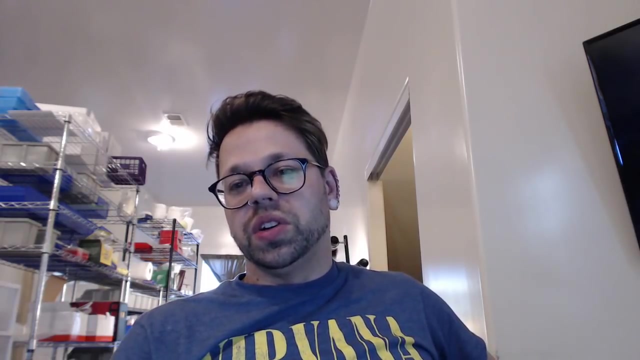 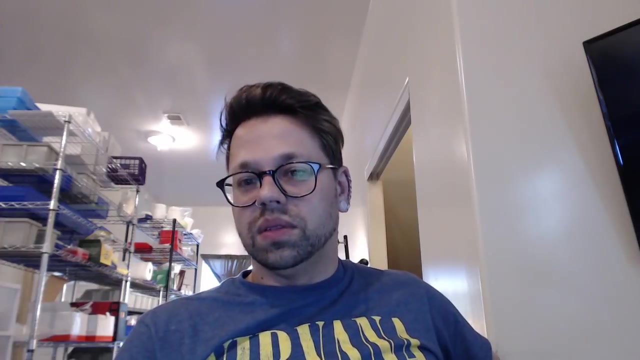 as applied as genetic engineering. genetic engineering is a lot more applied. so protein engineering is like, uh, people who like to- uh- you know, i don't know- write program code or write code or something like that, and genetic engineering is like people who like to build robots. so they both can be pretty cool, but uh, so anyway, i'm gonna go for now because jill's gonna take over. 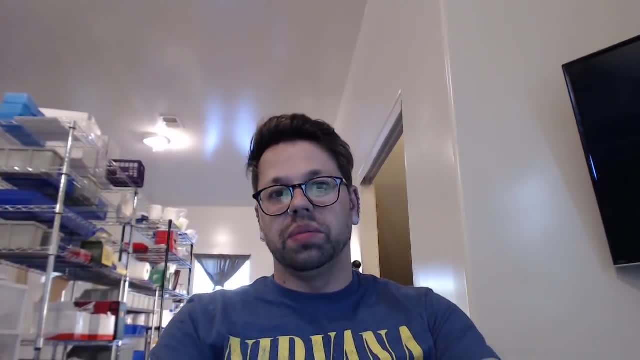 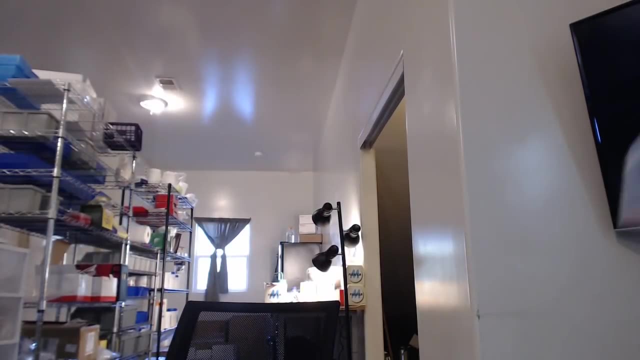 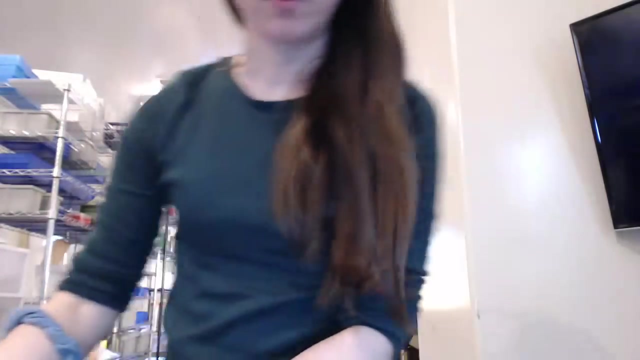 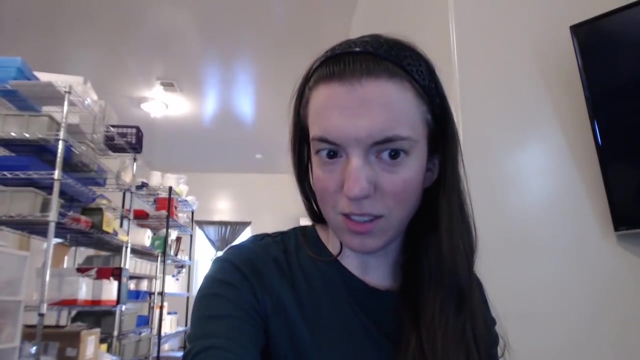 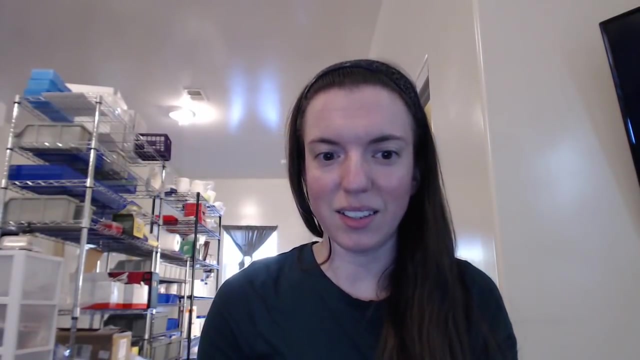 so you all be ready for jill. she's gonna show you how to do some pipetting and stuff and we're gonna switch. all right, okay is it? is it just like frozen? it's still working. oh yeah, let's just pause. okay, it doesn't get feedback and stuff. if you want to, that's so. it has the chat. if you want to like, look at the. 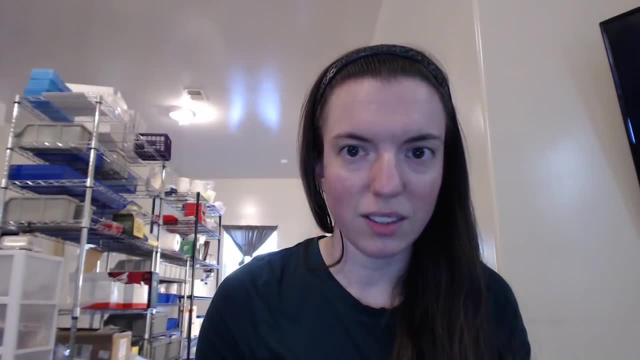 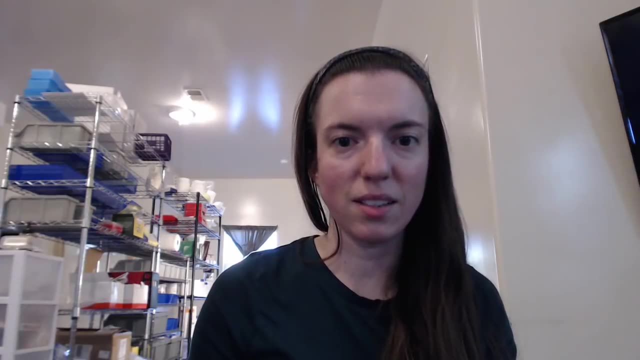 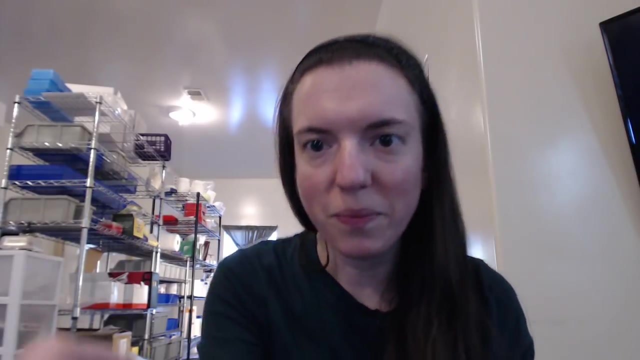 edge of the screen. oh, it's like. oh yeah, so that's, it's a little lagged. yeah, it's like 10 seconds, yeah, so making sure i'm gonna. yeah, sorry, everyone, okay, it's good, it's probably really tight, so that's good. okay, hi, peter, how's it going? 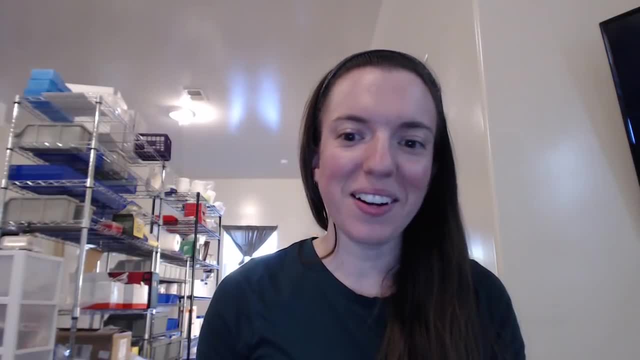 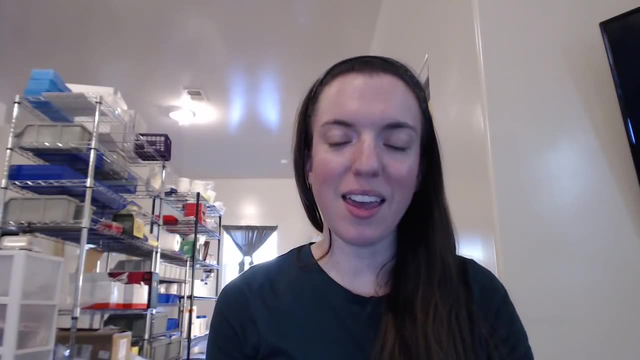 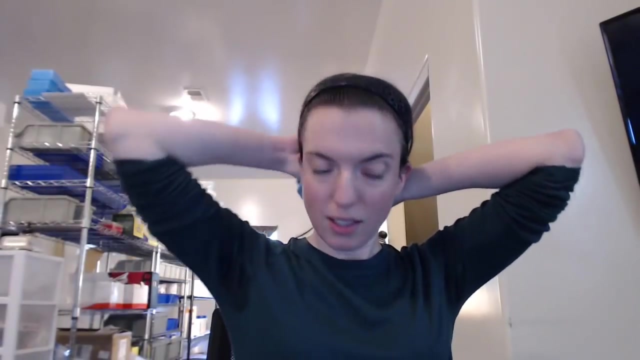 okay. so today we're going to um be going over using our scales and our pipettes, and first things first is safety. so if you have long hair, you are going to want to put it up, because hair and food is gross and hair and plasma plasmid is worse. 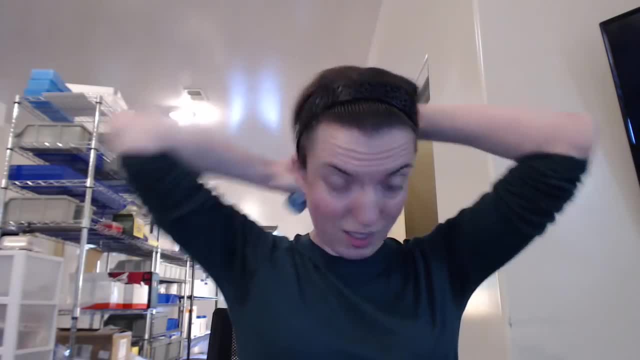 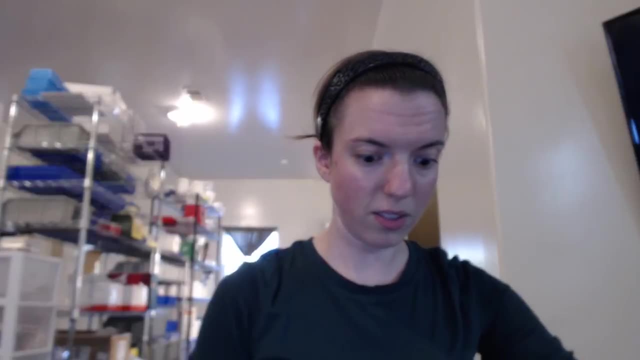 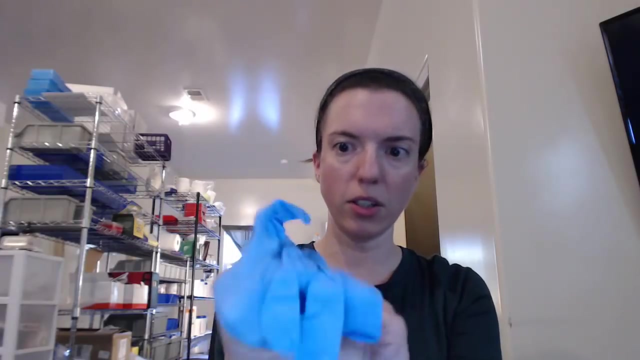 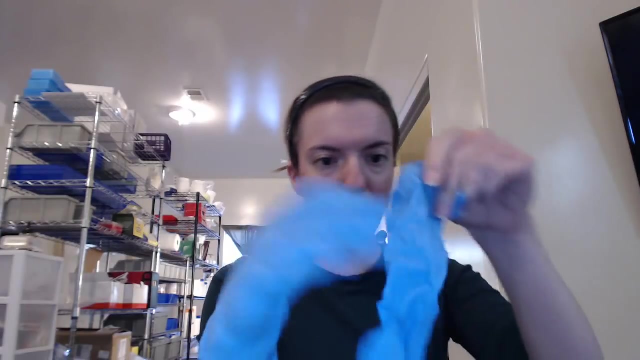 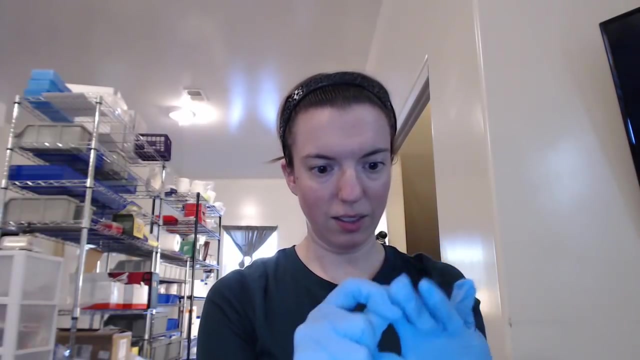 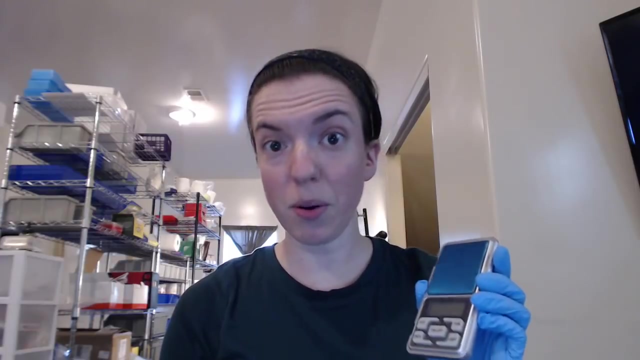 and then next, since we're doing science, we want to put on our gloves, and this will be pretty good for everything you're going to do. you don't really need eye protection or a mask, but gloves are great, okay. so either you already have or you are going to get a scale very much looking like this one. 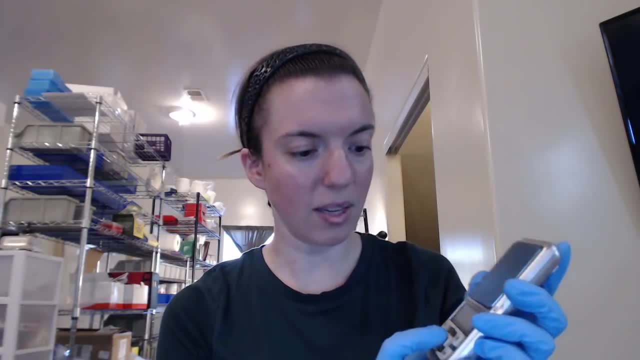 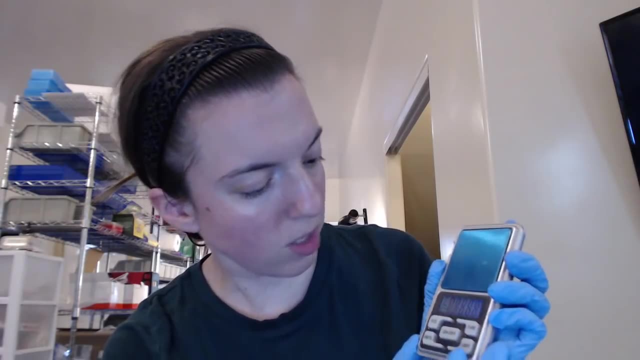 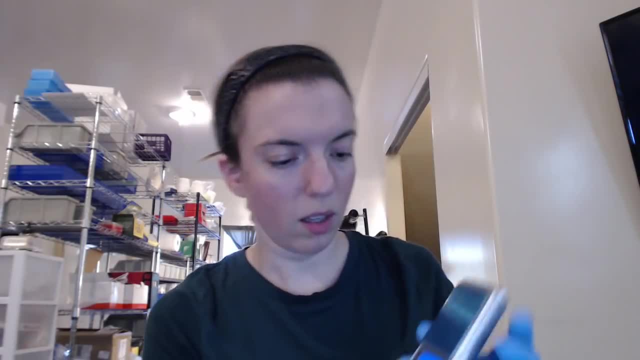 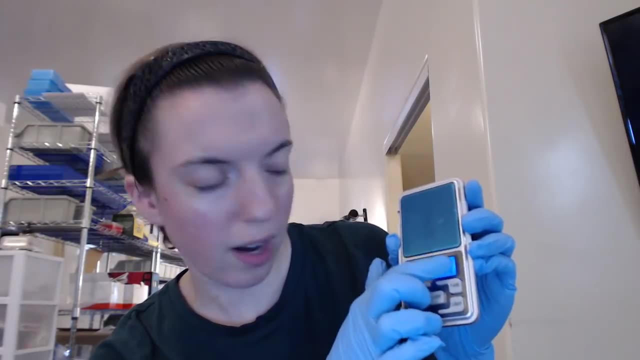 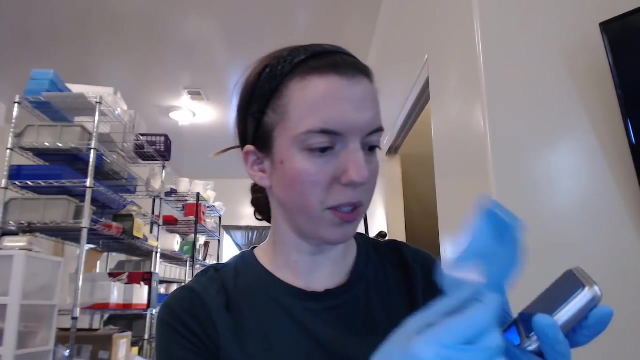 doesn't like it because i'm holding it up and right now it's going crazy because i'm messing with it, but we have different units. make sure it's on grams up top and then, basically, what you're going to do is you're going to put your- this is all going to be- on a nice, stable table you're going to put on. 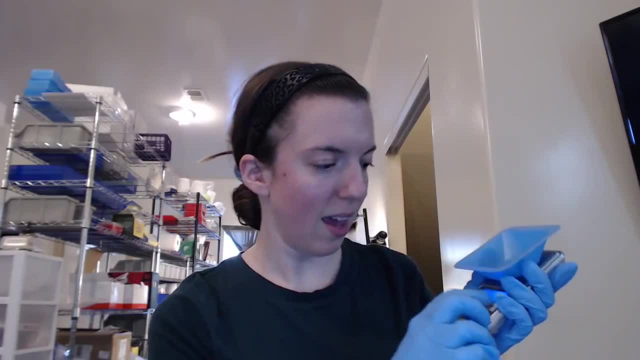 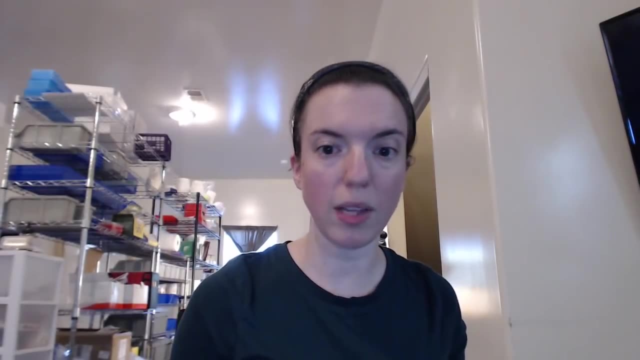 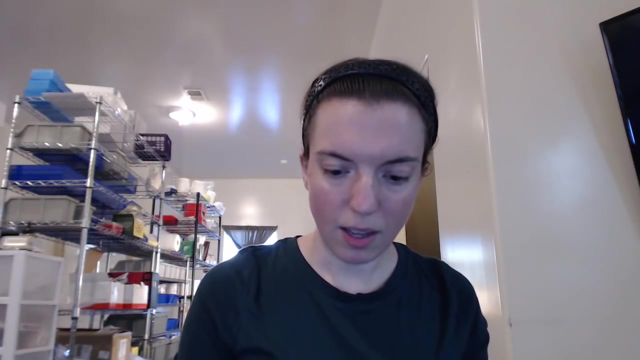 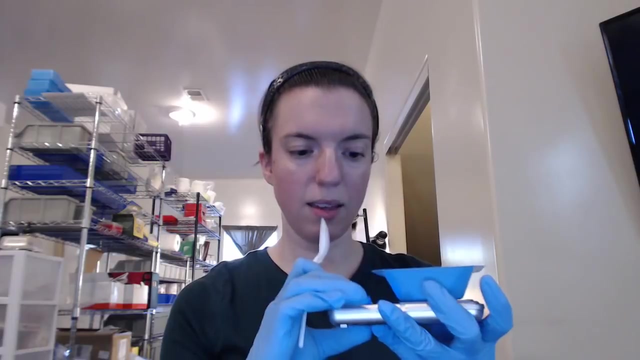 your um, your way boats and tear it. and when you do it on a table, when you press the tear button, it makes it zero, so that you don't have to subtract the way boat mass from whatever you're weighing out, and so it'll be like. it'll be like that, and when you press tear it'll be zero, and then you just 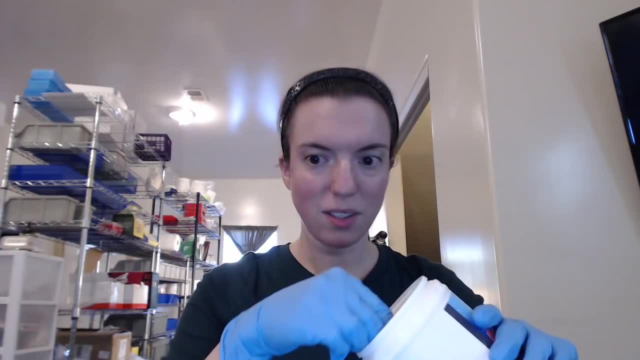 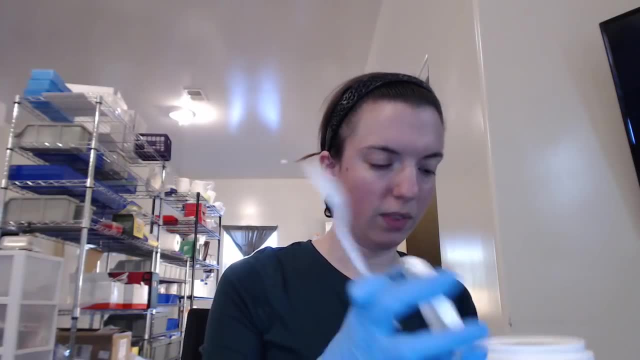 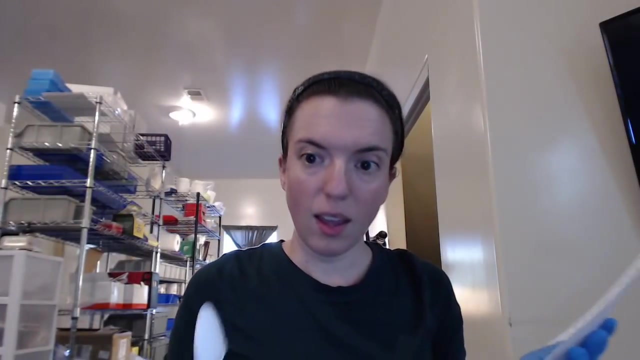 get whatever you're measuring out. we gave you guys spoons so that you can weigh out the proper amounts and, oops, left my notes over here, and so that's pretty straightforward. um, one note is that you want to kind of center as much as possible everything you're weighing for. 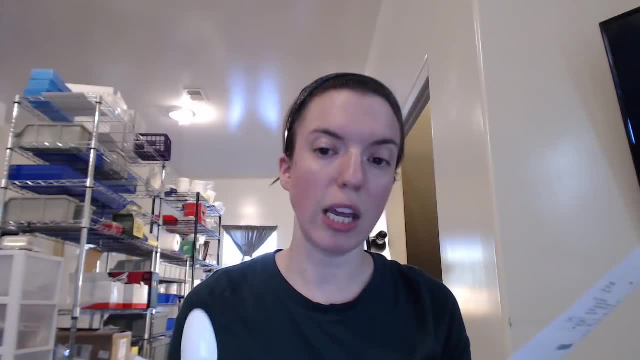 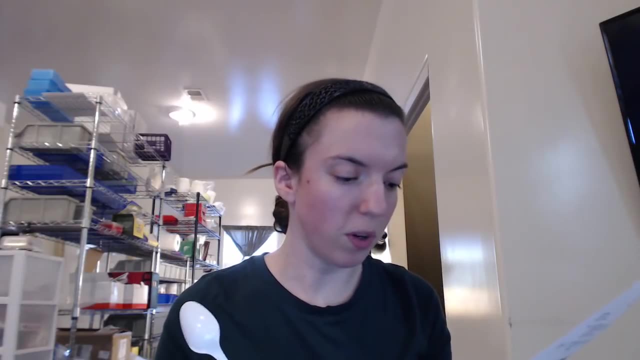 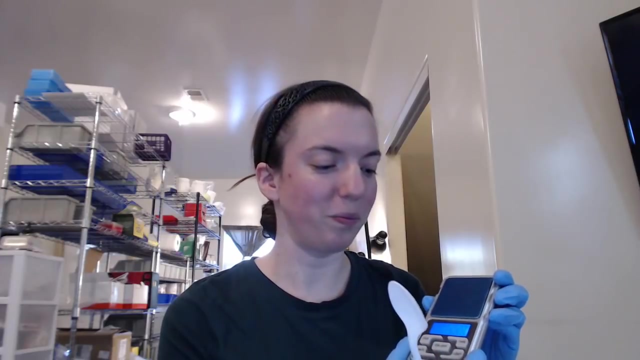 better accuracy. uh, you want to bench your table that's as stable as possible, so heavier is better. um, if at all possible, you want your work area free of vibrations or drafts, because that will also mess up um your measurements. and then, um, ours broke off, but you all have a nice little um cover for your scales. 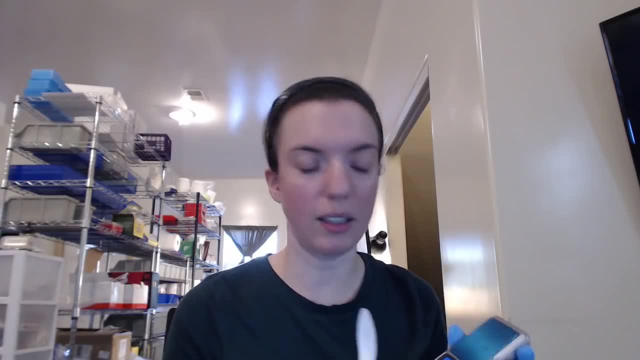 and so, when you're done, you just want to clean off any um of the um powders that you're weighing. if it fell, that's okay, you just want to clean it off your table. let's go ahead and buff that straight and then come to the next page, which is measuring the solved. 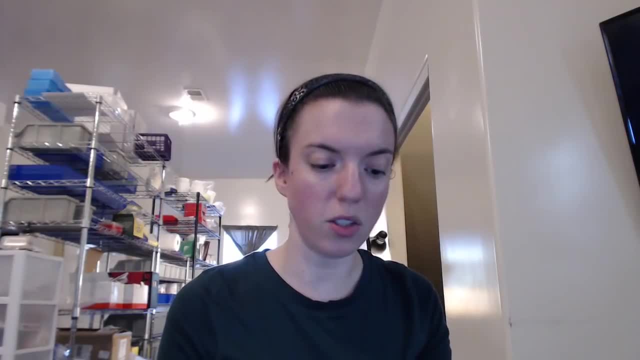 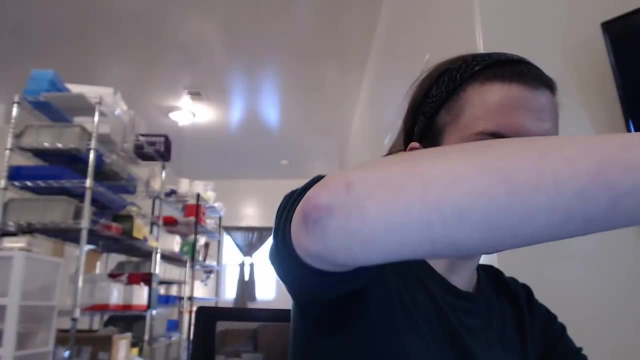 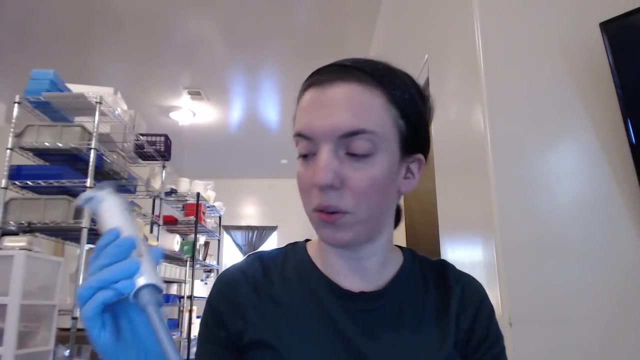 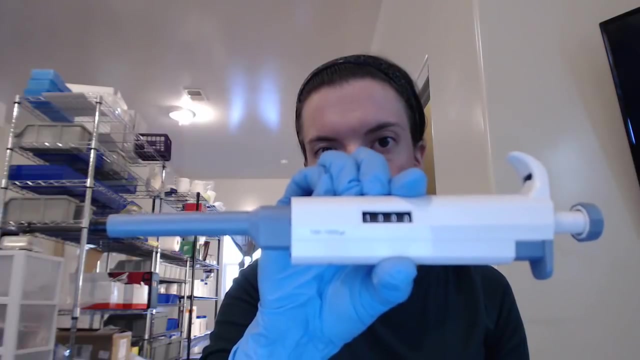 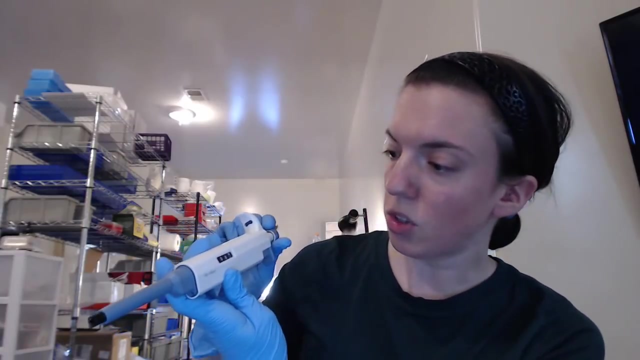 clean it off afterwards before you close it, to keep your scales in good shape, And so that's basically scales. Those are pretty easy. And then we have our pipettes. So you have, or are getting three different pipettes. I'm currently using the 100 to 1000 microliters, So you change. you still want to use your gloves always, and you 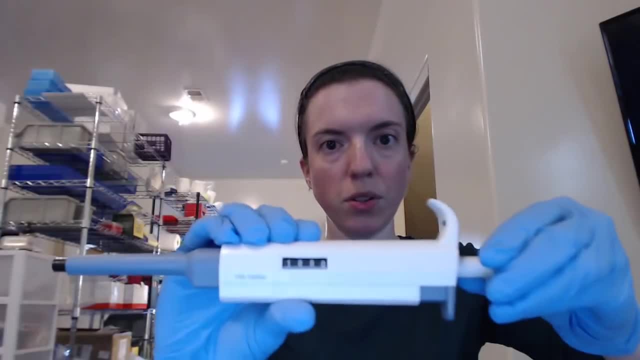 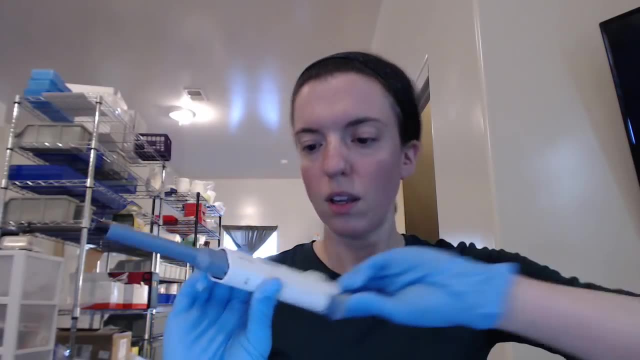 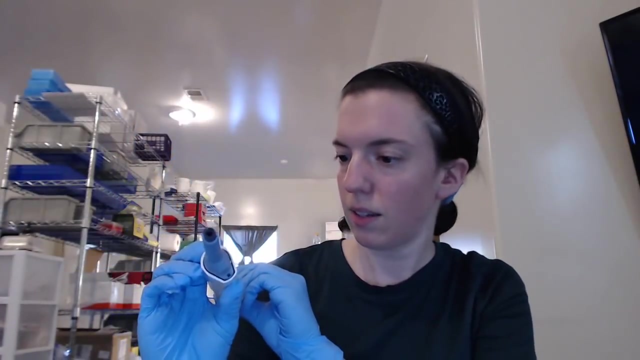 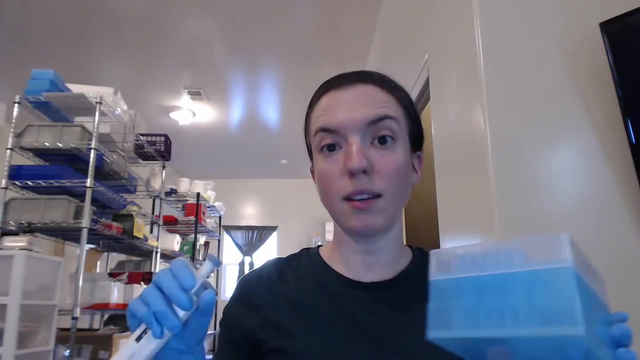 change how much the pipette holds by moving, rotating the end part. So if I want, for example, 900 on this one, I'll just go like that And it's at 900. And then you're going to put on your tips. So we sent you three different sizes of tips for your. 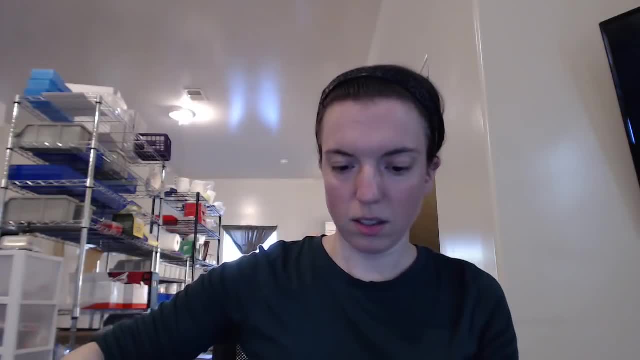 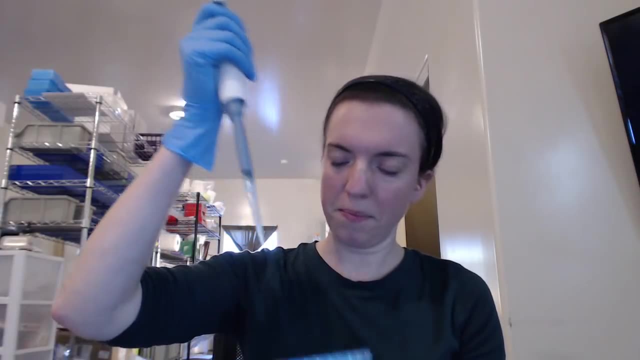 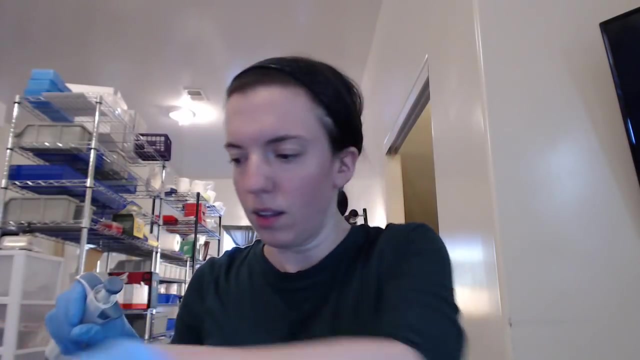 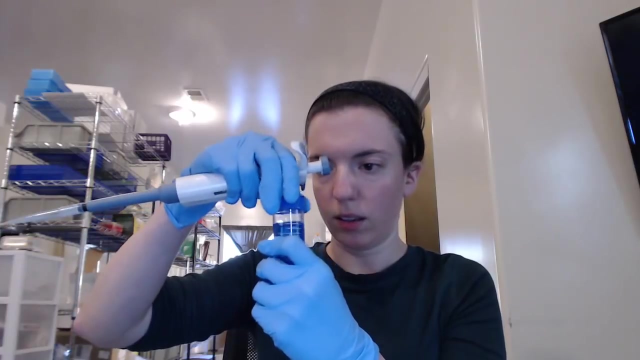 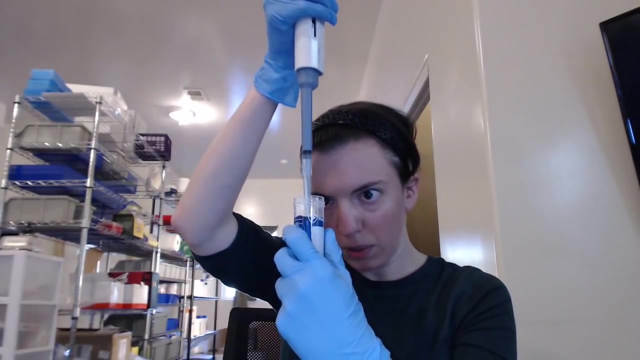 three different sizes of pipettes. So when you put it on you just make sure that it's on nice and firmly. Sometimes do a tap and bring it up. Then you're going to take your liquid that you are pipetting And you want to insert the tip far enough down so that you'll make sure that you won't suck up any. 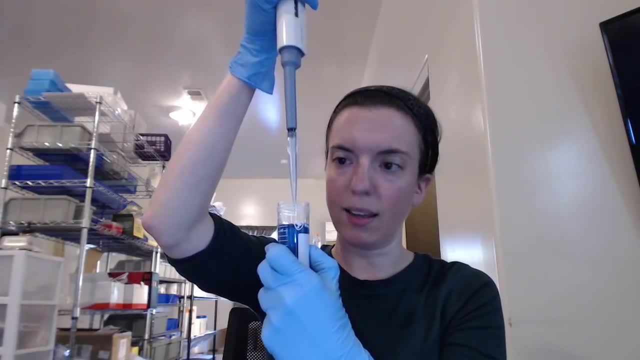 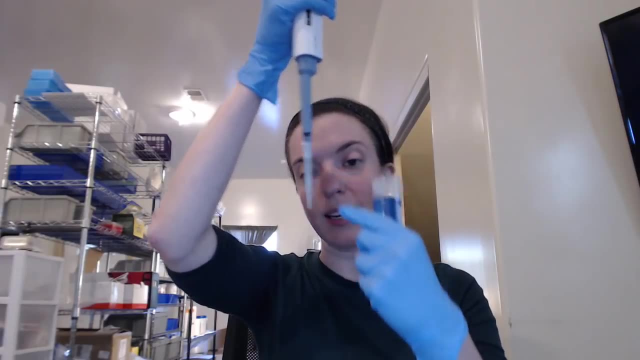 air bubbles. But you don't want to stick it in as like as far as it can go, because then you'll have a lot of liquid adhering to the outside and it could mess up your measurement. So you stick it in a good amount And first you do. 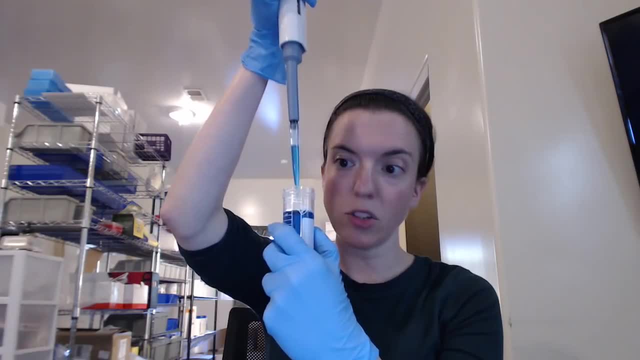 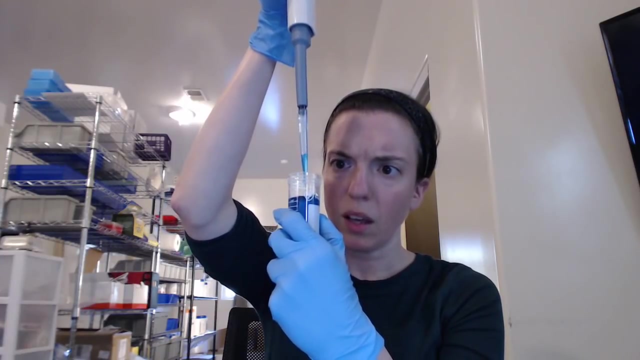 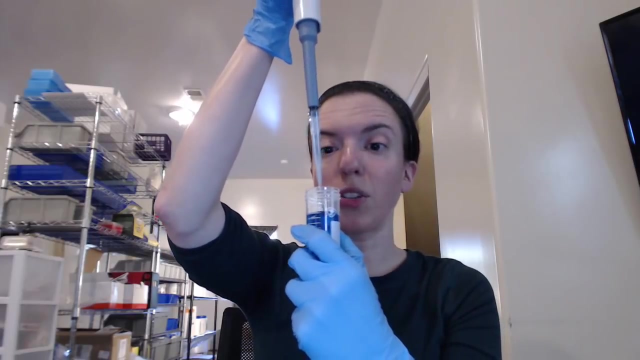 three times where you suck up the liquid and then just put it back, because that coats the inside of your pipette tip So that you don't lose any. You don't lose an amount of liquid the first time you're doing it. Um, also, right now I'm just using colored water, So it's coming up pretty quickly. However, when it's 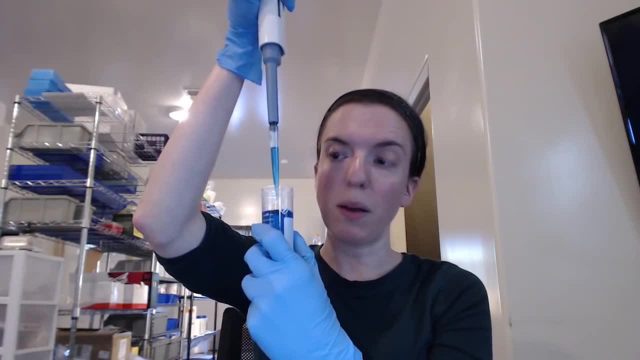 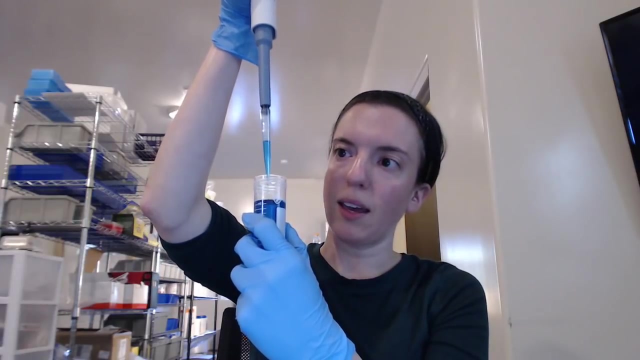 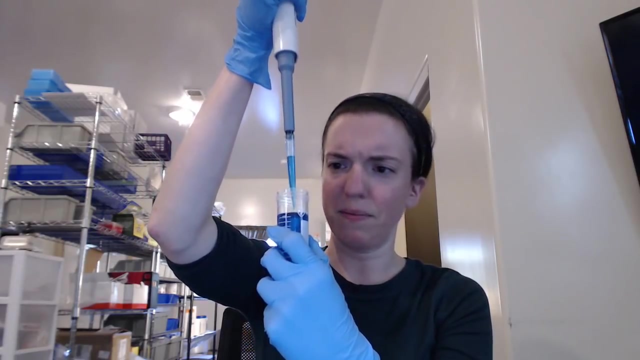 wet. you don't want to put a paper towel in it, You don't want to. if you're using, if you're pipetting something thicker, you might want to wait- and I generally like to count to a three if it's a thick liquid- to make sure that it's had enough time to to uptake all the liquid. and you want to uptake and put out nice and smoothly. You don't want to like flick it or anything that's gonna mess up your measurement. 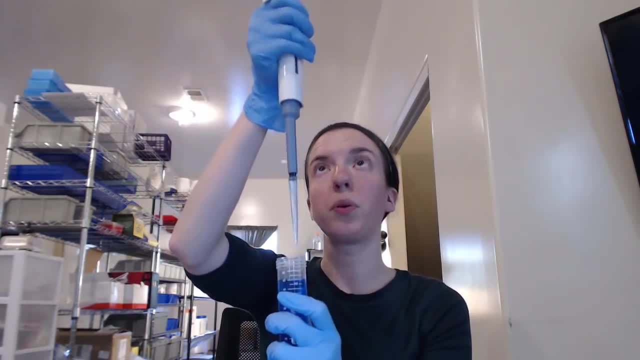 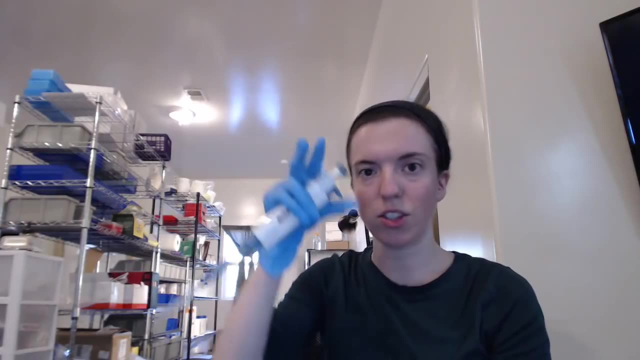 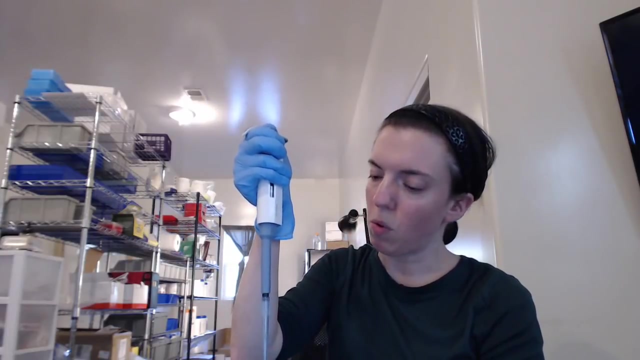 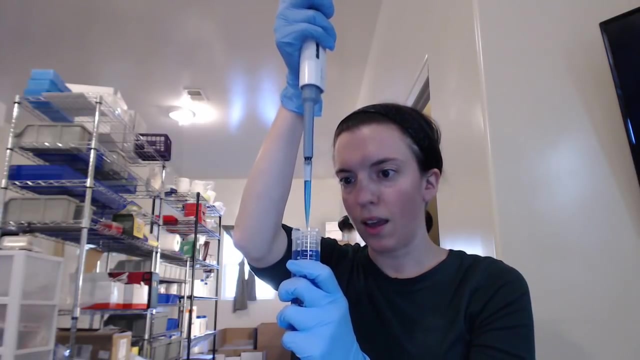 Um, So when you uptake, you go down, there's two stops on a pipette. There's what's called the soft stop, which is where you feel slight pressure, but then you can push it down more, And the reason for that is you go to the soft stop to pull up your liquid and then, when 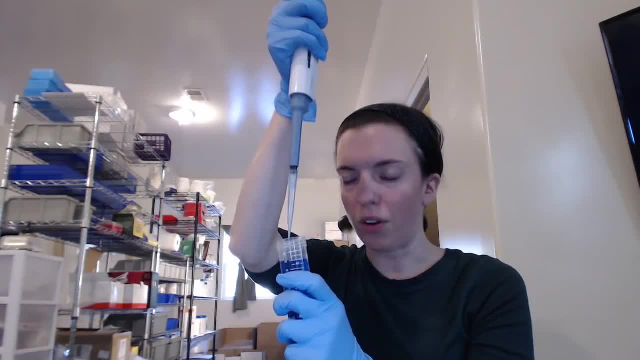 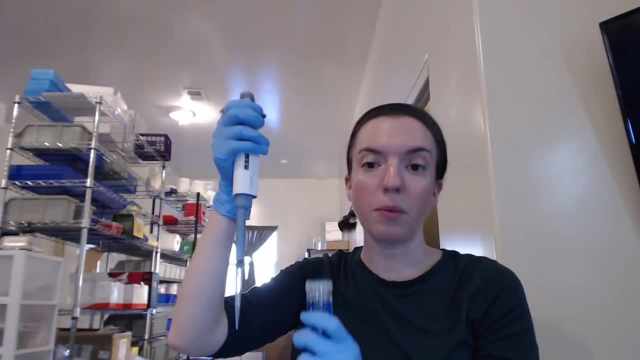 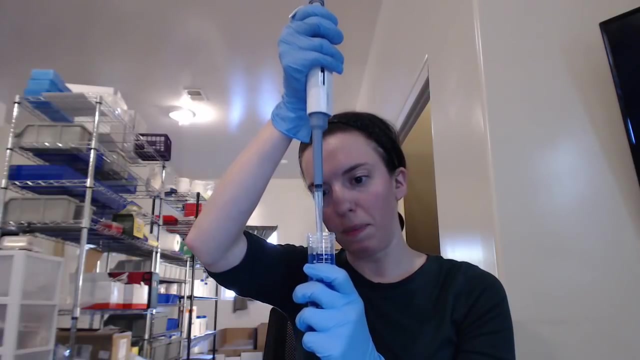 you go down to release your liquid. you go all the way to the full stop and then that makes sure that all the liquid that was in there is pushed out. It just pushes it out with some extra air. You want to have the pipette go in at 90 degrees when you're taking up. 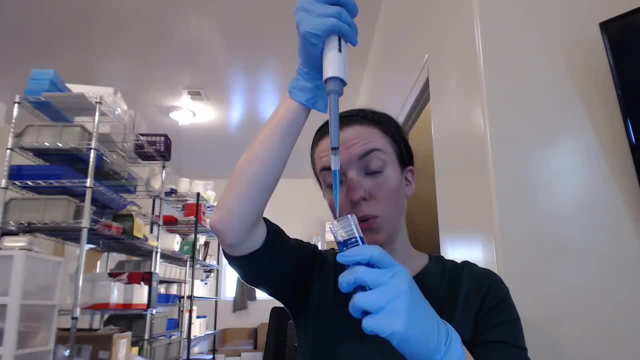 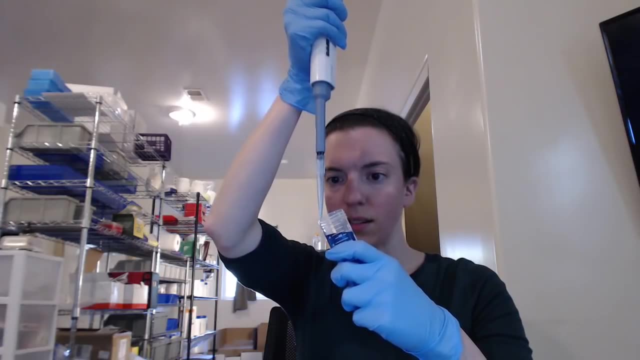 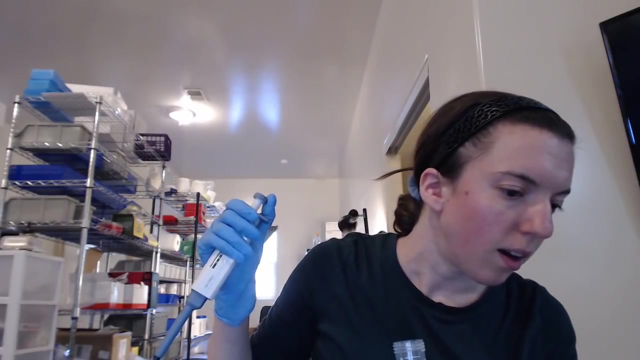 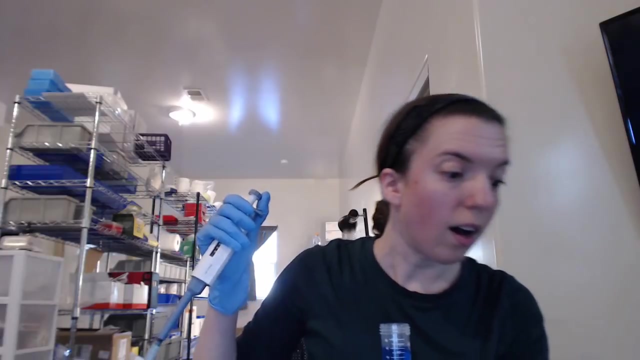 However, when you are putting it into another container, You want to slightly angle the container so that it doesn't splash and it goes in nice and evenly. Okay, let's see If your pipette is full. you do not want to lay it on its side, because then the liquid. 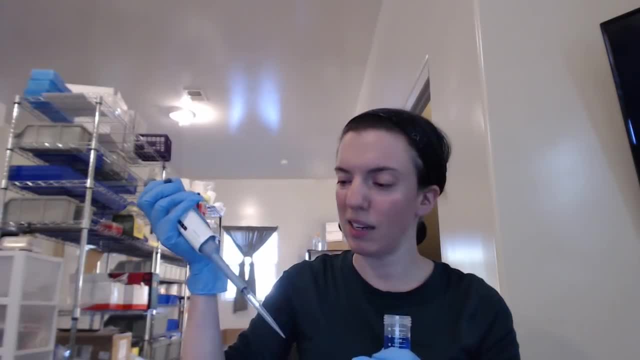 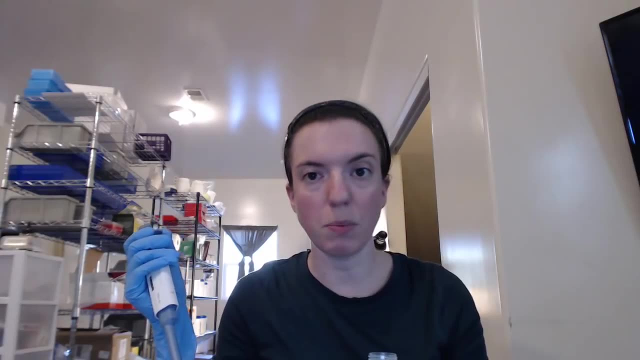 can get into the actual pipette and contaminate it and that would be a pain to clean. so you'd have to do that. You definitely don't want to do that. If your pipette does get dirty, you can clean it with 70 to 90 percent ethanol and that'll. 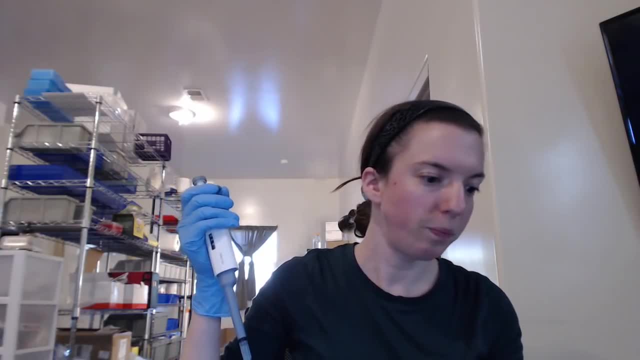 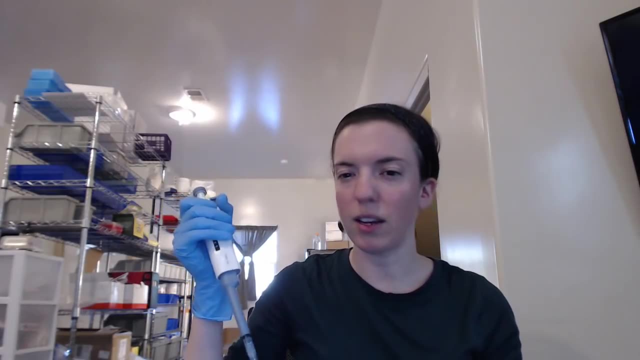 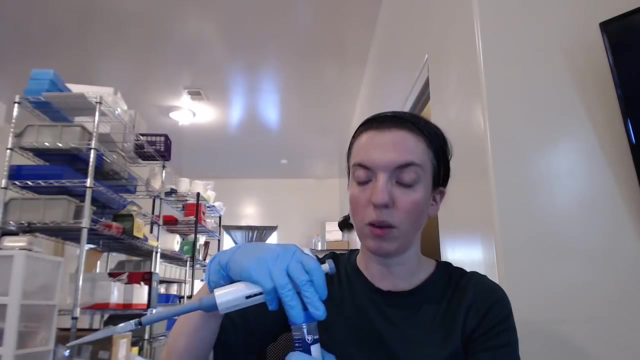 help sterilize it so that you can use it again without contamination Once a year. you want to calibrate your pipettes. I believe there's instructions in there on how to do it. Basically, you're using the density of water and you have a scale and you weigh out the